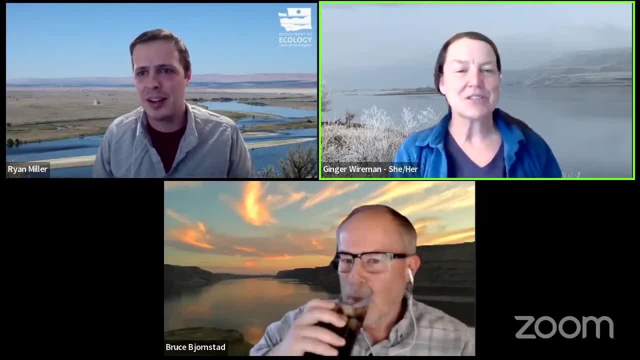 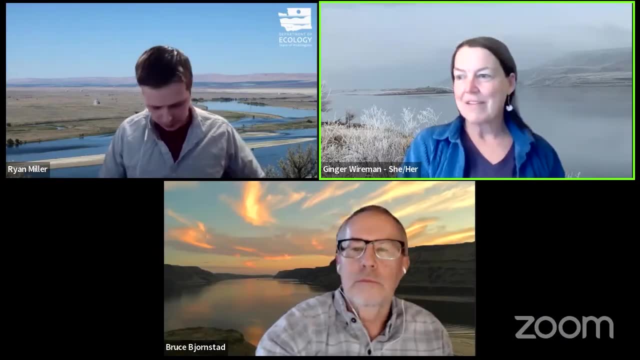 Well, welcome everyone and thank you so much for your patience. My name is Ginger Weierman and we're glad to have you here to participate in our Let's Talk About Hanford tonight themed Hanford: geology, floods, lava and more. 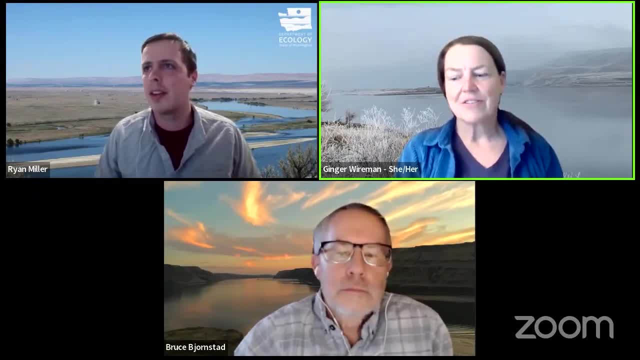 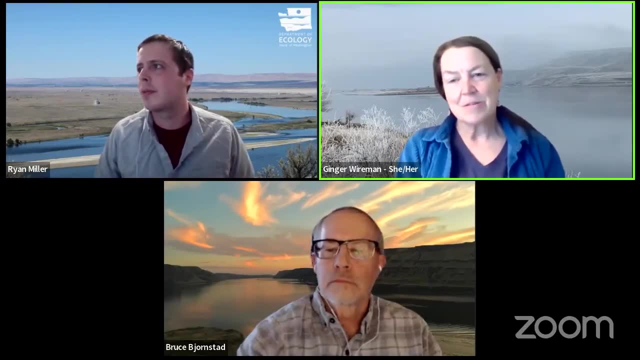 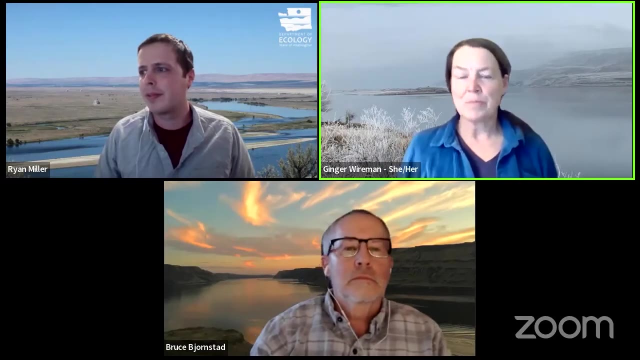 And gosh. this is our fifth or sixth episode of Let's Talk About Hanford, and we are using this to be able to reach audiences that we can't reach because we have been all stuck in our homes and not going out into public to do public speaking. 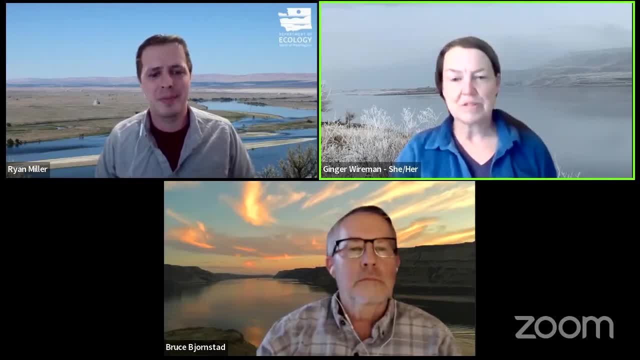 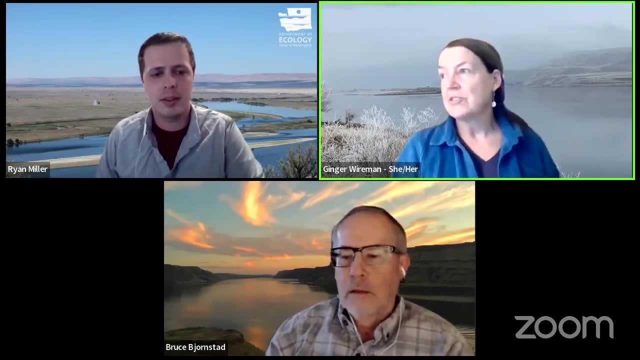 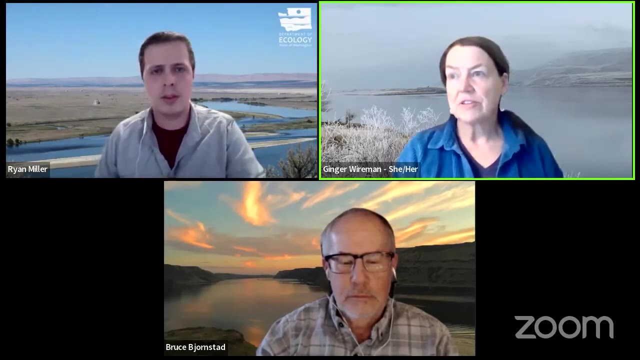 So this has been great and we are really excited to have Bruce Bjarnstad with us tonight. Bruce is a licensed geologist and hydrogeologist And retired senior researcher from Battelle's Pacific Northwest National Laboratory. He earned a bachelor's degree in geology from University of New Hampshire and a master's in geology from Eastern Washington University. 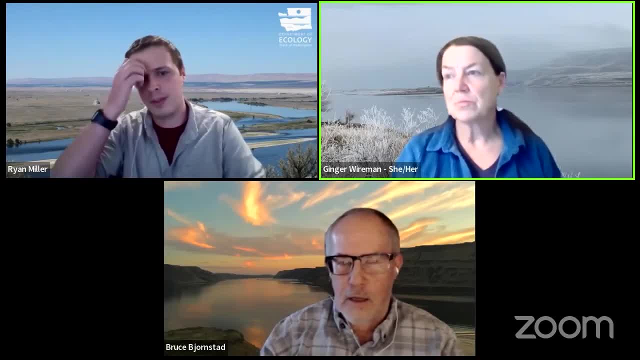 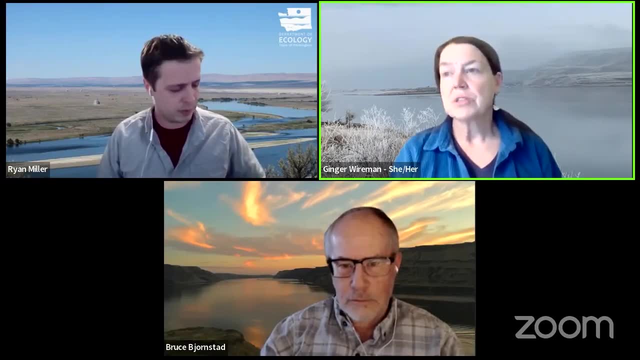 And during his 35-year career Bruce published numerous reports and documents on the geology of Eastern Washington and the Hanford site, in addition to numerous books on the local Ice Age megafloods. So we are excited to have Bruce here tonight. 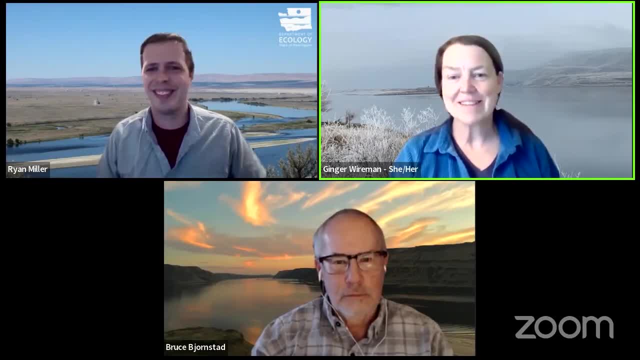 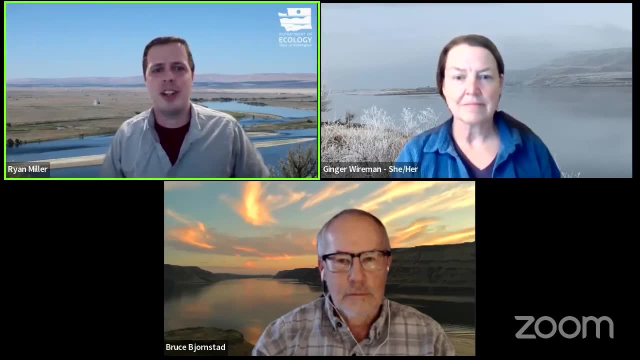 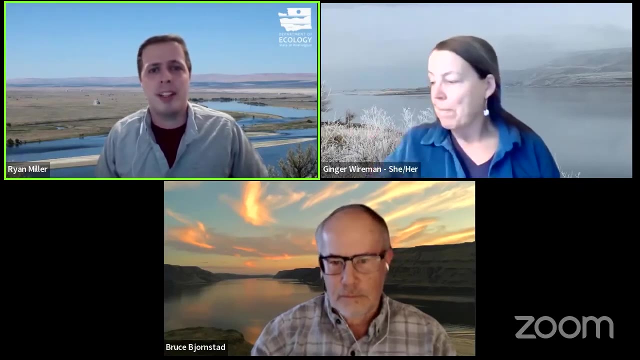 But real quick, Brian's going to go over some housekeeping and then we will get into the presentation. Perfect Thanks, Ginger. And thanks again everybody for your patience, as we got everything set up a few minutes late today. So, as per usual, with our Let's Talk About Hanford events, we're going to start the night with a presentation. This time will be Bruce covering Hanford geology. 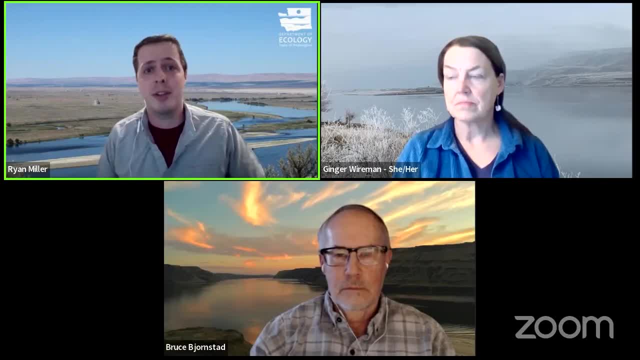 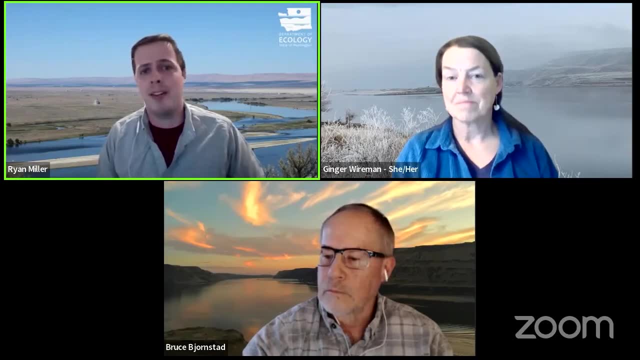 And after that we're going to move into a live Q&A with you, the audience. So anytime during tonight's event you can input any questions or comments you have into the chat if you're on Zoom or the chat if you're on Facebook. And since this is our first time on Zoom, 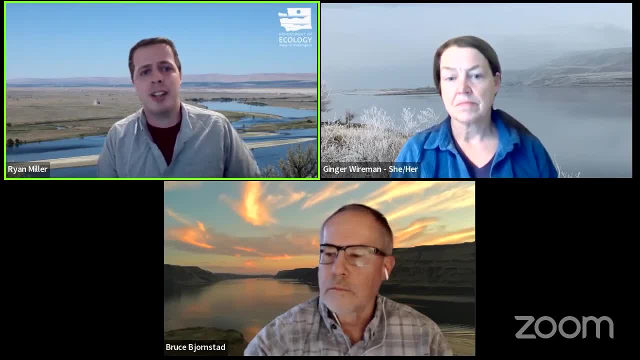 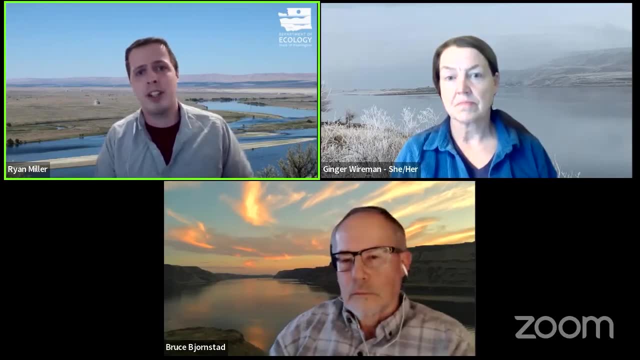 after Bruce's presentation, I'm going to change the feature so that those in attendance on the Zoom call can unmute themselves and turn on their cameras if they would like to, you know verbally- ask their own question to Bruce, or you could just put your question in the chat. either would be just fine. 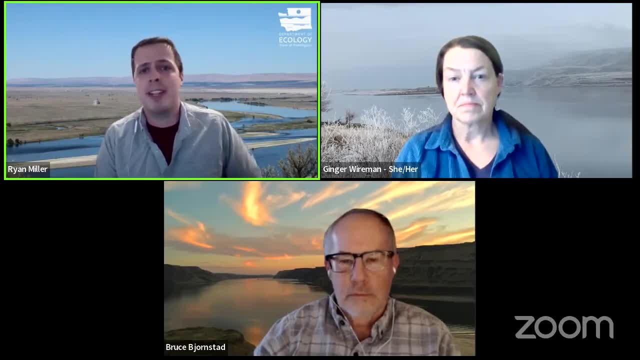 So definitely, as our event goes on. if you have any questions about tonight's presentation, feel free to put it into the chat, And it's just a reminder that we're going to be doing a lot of work on our website, So if you have any questions, feel free to put them in the chat. 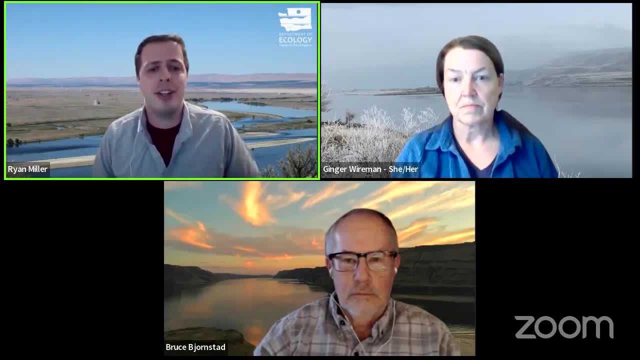 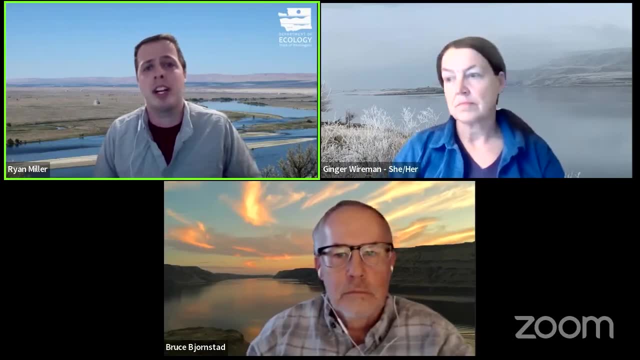 And it's just a reminder. these presentations are geared to be more high-level information and for those who are new to or getting to know about the Hanford area or those who only know parts of Hanford and would like a refresher. so we really try to keep these high-level so everybody can understand them pretty easily. 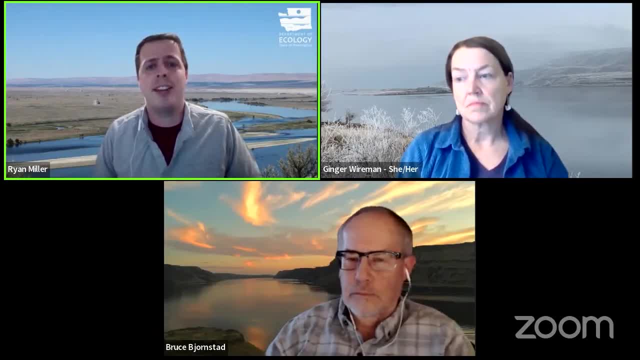 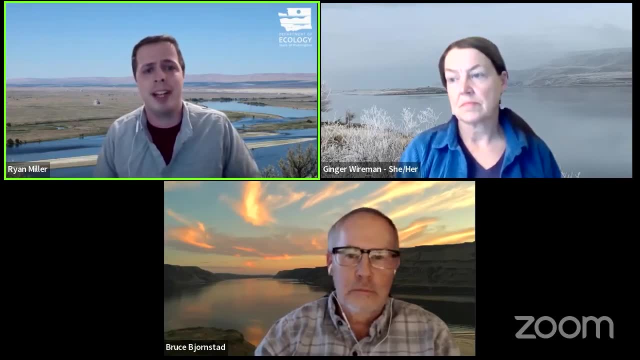 So, like I kind of mentioned before, we encourage questions and comments into the chat at any time, but we do ask that you please gear your questions to Hanford area geology, as that's Bruce's area of expertise and not Hanford site cleanup or other. 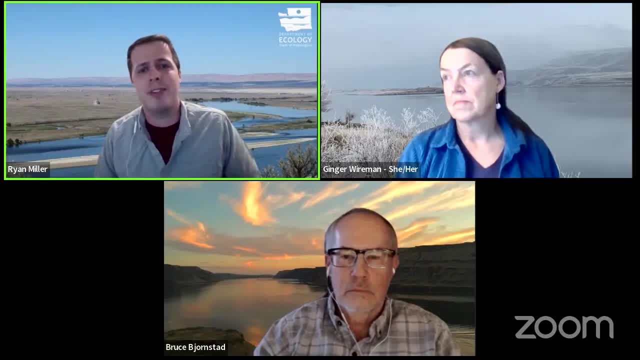 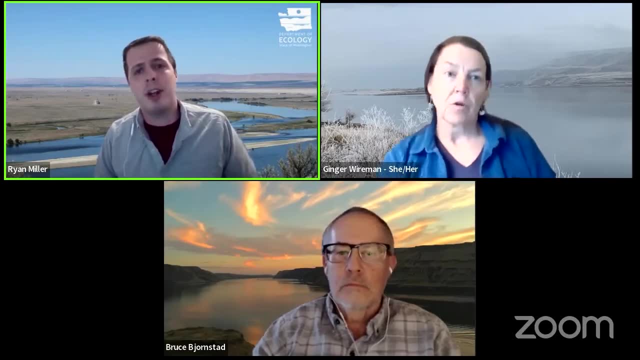 topics. We'll do our best to answer your questions questions, but if we get questions that are off topic, we'll probably have to defer your questions to a future event where we focus on that specific topic you're asking about. Alternatively, you can: 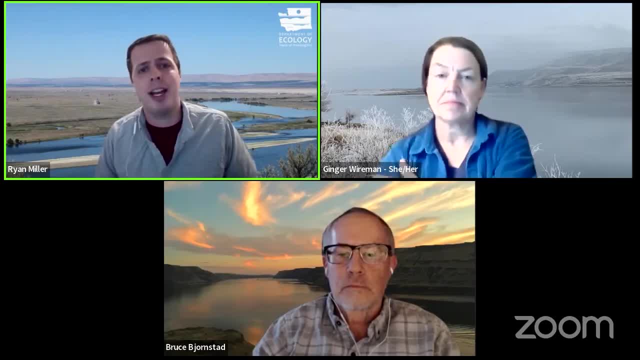 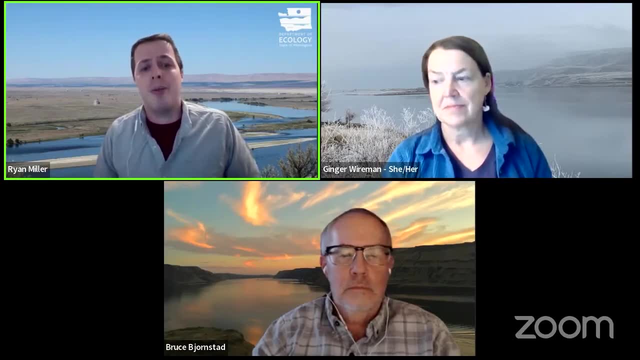 always send those questions to our email at hanford, at ecywagov. Again, that's hanford at ecywagov and I'll put this into the chat as well. But if you have any questions about Hanford, 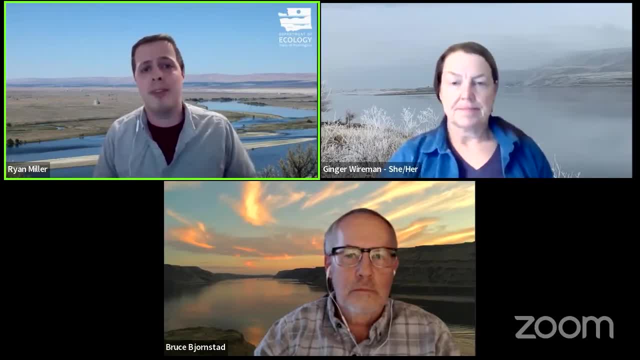 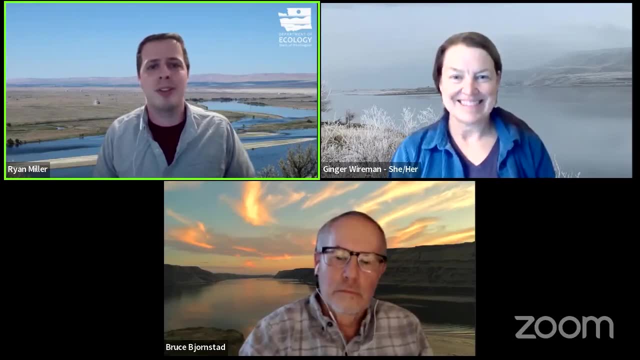 feel free to stick them into that email and we can answer those off-air as well. But with that let's go ahead and kick over to Bruce and he can start teaching us about Hanford's geology. Over to you, Bruce, Okay. well, thank you for that introduction. It's a pleasure to be talking to you guys. 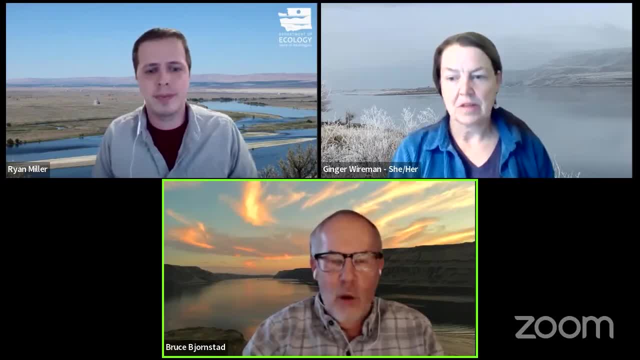 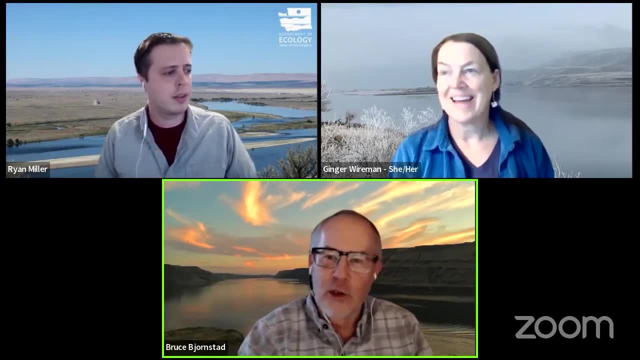 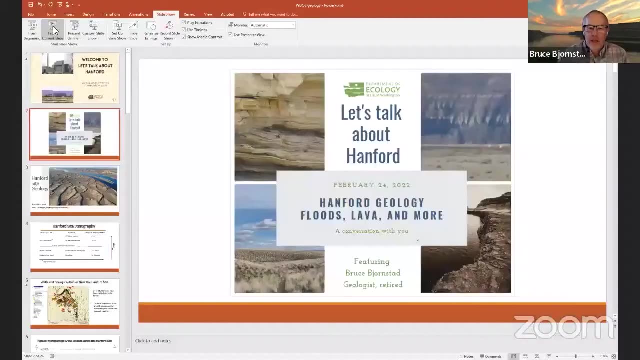 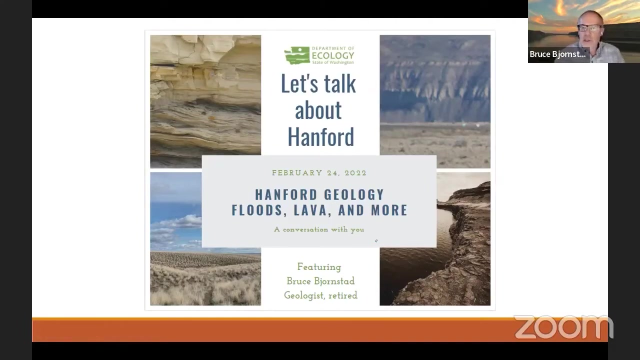 about Hanford. I've been away from the Hanford site working as a geologist for about eight years, but the geology really hasn't changed much during that time, So hopefully I can shed some light on the geology for everybody. So here's my cover of my presentation. 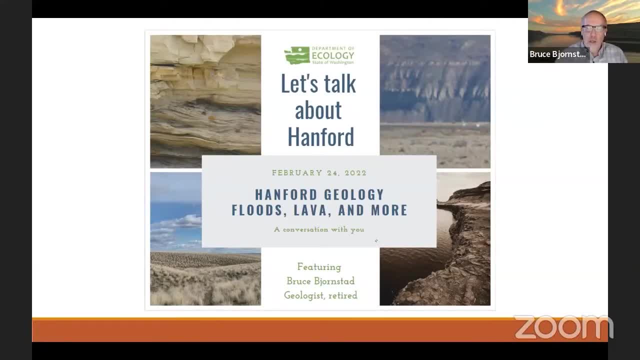 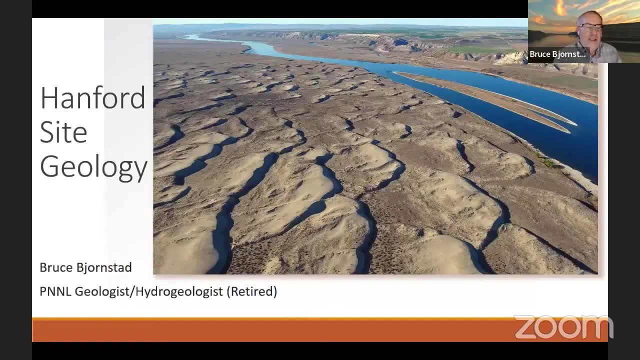 and I think Dana, who's there with you guys, is gonna bring my presentation to the screen. There we are, And this is a view looking across the Hanford site on Columbia River and the White Bluffs in the background. The geology of the Hanford is. 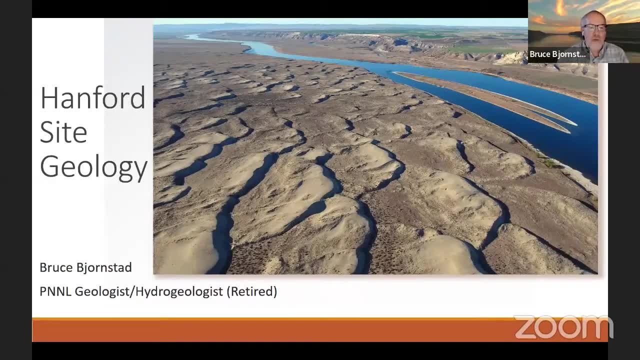 very diverse and it's fairly unique. It's got an assemblage of geologic features that are kind of unique to anywhere else in the world. So it is a unique geologic environment, and that's what my presentation is about today. So let's go on to the next slide. 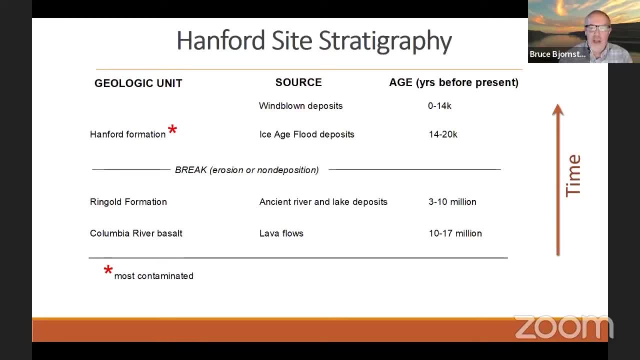 It's important first of all to set the stage for the geology, And the geology is really based on the stratigraphy, these deposits, the geologic evidence for past events on the Hanford site And that is revealed here in the stratigraphy, As you can see here that we have the Columbia. 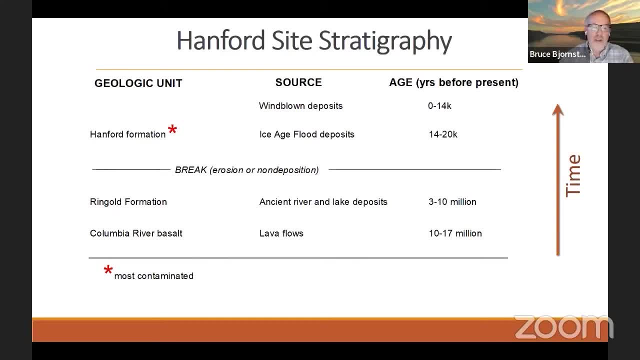 River Basalt down at the bottom. That's the oldest unit geologic unit. And then we have something called the Ringel Formation, which are sedimentary deposits over the Group Basalt. And then above that we have this big Ice Age Flood coming through the Pasco Basin and through the Hanford Site. 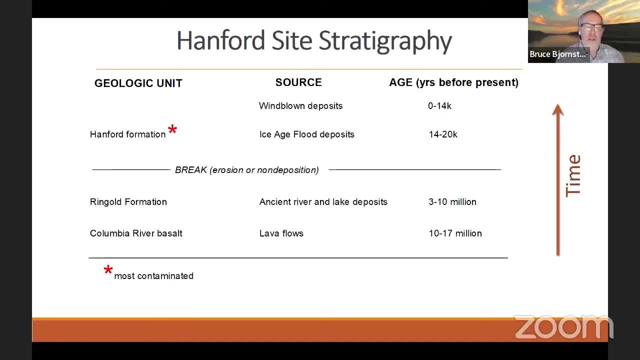 And it deposited up to 300 feet of flood deposits over the Ringel Formation and the Basalt. And lastly, we have the frosting on the cake, or a thin sequence of windblown deposits which have blown across and been deposited on the Hanford site since the last floods about 14,000 years ago. 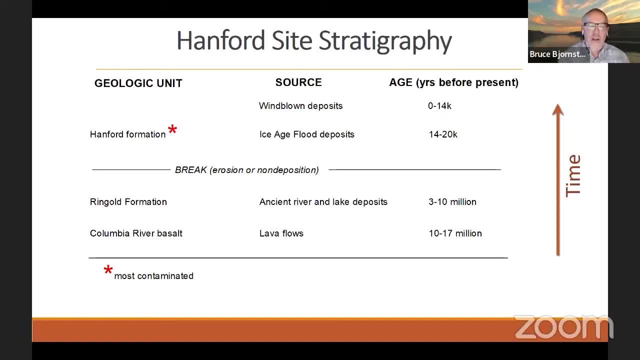 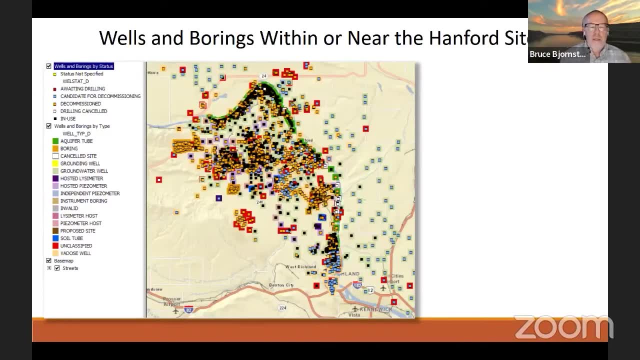 So this is the foundation. this photography is the foundation for the talk that I'll be presenting tonight. So next slide, Next slide: We know the subsurface geology at Hanford, based on wells and boreholes that have been drilled on the site and around the site. 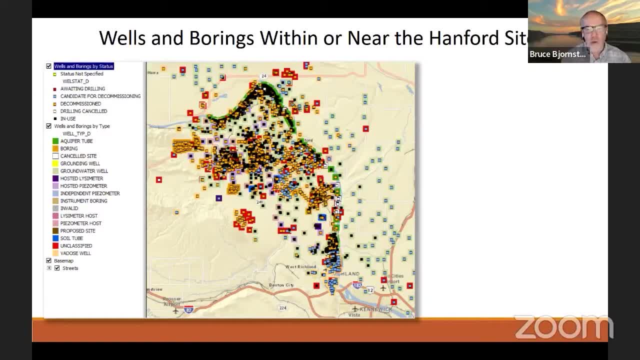 And here you can see the, you can see the where the Columbia River comes through. the Hanford site is basically that really dense cluster of wells that you can see off on the left side of the and lower left side of this, this diagram, And let's 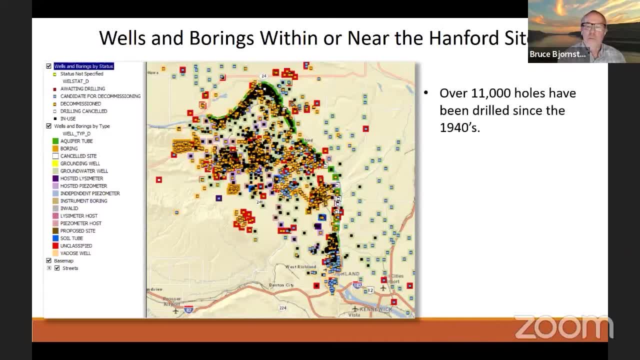 Well, we'll click Next, Go next And, as you can see here we have over 11,000 holes have been drilled on the Hanford site since the 1940s And next, But only about 4,000 of those are still being used. They're still available for use. A lot of the wells have been decommissioned and are no longer in use, So we actually have about 4,000 wells, But with those with that number of wells, 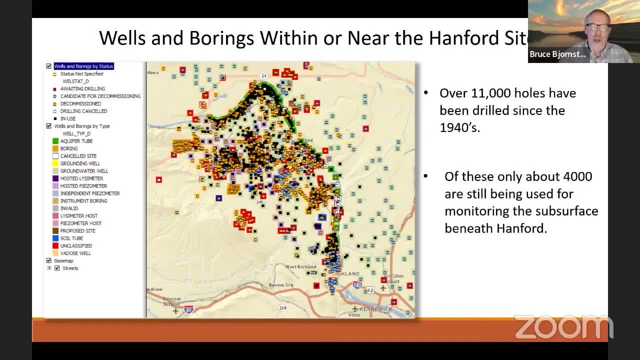 you can get a fairly good detail on the subsurface geology of Hanford And the reason for knowing that is because of the you know contamination and the waste sites that are on Hanford site. So you really need a lot of wells to really understand what's going on in the subsurface and how these contaminants move over time. Next, 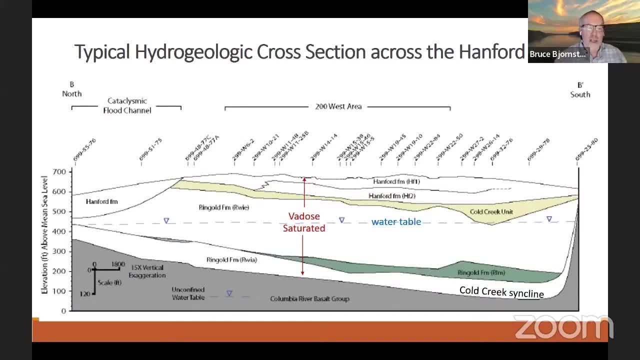 Here's a geologic cross section, Okay, going from north to south, And it's it's showing you these different units that have laid out. the Columbia River salt is that gray area down in the bottom That's. that's down hundreds of feet below the Hanford site. 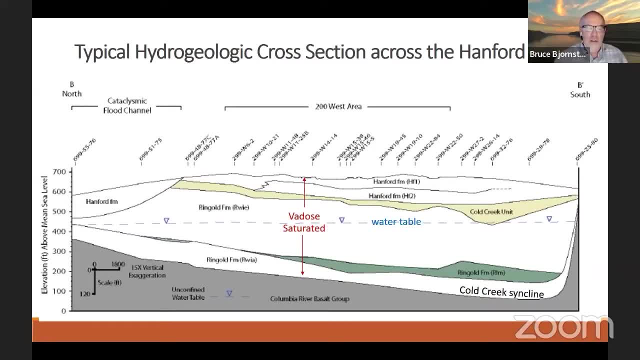 And I could be talking about all these individually in the coming slides. And we have a thing called the Coal Creek Sink Line, which is a basin that was formed due to the due to Yakima, the Yakima Falls tectonic depletion. 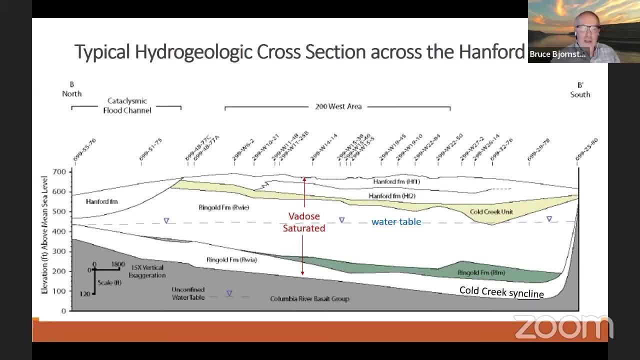 And it's this basin that is actually a base for the Hanford site, which is found up here, up at the right-hand side of the retreat. So this is the base of the Reformation Folding the basalt is created, this basin beneath the Hanford site, And above the basalt you can see there's a thing called a wrinkled formation. 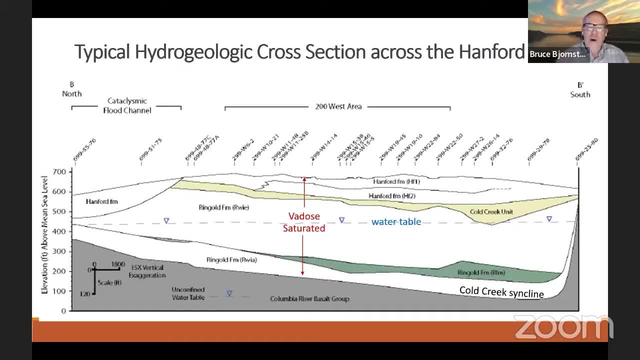 And that goes up to Coal Creek unit, which I'm not going to really talk about much today. It's fairly thin and it's not continuous everywhere. I'm not going to talk about that so much. but formation is both within the saturated zone in Methanford. 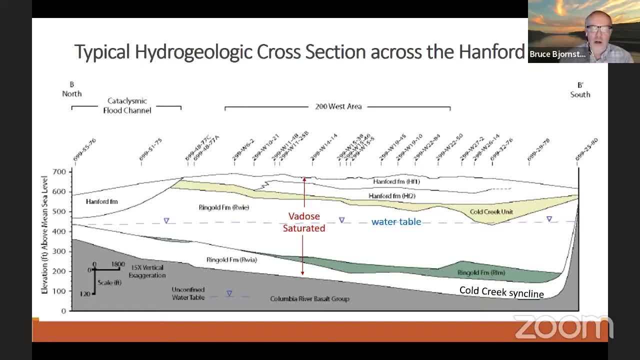 which is the area where there's water. groundwater is filling all the pores in the sediment. And then we have the Vado zone, which is above that. That's the area above the water table where the sediments are unsaturated. In other words, there's not much water present. 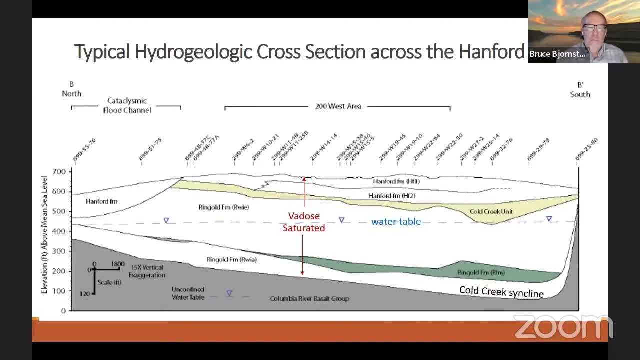 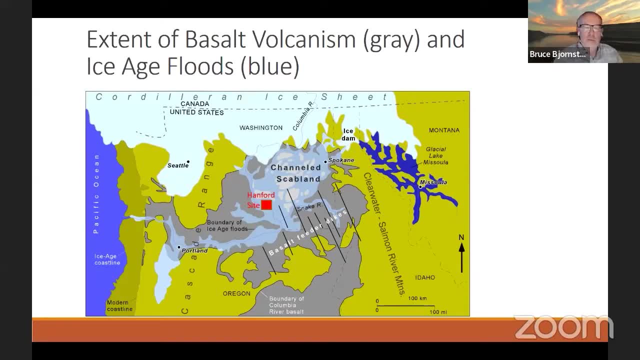 in that Vado zone. And so let's go to the next slide, And here you can see the distribution of the basalt- Columbia River basalt, which is in gray on this map And in contrast to where the Ice Age floods came through. 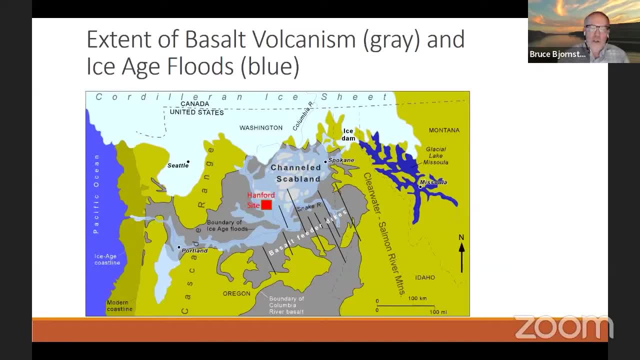 which is the area in blue So that you can see the Hanford site, experienced both the floods from volcanic lava flows as well as floods from Glacial Lake, Missoula, Okay next, And that circle, the oval, is indicating where we have the basalt coming out of basalt feeder dikes. 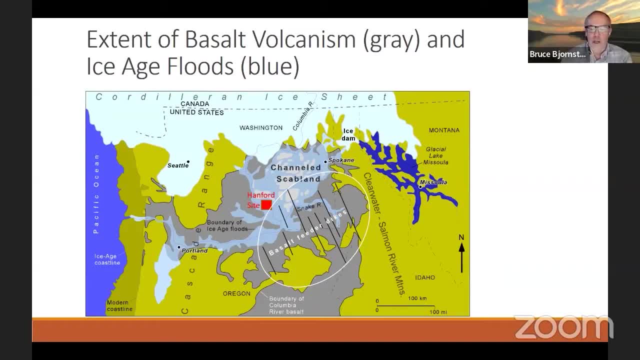 down in the Southeast part of Washington, Northeast part of Oregon, Western part of Idaho was the source for all the lava, is all lava that came out And these are feeder dikes of the Columbia river, basalt And basically, when the lava came out, 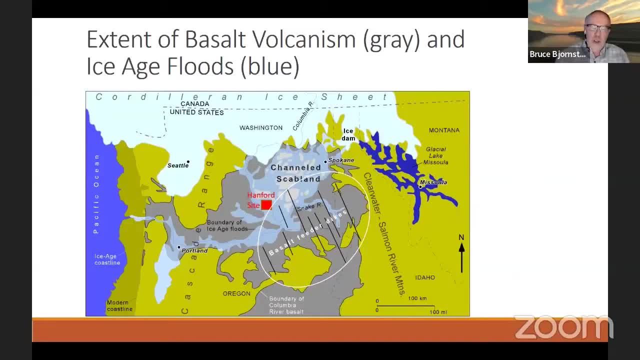 it's downstream but under gravity coming to the surface, And most of that gravity and area downstream was to the West. So basically the basalts were flowing out onto the channel scabb Кто, ůland of Washington, and then down the Columbia River gorge. 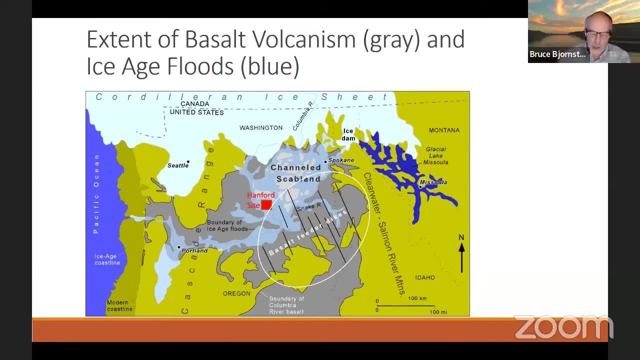 And then eventually you've got the eventually out as far as the Pacific Ocean Next. So there are up to 300 separate lava flows: Columbia River salt lava flows that came out between about 17 million years ago and the last ones coming out. 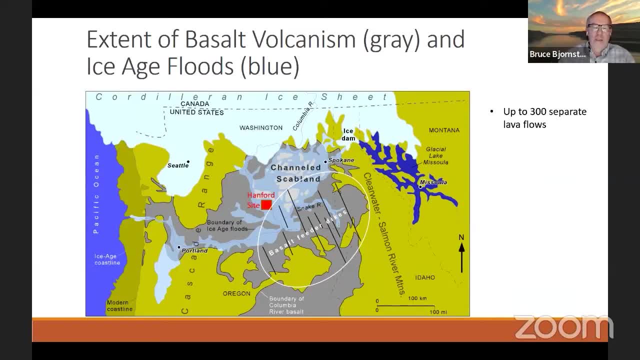 about eight to 10 million years ago, Coming out of these dikes and then spreading out across Eastern Washington. The combined thickness, the maximum thickness for those lava flows, is about 15,000 feet, And that is down in the Prosser area. 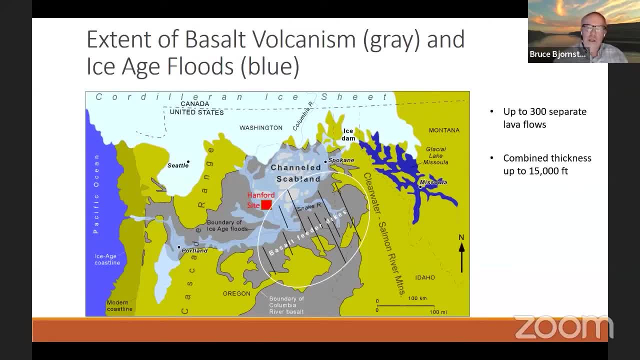 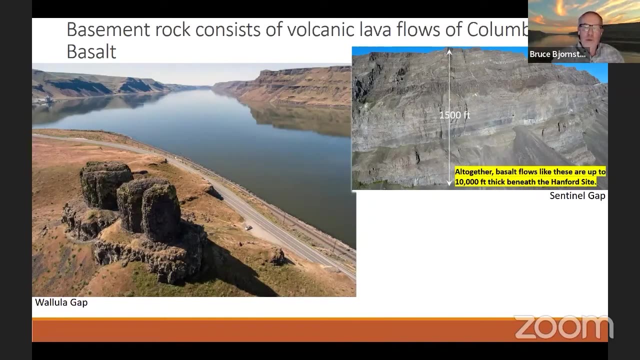 to the west, south and west of the Hanford site is the actual the depot center, where the center of the Columbia River salt and the thickest accumulation- Okay, next, The Columbia River salts reached, about 10 million years ago, 10,000 feet thick underneath the Hanford site. 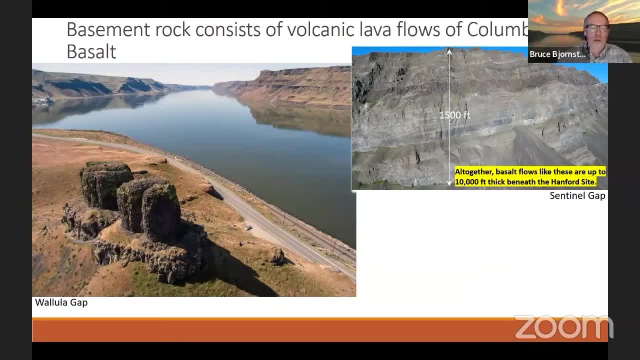 And here you can see where the lava flows are outcrop at the surface, at two wind water gaps, One called the Bullen Gap, which is on the left, And then there's another place called Sentinel Gap on the right, where you can actually see these lava flows. 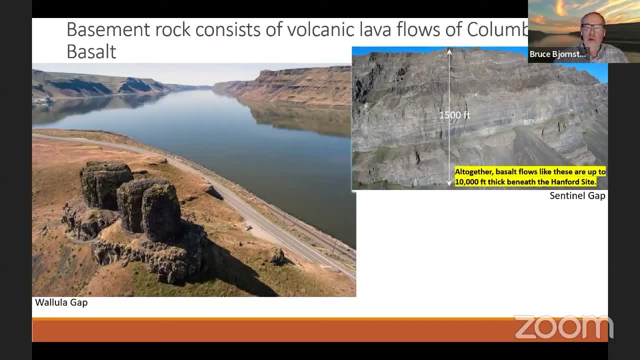 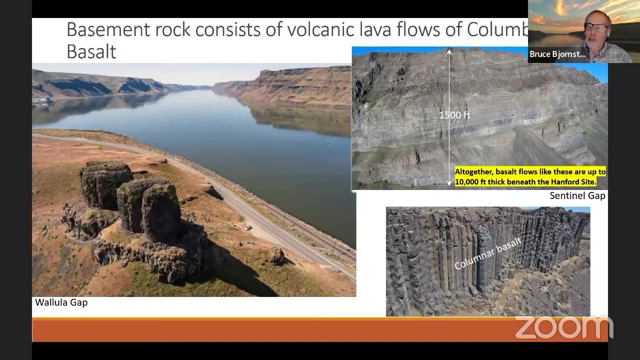 where they come to the surface, But these same lava flows are going to go underground another 10,000 feet or more beneath the Hanford site. Okay, next And these lava flows. there's quite a bit of heterogeneity, a lot of variation within these lava flows. 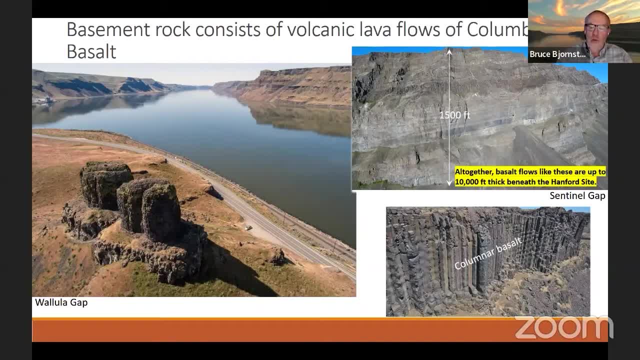 But most lava flows show a zone of what we call columnar basalt, where the lava was insulated and cooling very slowly after it came out. And then there's another zone called the Basicular's zone, which is a more hackley, more random. 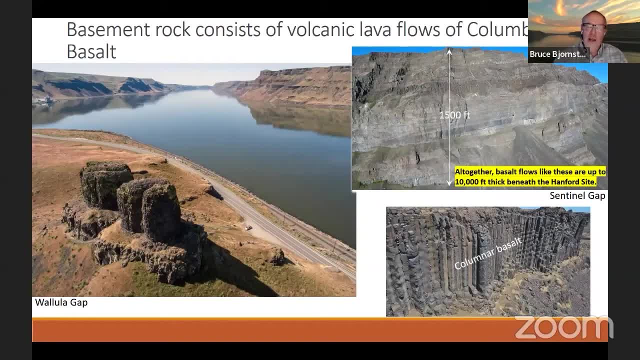 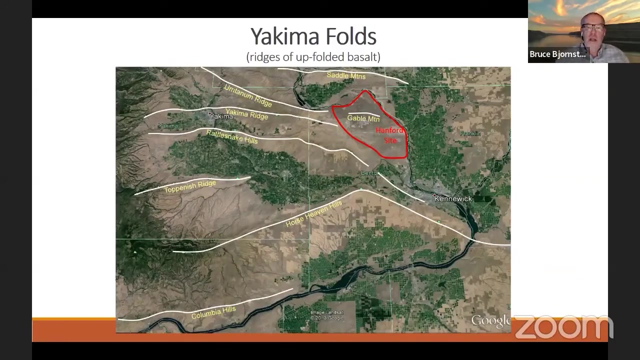 tightly a fractured rock above the columnar basalt. So those are the two major zones of these lava flows And they do affect the way water- groundwater- moves through these lava flows Next. So here's the Hanford site in red and what I'm showing here. 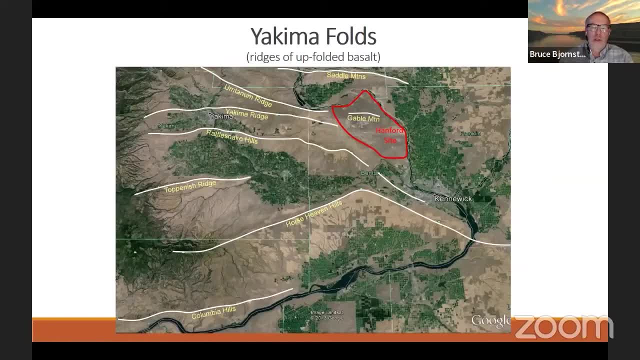 showing on this map are the Yakima folds, starting with the Columbia Hills down south and ending with the Saddle Mountains, And there's another fold called the Frenchman Hills, which are north of the Saddle Mountains and it's not shown on this map. 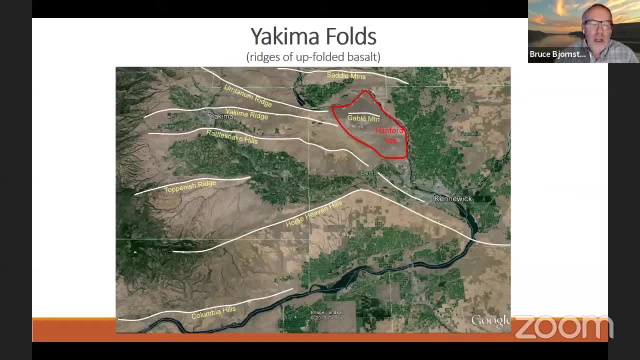 These are the Yakima folds and these are places where the salt flows have been folded, have been deformed by squeezing of the crust, And you can see, within the Hanford site we have the Gable Mountain and the climb, the Rattlesnake Mountain and the climb. 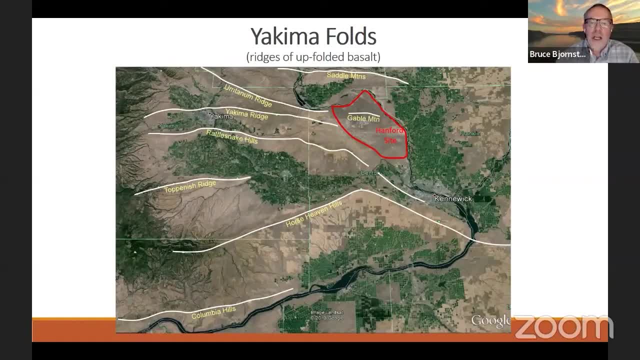 which is to the south, the Yakima Ridge to the west, Saddle Mountains to the north, surrounding us Next, And here's the locations of the Lilliput Gap and Sentinel Gap that I showed in the previous slide, showing you where these basalt flows are cropping out: 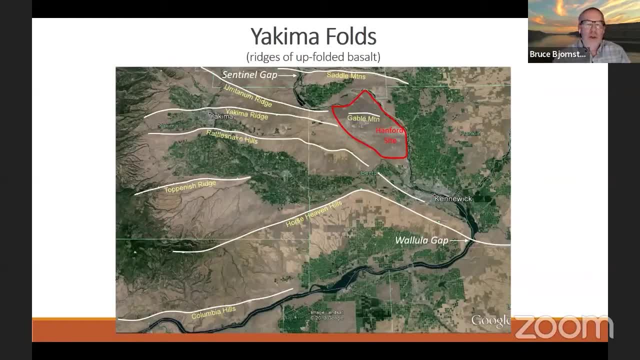 onto the surface And you can see that they have been exposed so that we can see them. but those same flows extend underneath the Hanford site and in the valleys where the sink lines in between these Yakima folds, So the folds themselves, are anti-clines. 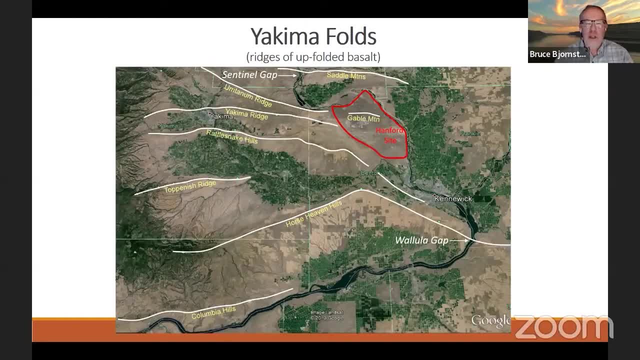 which are up-folded basalts, And then in between these ridges we have valleys or sink lines which tended to accumulate sediments since they were formed, Starting about 10 to 12 million years ago Next. So here's kind of a cross section. 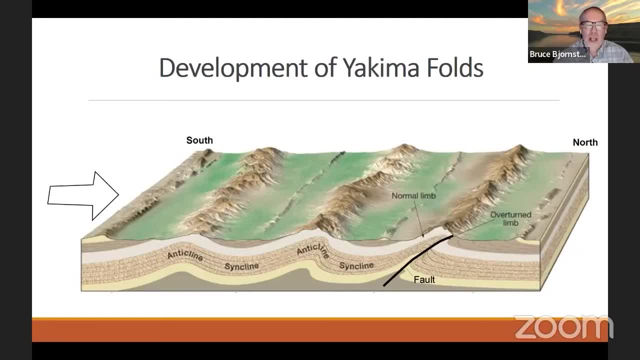 showing you how these Yakima folds develop. When the lavas came out, they came out as flat, pancake-like lava flows that spread out for dozens to hundreds of miles in many different directions. And then, after the lava flows hardened, the earth's crust was getting squeezed. 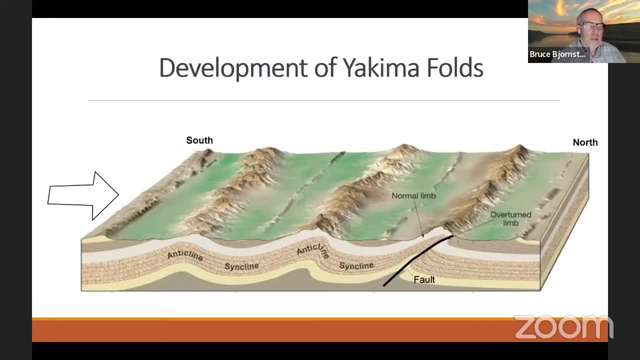 from the north and from the south And so that we get these ridges or wrinkles in that basalt surface. So here you can see, the up-folded areas of basalt are called anti-clines and the down-folded areas are sink lines. 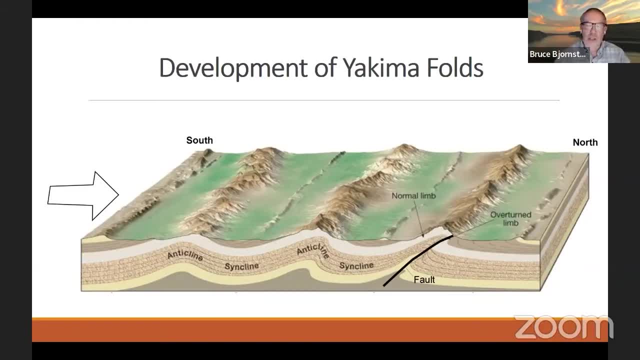 that have accumulated sediments, sedimentary deposits, since the lava came out, And occasionally those folds can be folded so drastically and so forcefully they can generate faults. You can see there's one overturned limb of a fault along the fault line in the right hand side in this image. 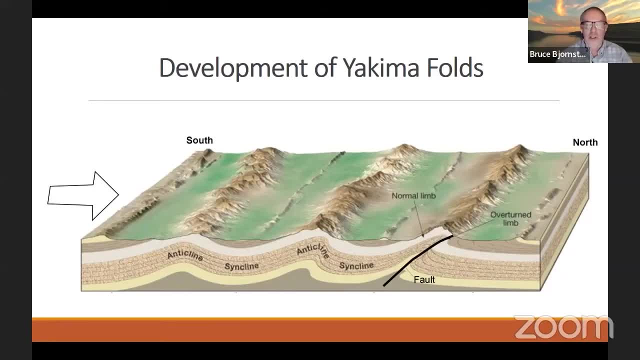 not all of the folds have these faults than many do, and there are always being. They're overturned to the north, So that's an indication that this is. you know that the force that was creating these folds was being directed from the south the area to the. 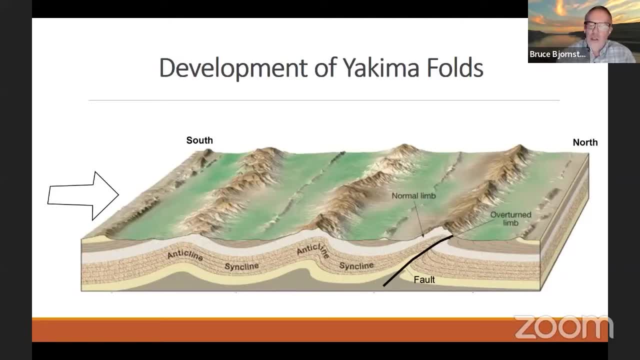 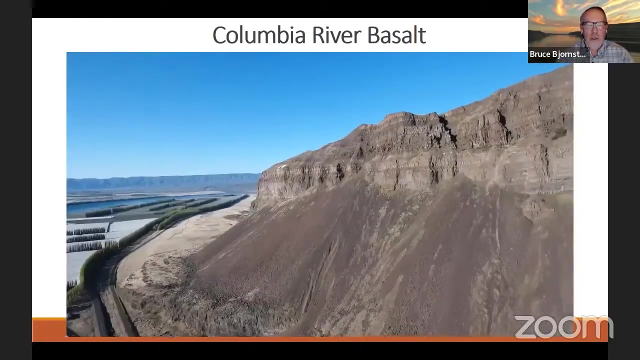 north was more rigid and uh was a was wasn't really moving much, but the area to the south was getting moved and pushed to the north. that created these uh anticlines and synclines and uh faults that you can see here next. all right, so, uh, now we're going to try to. here we go. we have a video showing the basalts in a. 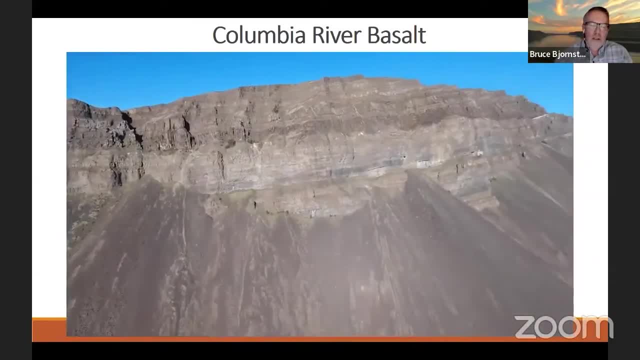 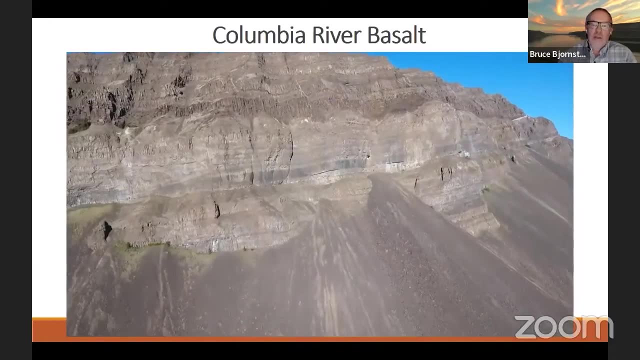 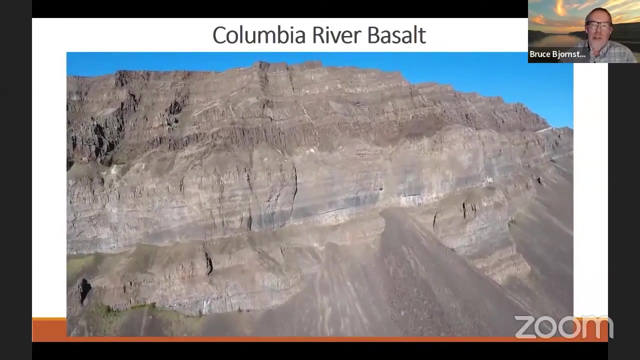 place called the sentinel gap, which is where the uh, the columbia river, cuts through the saddle mountains. so this is an anticline and these are basalts that uh were taken with the drone. you can see there's dozens of lava flows represented here in this exposure. 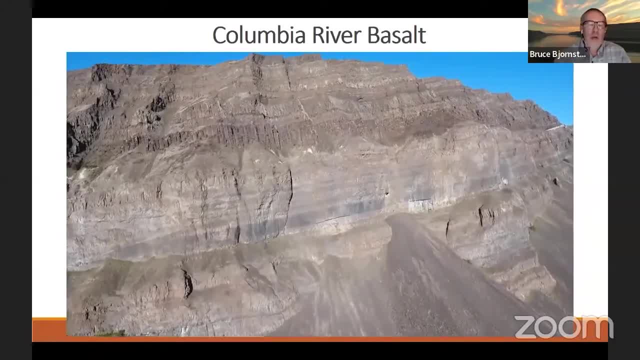 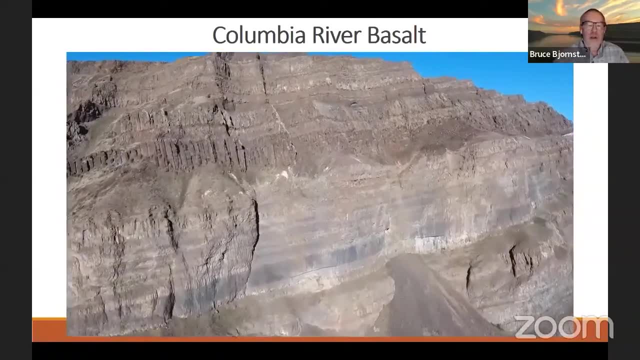 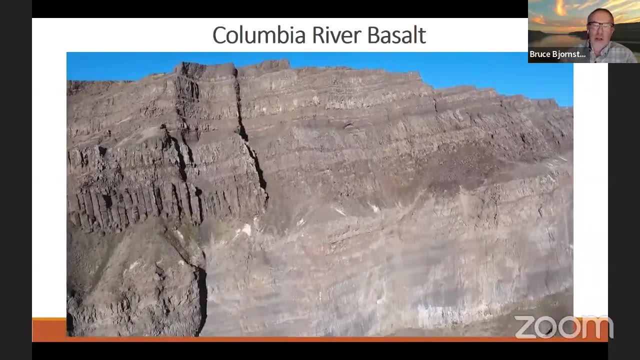 here and you can see some areas where there's a columnar basalt separated by areas with this more tightly fractured uh entablature assault and there is a white band that runs through through the middle of this. that's actually a sedimentary inner bed called the vantage inner. 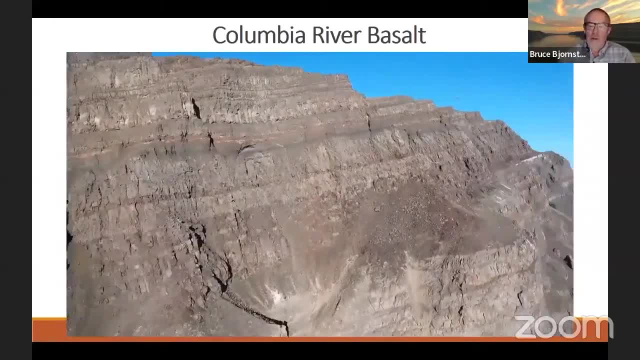 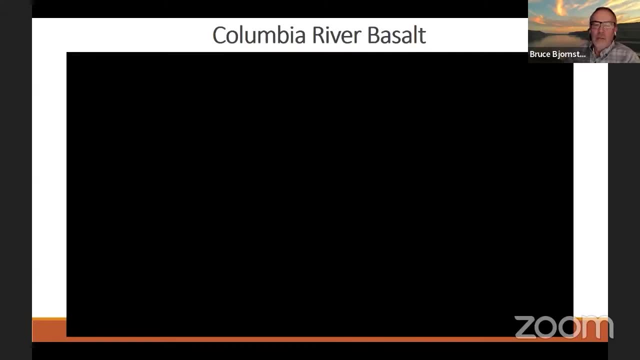 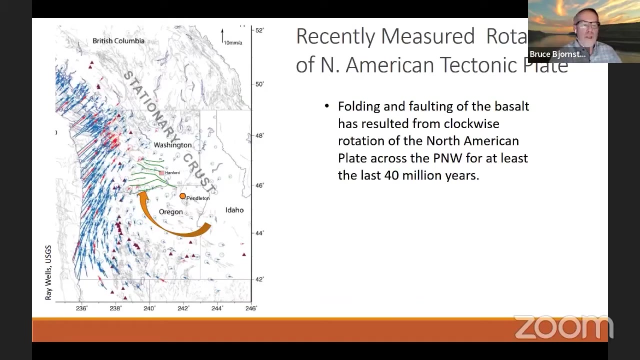 bed that was laid down between basalt flows. so these basalt flows were coming out between about 10 to 17 million years ago and when i showed you pictures of the yakima folds and where they're located, you can see in this image the green lines are these yakima folds and the reason that they're there and kind of 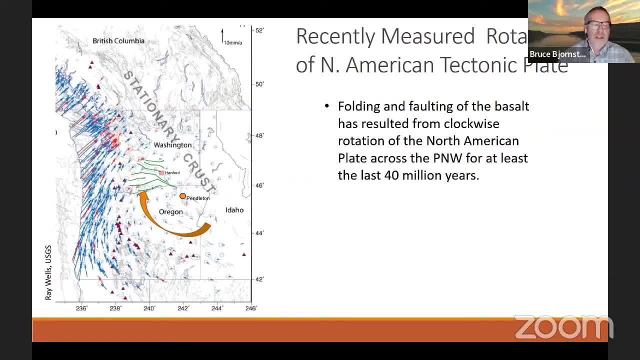 restricted to this area is because this whole area is being tectonically rotated in a clockwise direction and that that this is all related plate tectonics, uh related to the subduction zone, where where the pacific plate, the farallian plate, so the on the west side, uh in the ocean. 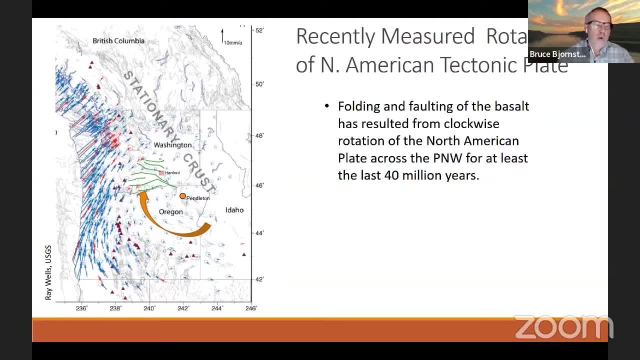 west of washington and oregon were being subducted obliquely to the northeast and that the pushing of those tectonic plates down into the subduction zone has caused the crust to rotate in a clockwise direction and the blue arrows and the red areas you can see here. 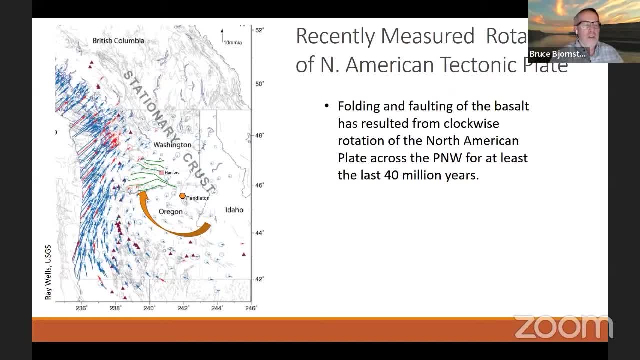 are relative distances, that the plate, the- uh, the north american plate- has been rotated over the last 40 million years. it's continuing today. these are actually real, real life. this is real-time data that was collected for one year, or or maybe the last year, and this is the average of several years, showing you how much tectonic rotation has occurred. 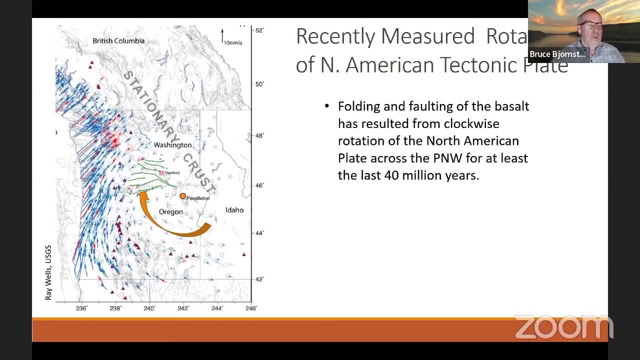 and they measure these, these distances, using gps units that are spread out across the northwest. so these are real-time data collected in the last couple dozen years, showing you the amount of tectonic rotation that's occurred, and over on the west side of the state, there's been up to 10. 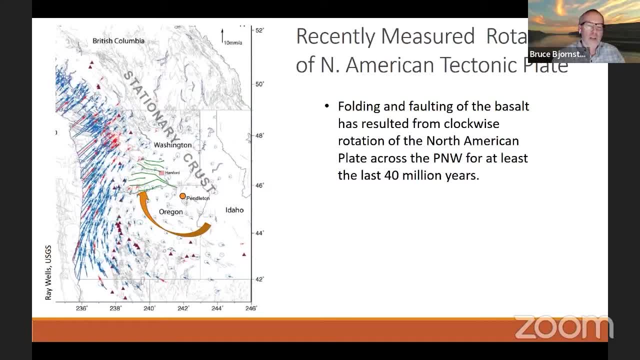 10 to 20 millimeters per year of tectonic rotation. next and uh that that 10 to 22 millimeters per year is about how long or how much distance your fingernails grow in one year. so the rate of tectonic deformation is relatively slow. but 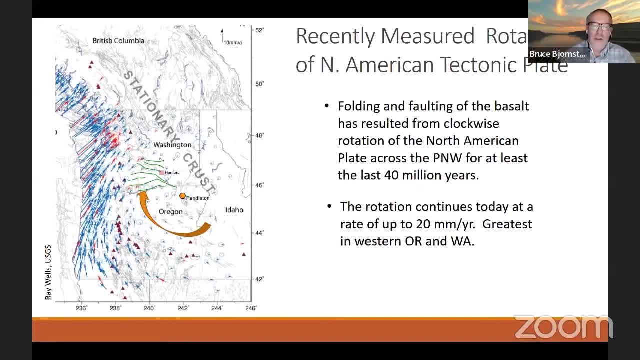 spread out over millions, 20 to 30 million years. you can easily get lots of tectonic rotation taking place, and it's these, this rotation. it's moving against the stationary crust north of the hanford site. it is causing these ridges to form in the basalt. next, and the pivot point for that rotation is right in our 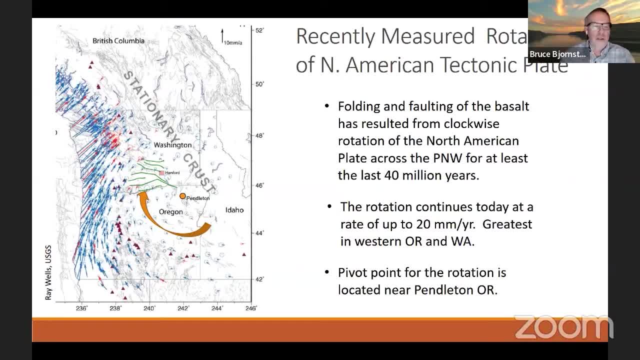 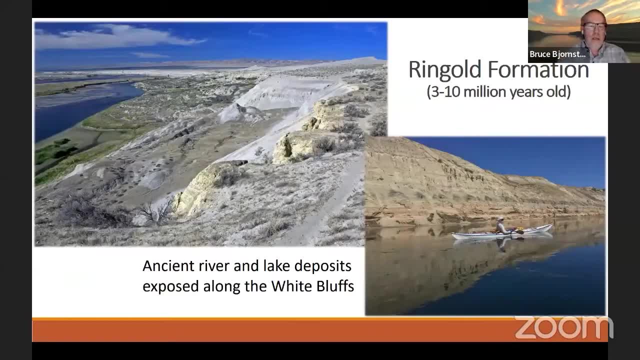 right in nearby pendleton, oregon, which is just south and west, south and eastern hanford site next. okay, so i'm moving on from the uh basalts and the next youngest geologic unit is what we call the wriggle formation. okay, these are ancient river and lake deposits, probably from the ancestral columbia and snake rivers. 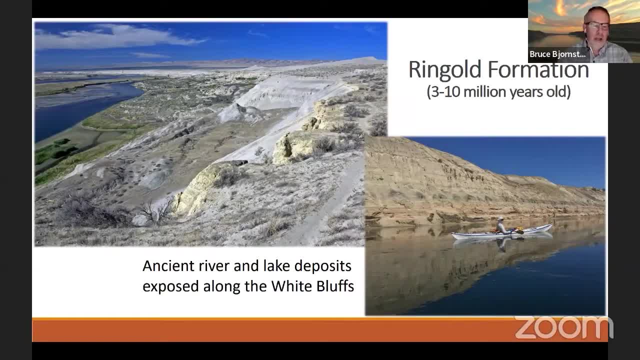 the same rivers that flow through through our area. today, we're actually uh depositing sediments within this single line, or this basin in between the saddle mountains and rattlesnake now, and depositing the wrinkled formation starting in the mid米 краves and over the greater saidalaize region. tip can be about five kilometers cargo or maybe about 10 kilometers left in the county of Indian keep we start the 2500-plus hippo, vibrant, arable, landsSam, Obama and the San Antonio. Would you like to take a closer look at the sea at this site, both Big Anticaport, artificial wildfire and mangon bloque? 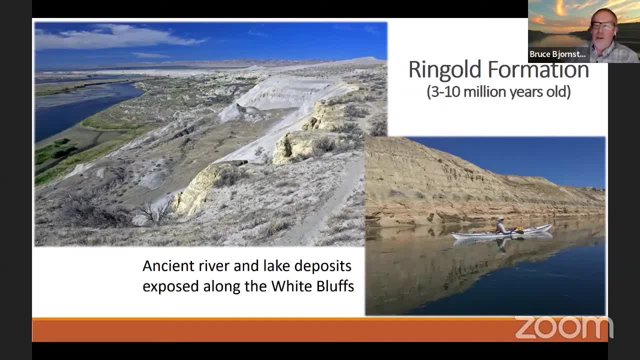 bioghy and the�imình crest trees. there are three numbers worth 10 million and 10 million feet. in Mumbai there's 13 Dé advised. there is a reduction over the nation beyond Kanto, starting about 3 million years ago, starting at 10 million years ago. 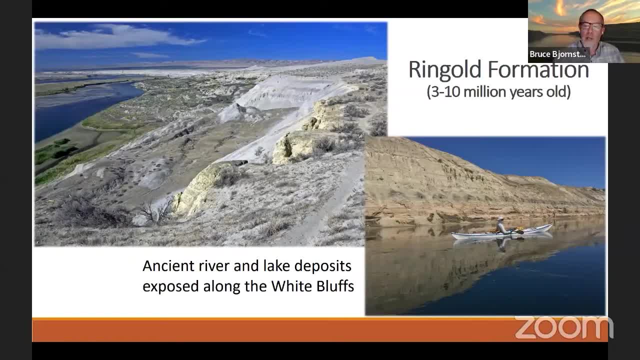 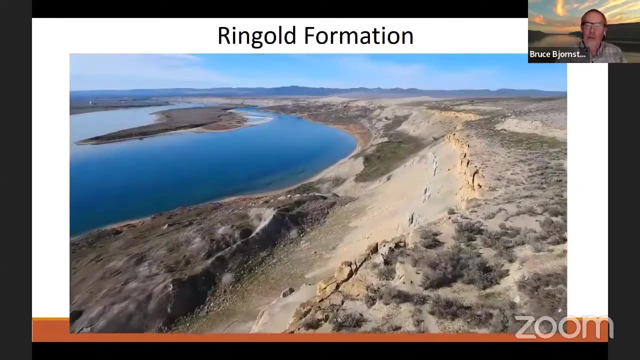 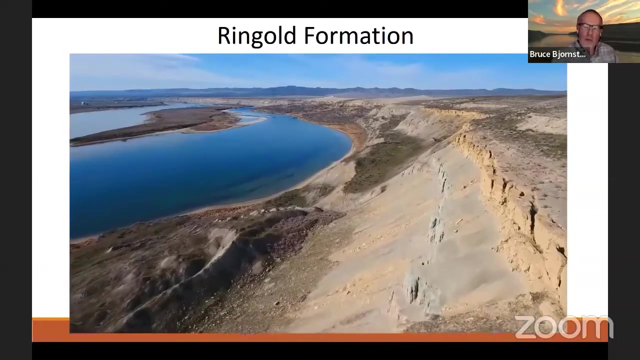 and ending at about 3 million years ago, for the ringgold formation. Next, Next, There we go. So now we have another video showing you the ringgold formation. These are mostly deposits of silt and clay here along the white bluffs. 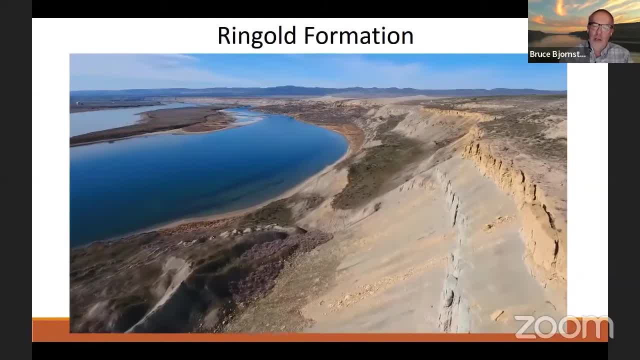 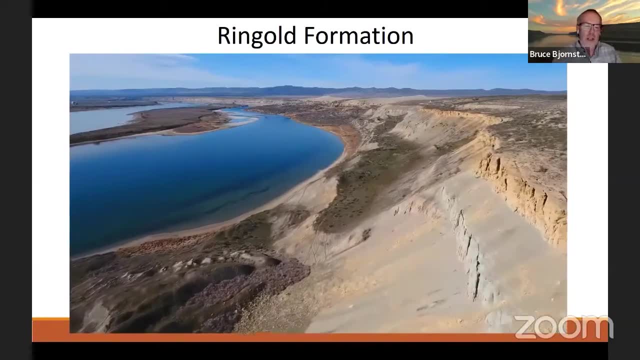 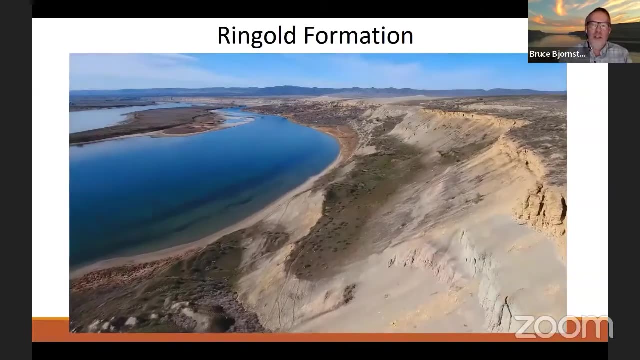 You can see the. it's very colored in brown, grays, greens. lots of clay and silt and lots of sand deposits that were laid down by the ancestral Columbia in this area and Snake River elsewhere, And in the distance you can see there's these, there's some sand dunes. 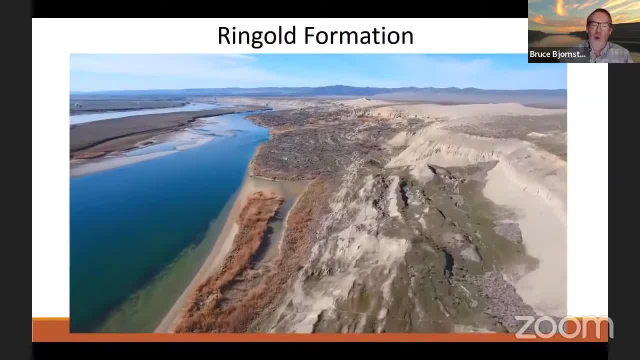 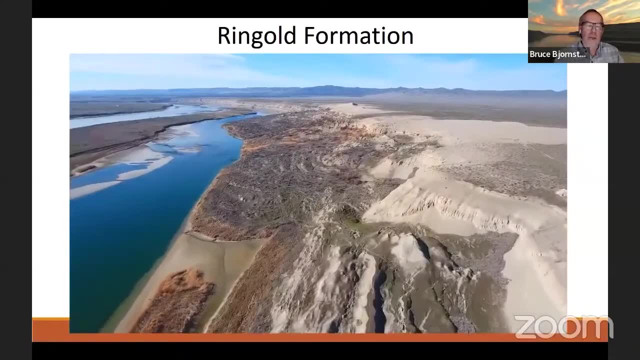 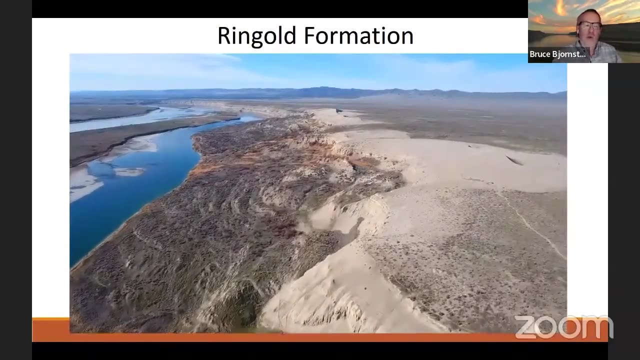 that are being deposited above the bluffs by winds that are blowing across the Hanford site against the white bluffs and then blowing sand up onto the top of the bluffs. There's a huge landslide complex there too. You can see in the middle of this image that is formed from water. 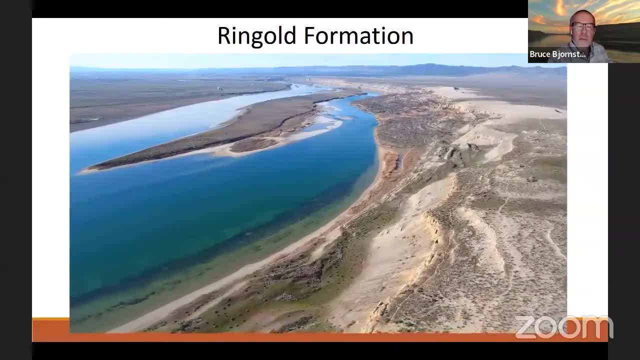 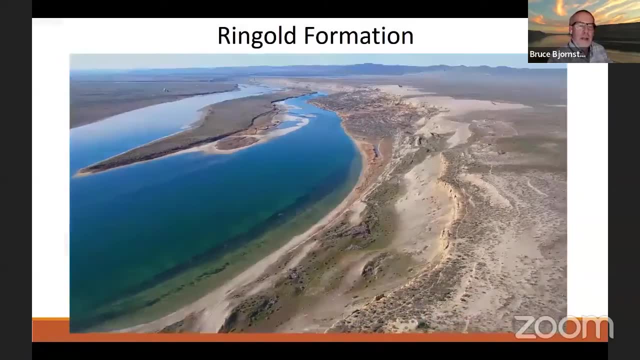 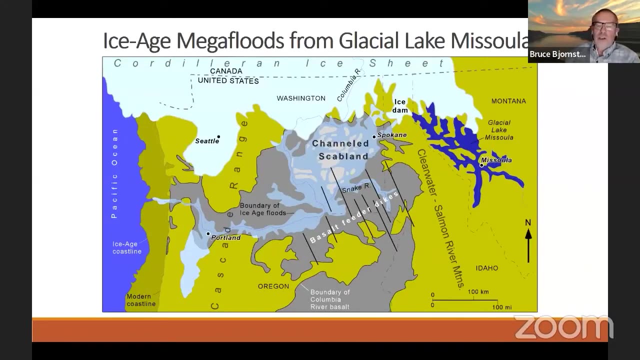 saturated sediments that have moved along landslides more recently. And there's the Hanford site is up in the middle In the upper left of this image, that H-reactor you can see cocooned there on that image. Okay, so moving on to past the ringgold formation, which ended about 3 million years ago, and then 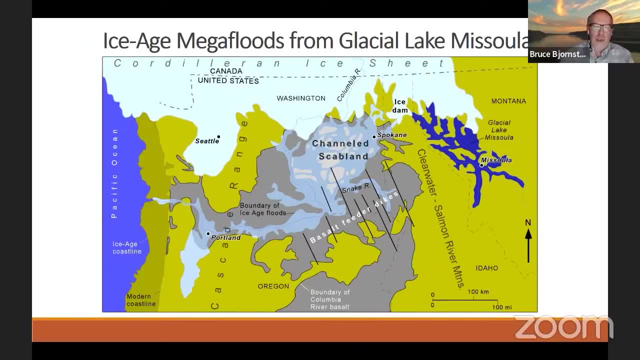 sometime around during the ice age, which started two and a half million years ago, we started getting mega floods coming from glacial lakes from the ice age. during the ice age, The most notorious floods are from glacial lake Missoula that you can see in this image. It's 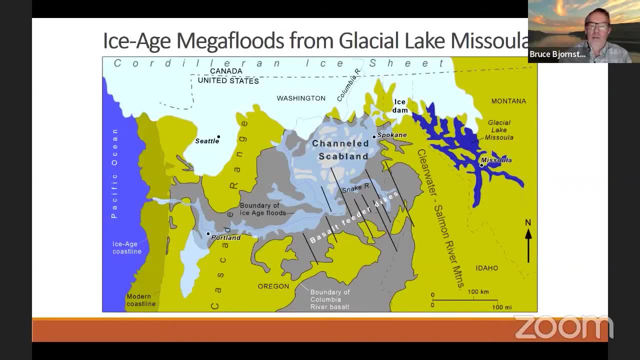 that dark blue area in the upper right And what would happen during the ice age. We know this happened at least 100 times during the last glacial cycle, but there are older ice ages that occurred previously, going all the way back to maybe one to two million years, where we had similar. 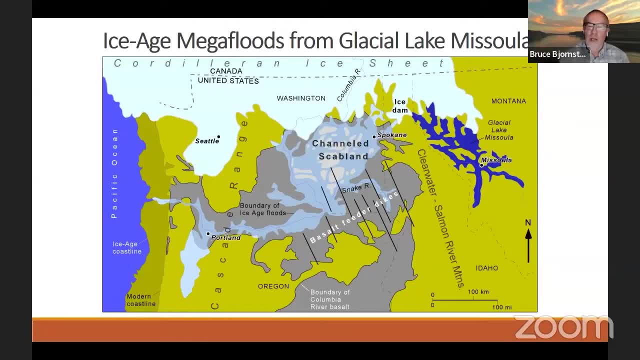 ice dams forming in glacial lake Missoula, And that's the reason why there's so many more glacial lakes forming that cause floods to travel through this, through eastern Washington. So here you can see the ice dam on the upper right creating glacial lake Missoula, and what happened periodically is that ice dam would break as the 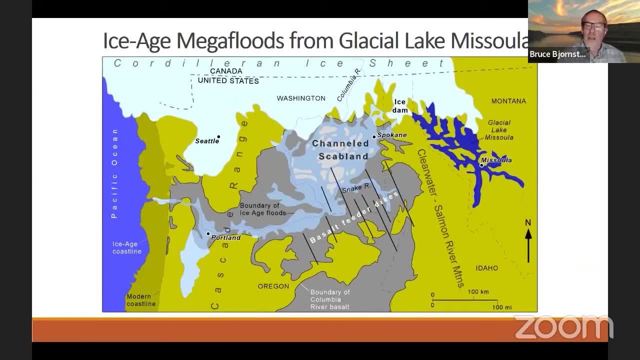 lake filled up behind it and caused all that lake water from lake Missoula to drain out In just a matter of a week or less. out across the channel, scab land, across the Hanford site Which is shown in the next. if we can, there we go. the red triangle rectangle is near the 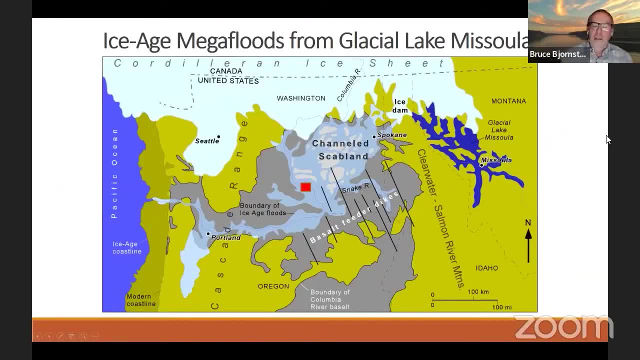 the Hanford site. There we back up, and there you can see the. these ice age floods traveled across eastern Washington through the hand by the, by the Hanford site. Now they were all forced to go down through that one little opening called the Lilla Gap, at the Idaho or at the Washington. 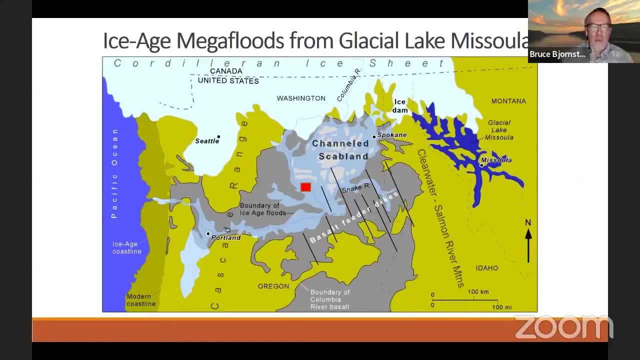 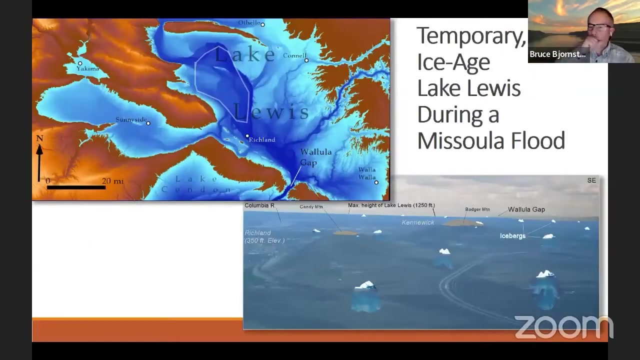 Oregon border. From there they went down through the Columbia river gorge, backed up into the Willamette valley south of Berlin, before eventually draining out to the pacific ocean. These floods all took from start to finish, lasted probably only a couple weeks or less during each one of these floods. Okay, next. Okay, here you can see the effects of the, the floods on. 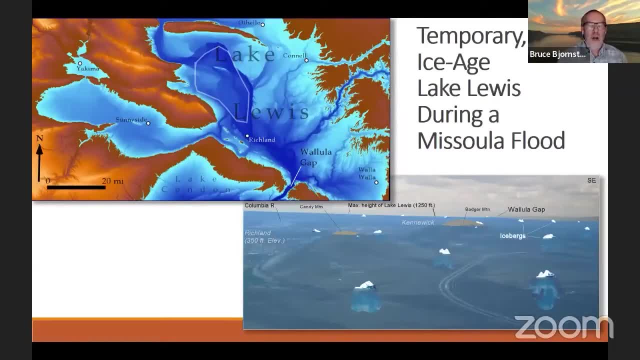 our area in the upper left. you can see I've outlined the Hanford site there but you can see it was totally submerged in blue in that blue area. that was all the back water, the flood waters coming in to the into the Pasco basin, backing up behind the Lilla Gap and flooding the Pasco basin. 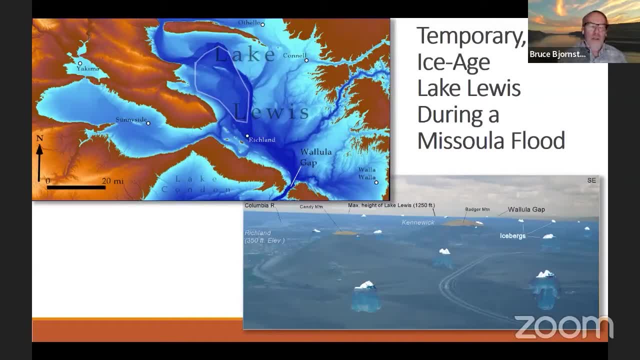 up to 1250 feet elevation, which would have completely submerged the Hanford site. The areas in brown would have been above flood level and the areas in blue were submerged. The darker the blue, the more the deeper the water during one of these floods, And in the lower right, 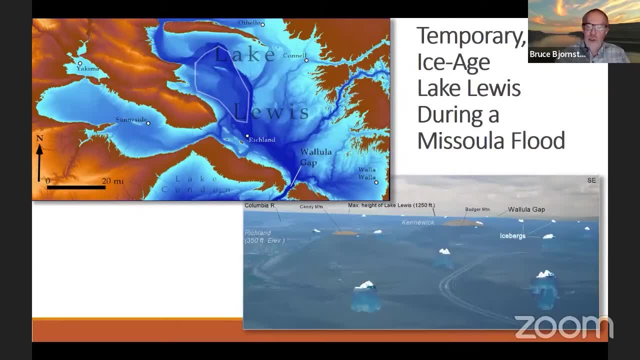 you can see an oblique view of how these flights might have looked when they came into the Pasco basin across dry cities. Just the tops of Candy Mountain and Badger Mountain Would have been islands within this lake. that was, uh, went up to 1250 feet elevation with lots of. 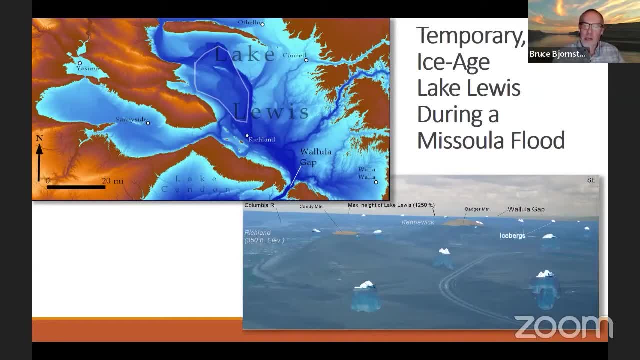 icebergs floating around from the breakup of the ice dam, from Placelet Reservoir Next, And, as I said earlier, there were up to 100 of these ice age floods that occurred between 14,000 and 20,000 years ago And we know that based on the sedimentary deposits that we see in backflooded. 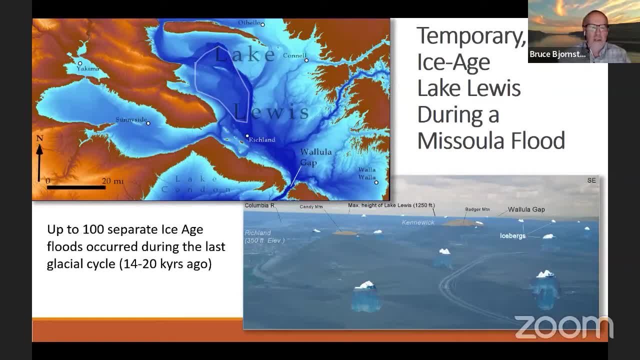 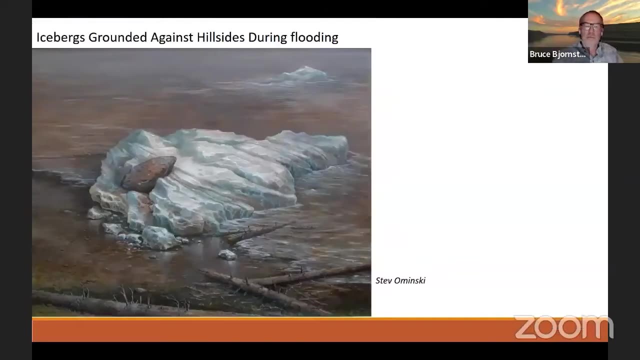 valleys like Yakima Valley, the Walla Walla Valley, the Willamette Valley in Oregon, all show these rhythmite, what we call rhythmites, Each of one, each rhythmite representing a separate flood, from Glacial Lake, Missoula Next. So here's, uh. here's an example of what one of these uh. 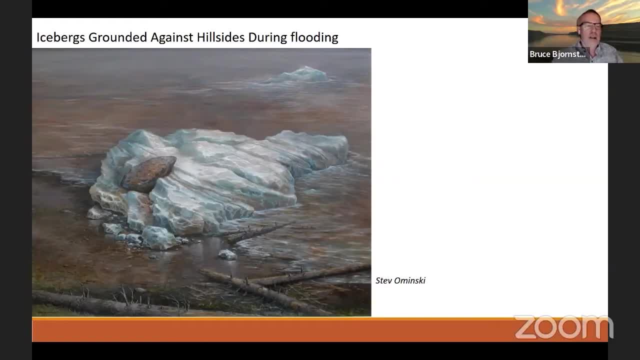 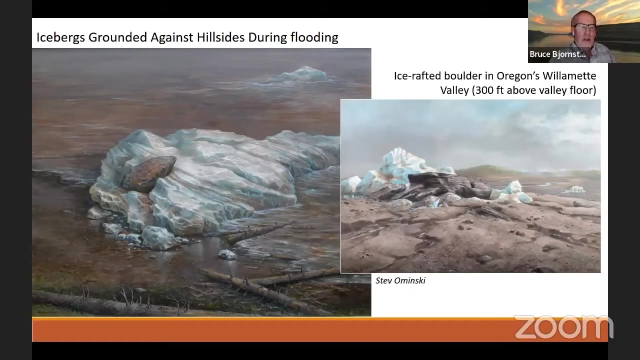 erratics that we call floated- floating in on icebergs- would have looked like, And this one, the happens to be in the Willamette Valley, It's called the Bellevue Erratic. Next, And it it rafted in on the iceberg, It floated up along the margins of the Willamette Valley. 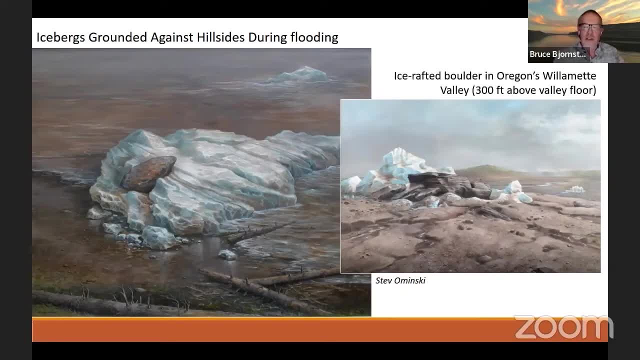 and uh, it ended up on the valley sides and the ice eventually melted. You know, within months or years, the ice melted, leaving behind uh, its payload of, uh, of boulders. It was rock boulders that were left behind and that we can see today, remnants of these ice age floods. 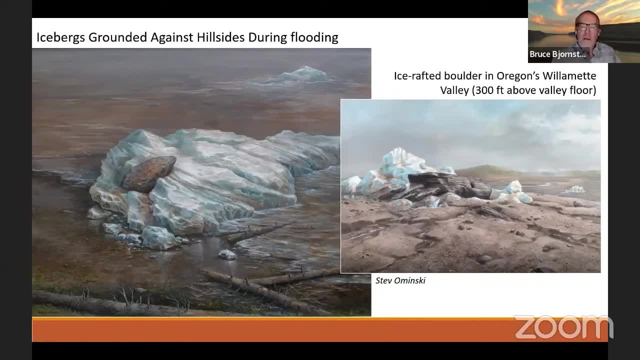 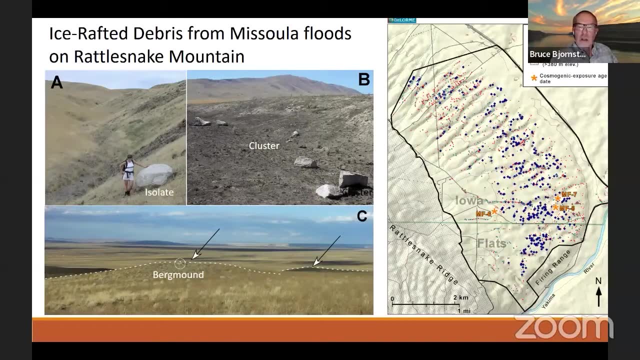 calling cards of the ice age floods. Next, And closer to home, here in the Tri-Cities and adjacent to the Hanford site on the Rattlesnake Mountain: Yeah, I've shown. here's a map of Rattlesnake Mountain, which uh borders the uh the Hanford site. 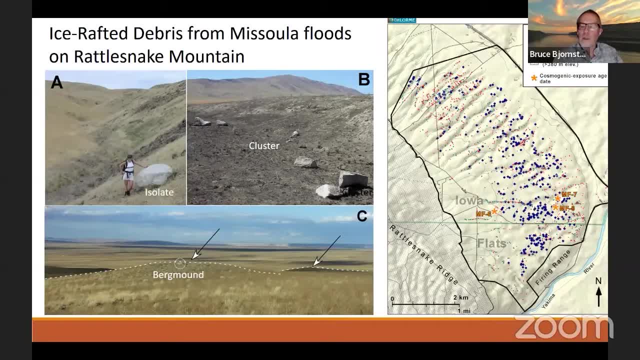 And you can. each one of those uh symbols you can see on that map is either a berg mound, which is a big pile of debris that rafted in on a really big iceberg, or a cluster of erratics, a grouping of erratics, and, in some cases, 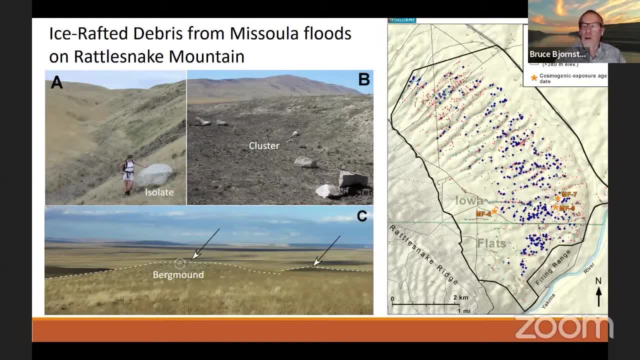 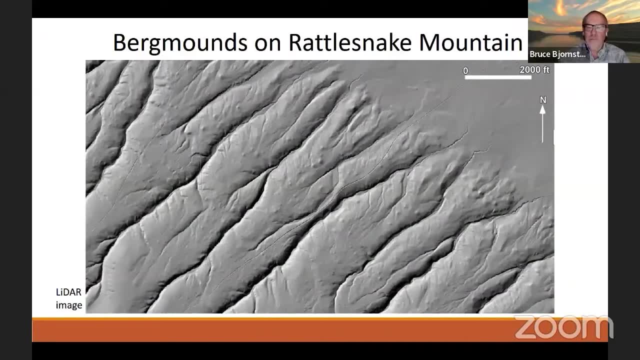 isolated erratics that are spread out across the Hanford site and Rattlesnake Mountain in particular. Next, Here's- here's a LiDAR image. This is a new imaging technique that really shows subtle changes in topography. uh, that's become available recently And these are uh berg mounds. 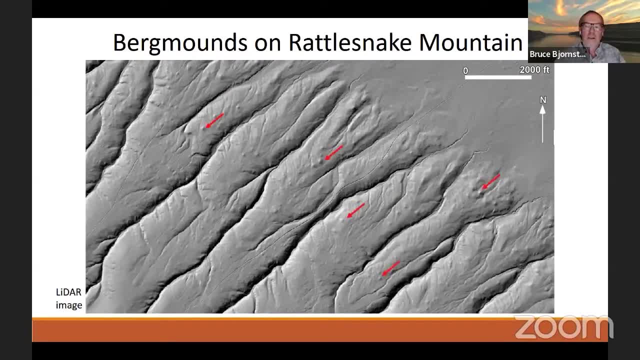 on Rattlesnake Mountain Next, And the red arrows are indicating individual berg mounds. There are hundreds of these up on Rattlesnake Mountain, as you can see on this map. Next, And the berg mounds go up to about a thousand feet elevation, but we know the floods went up. 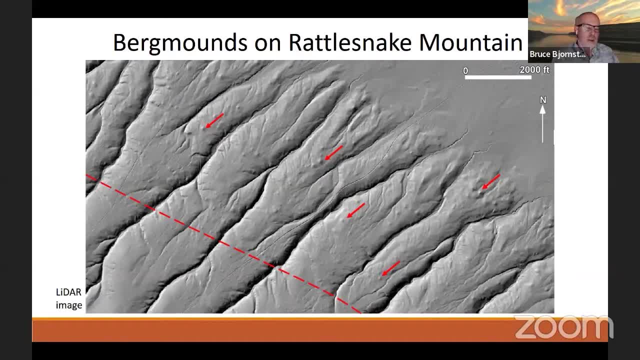 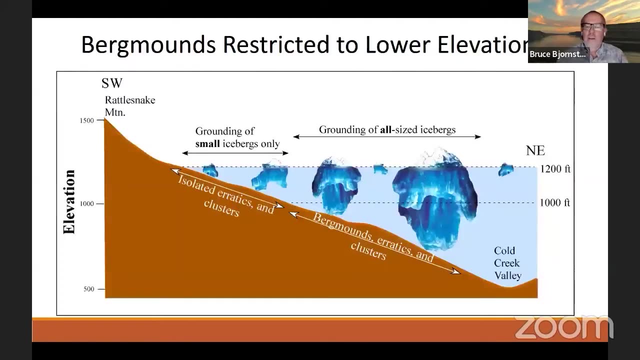 another 200 feet above that, based on the distribution of erratics up to that elevation. So why do the berg mounds, uh, why are they limited to only the lower slopes of Rattlesnake Mountain? So in the next image, uh, here's a cross section showing you how they, how these icebergs. 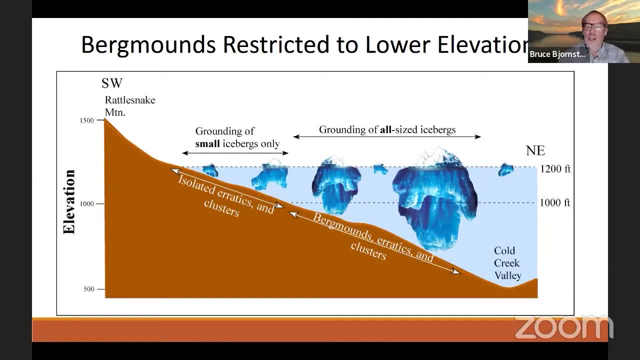 uh and berg mounds actually form The larger icebergs go deeper into the lake, lake bottom, so that they were not, they were prevented from getting up close to the higher elevations of the lake on Rattlesnake Mountain. So we have a. we have because we have bigger icebergs, we have a more. 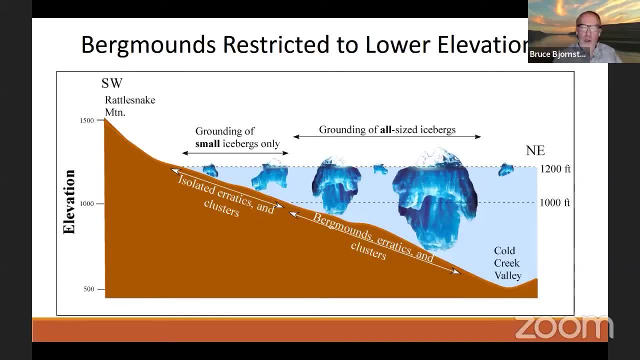 ice rafted debris, uh, in these bigger icebergs. so therefore we get mounds forming at the further away from the shoreline for Lake Lewis, whereas the smaller icebergs were able to get up up to the edge of the lake. but because they're smaller they don't have as much debris and therefore 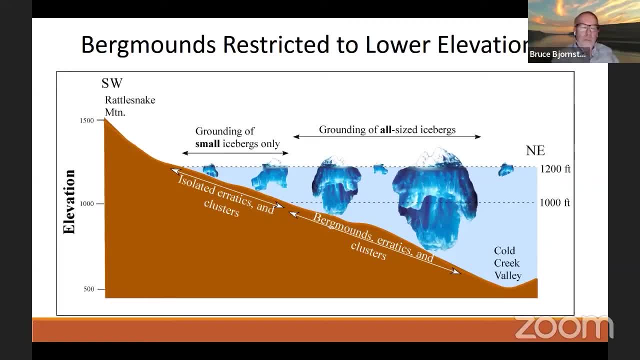 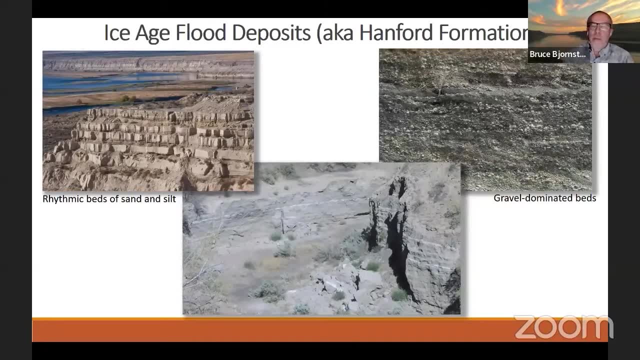 didn't leave behind icebergs or berg mounds Next. So, um, these are some examples of these flood deposits. and then, um, near the Hanford site, we have- uh, we have a a range of different types of sediments where the floods were moving really fast and furious. 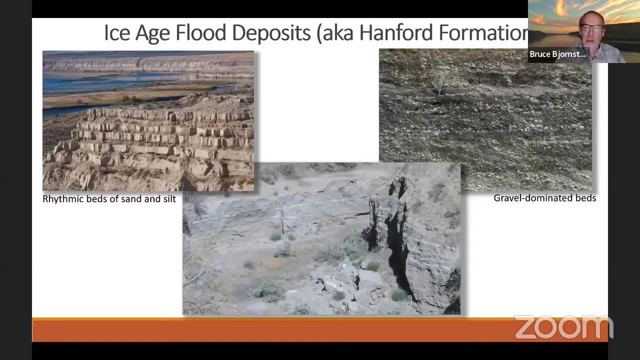 We get gravel dominated deposits, like we see in the upper right, but where the waters were able to slow down when they backed up behind a little gap around the margins of the basin, we get- uh, we get slack water deposits depositing mostly sand and silt, and those are represented on the images on the 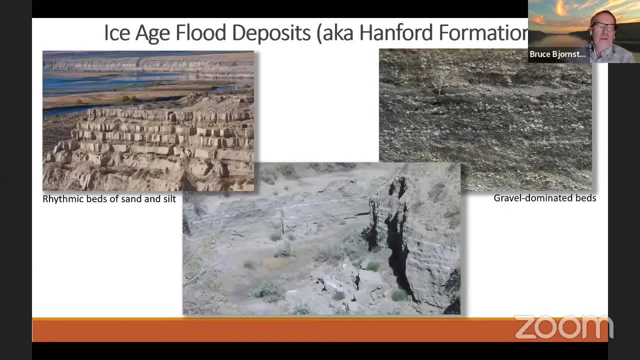 upper left and the middle there. So we we get a range of sediments deposited and it's these rhythmic beds of sand and silt that record the multiple floods that we see from from Lake Missoula Next, And in this image in the center you can see there's some rhythmic beds that are separated. 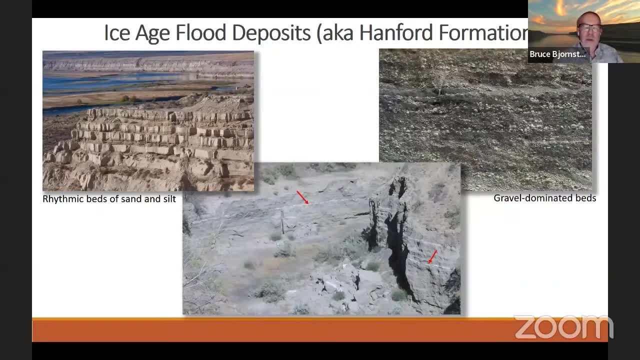 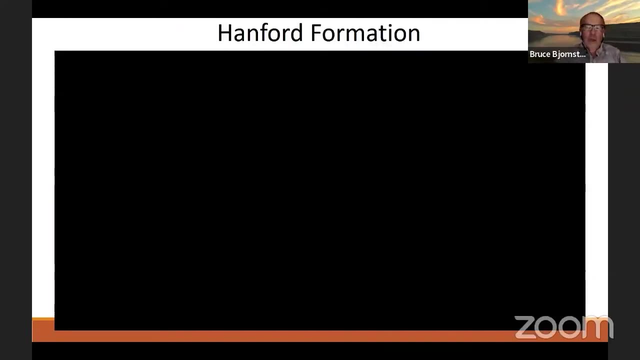 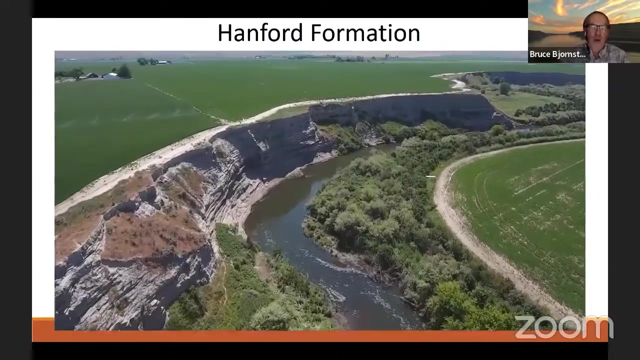 by a band, a white band, and that happens to be a volcanic ash from Mount St Helens that erupted about 15,000 years ago during or in between one of these ice age floods Next. So here we have another video showing you some of these slack water, flood deposits or rhythmites. 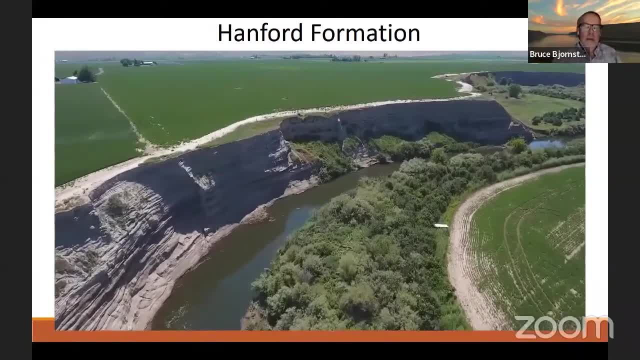 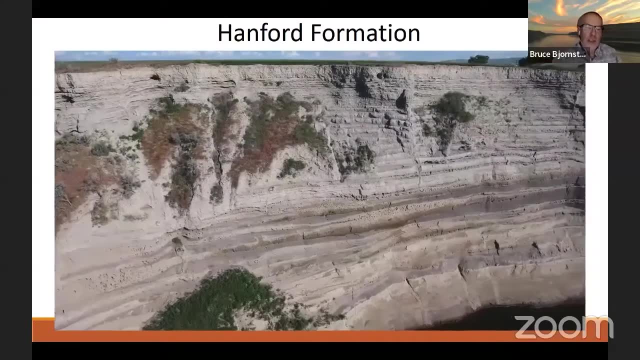 graded beds of sand and silt and gravel that is represented in the Walla Walla basin. We don't. you know Walla Walla basin is a ways away, but we have these, similar to the deposits. we've seen them in boreholes that we've drilled underneath the Hanford site. 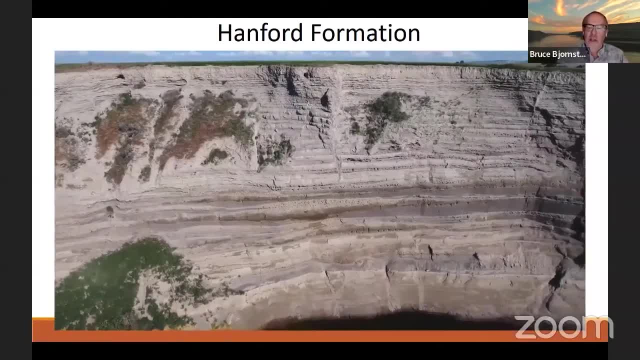 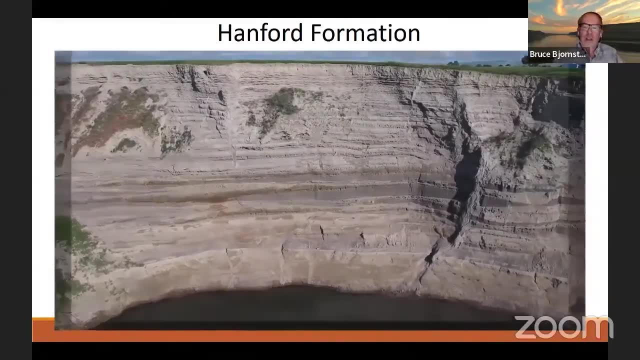 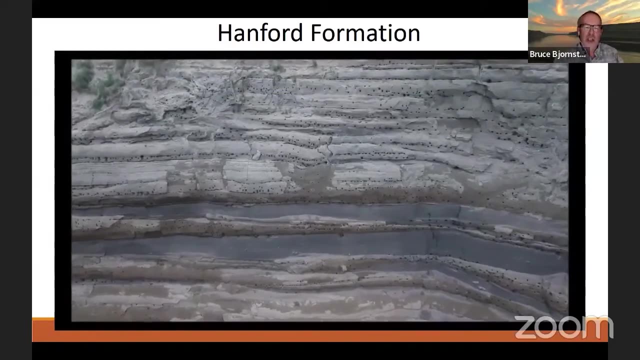 We see deposits that are identical to this. Now you can really see the multiple layers of sediment that were laid down. Each layer represents, uh, a separate flood from Lake Missoula, and here we happen, in this exposure, we happen to see as many as 60 of these rhythmites, or graded beds of sand. 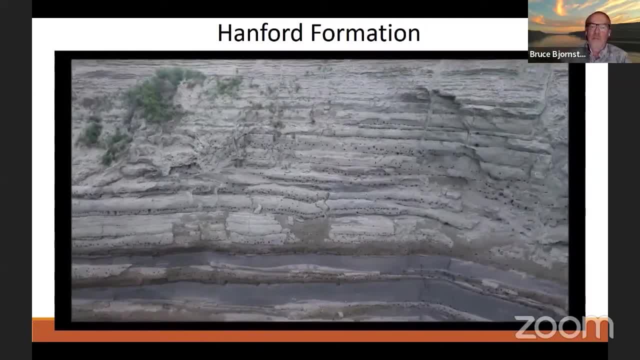 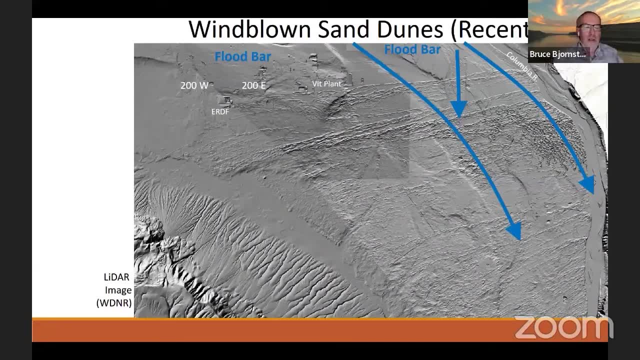 and silt that represent a separate flood from Lake Missoula. Next, As you can see, the beds get thinner and smaller as you go up section which, which is an indication of the floods were getting smaller over time. Okay, so, um, now we're gonna, we're gonna look at. 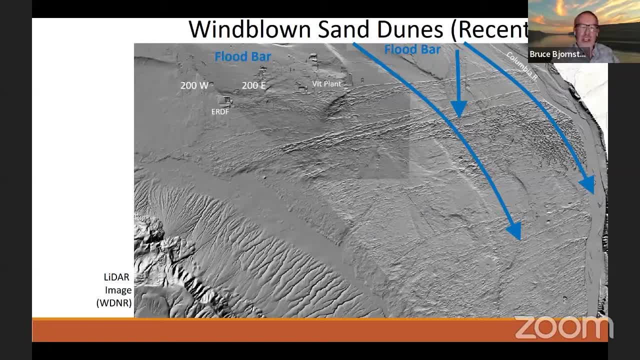 the uh sand dunes. uh, what's happened since the ice age floods? Not much has happened on the Hanford site, except there's been a lot of wind and it's reworked. a lot of these flood deposits that were deposited Brought in and on this image you can actually see flood bars. 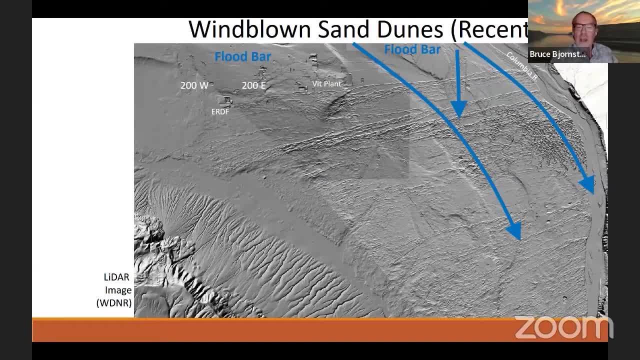 and channels. the blue air, the blue arrows are flood channels that were eroded, uh, when the floods came through the Hanford site, But superimposed on top of those flood deposits, you can see there's a thin veneer of a windblown sand and creating these dunes. Next, 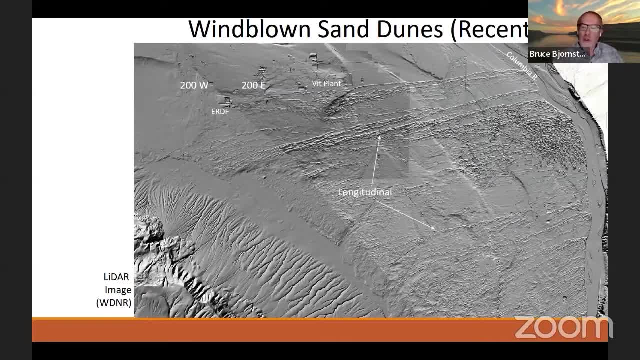 There's two types of sand, uh, sand dunes. there's these longitudinal dunes that trend uh, that go for miles and miles, mostly in an east-west direction. and then we have another type of sand dune, Next Called parabolic dunes, and the parallel parabolic dunes. you don't see them. off to the west as much. they're kind of restricted to that one little area next to the river. and those are there because of uh Ringgold Coulee, which is a flood coulee, And it acts like a wind tunnel. the predominant wind direction is coming from the southwest. 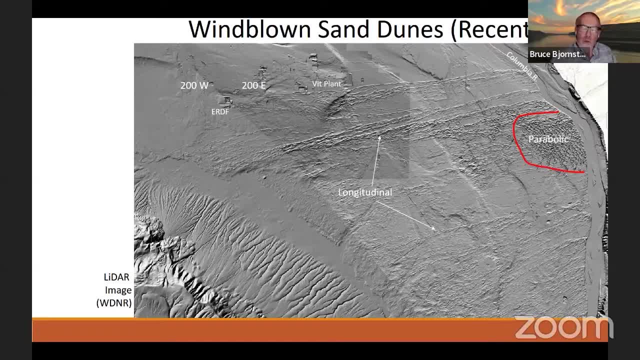 so that these longitudinal, longitudinal dunes form, uh, to the north, south, but they're in the middle that, the parabolic dunes- we have a wind tunnel effect that created these beautiful parabolic dunes, are true- are arc-shaped dunes, uh, in this one restricted area. Okay, so next. 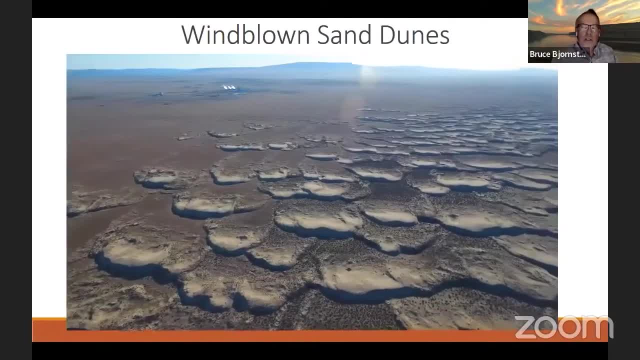 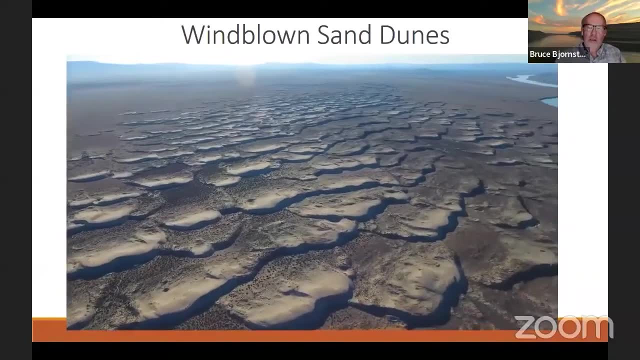 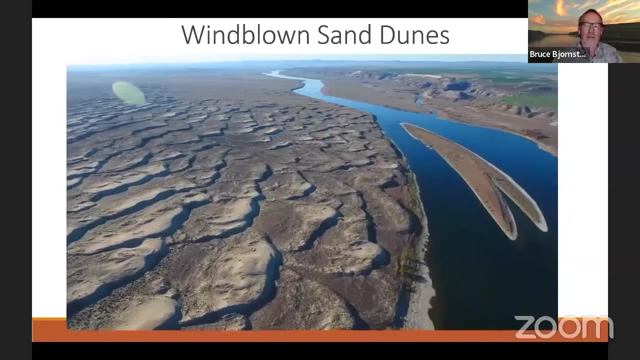 And here's a, here's a drone video showing you these parabolic dunes, looking kind of to the west. They're beautiful sand, they're very active. I mean, they're still moving today, they're very active. There's the Columbia River and, uh, Ringgold Coulee is off in the upper right. so that's, that's a lower. 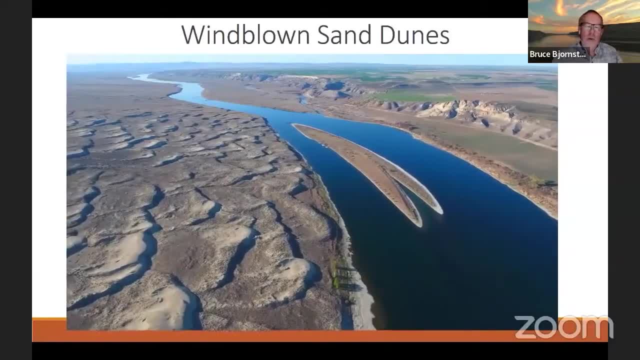 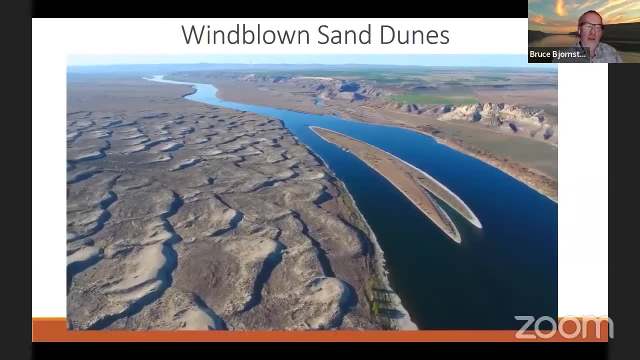 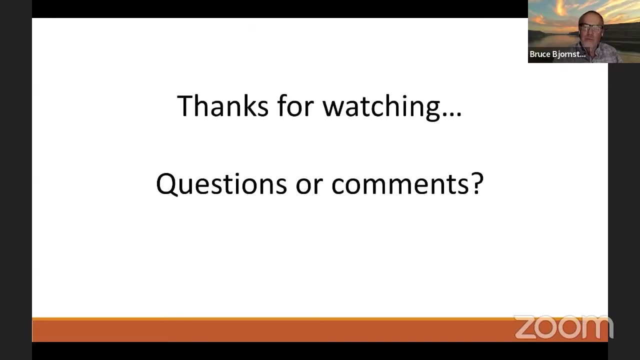 area where the floods are routed to channel and the winds, coming from the west, preferentially blow Through across Hanford up Ringgold Coulee and therefore have created these isolated uh parabolic dunes that we see here. Okay, so that's the end of my uh the slideshow and I guess I'll let uh. 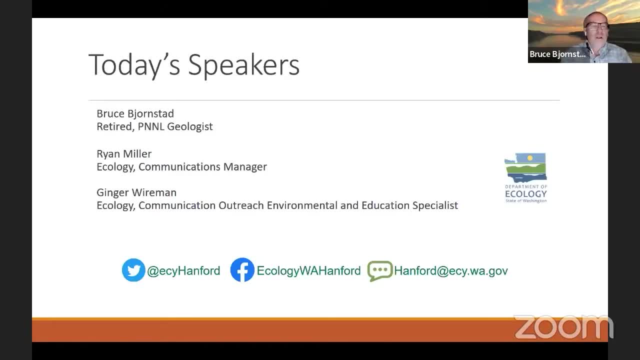 Ryan and Dana and Ginger. uh, take it, take it, take over from here and I'll answer any questions. Perfect thanks, Bruce. that was an amazing presentation and I know we especially appreciate, you know, the time you took to put that together and- and we do have a list of questions that are- 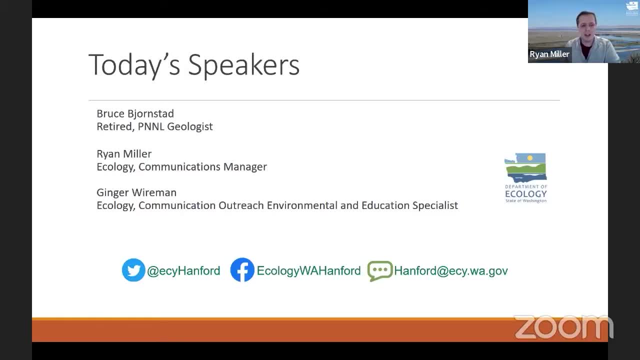 that are ready for your answering here. Um, I'm going to go ahead on zoom here and turn on the features for for guests to unmute themselves and start their video. I would appreciate, though, if, if, anybody would like to unmute themselves and ask a question that you just say you'd like to ask a. 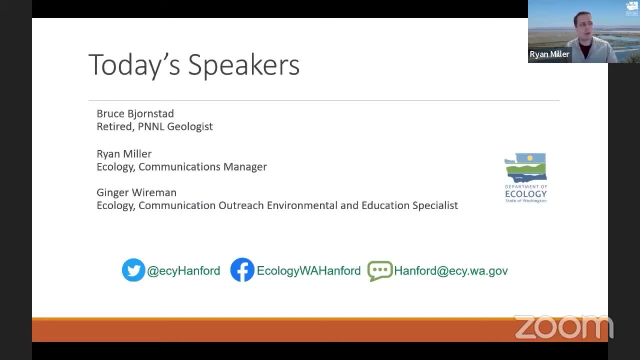 question in the chat. that way we don't get a lot of people speaking over each other. We do have one person so far that that did say they wanted to unmute, So I'm going to let them start their video. Um, so let me go ahead and turn on those features and we also have, uh, Facebook questions. we'll ask. 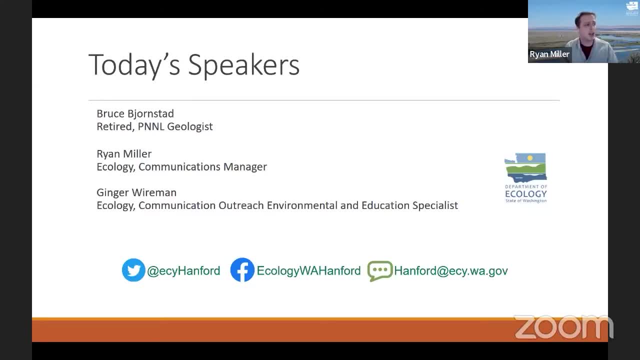 as well? Um, all right. so, Maya, I believe you had a question and you should have the option to turn on your camera and unmute. now if you want to ask Bruce your question, Hi, yeah, thank you so much for the presentation. I was just wondering. welcome, um you, you spend time looking at the past? 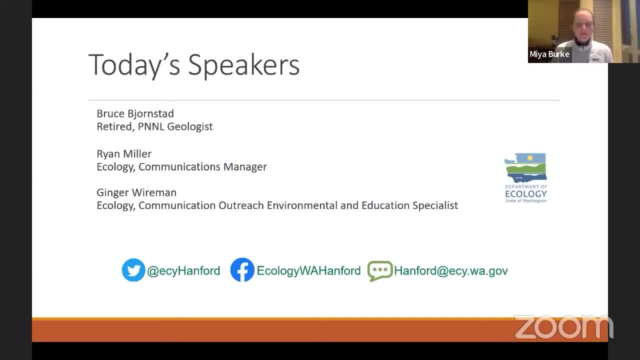 of Hanford's geology and I'm wondering if you can use what's happened in the past kind of predict the future of what will happen, let's say, 10,000 years from now, what the the geology specifically at Hanford will look like. For example, like would the Columbia River move um? 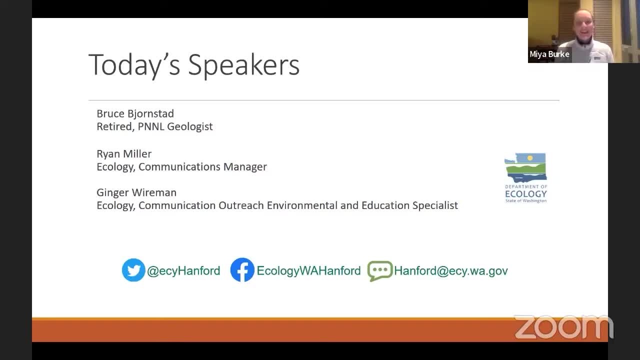 any, any kind of insight into that would be much appreciated. Thank you, Okay, okay, well, yeah, that's a really good question. Unfortunately, I don't have a crystal ball, but, um, like we can you know, the past is maybe an indication of what's in the future. The Yakima folds will are are continuing. 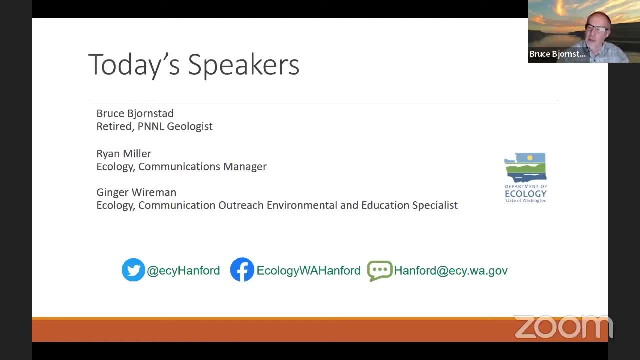 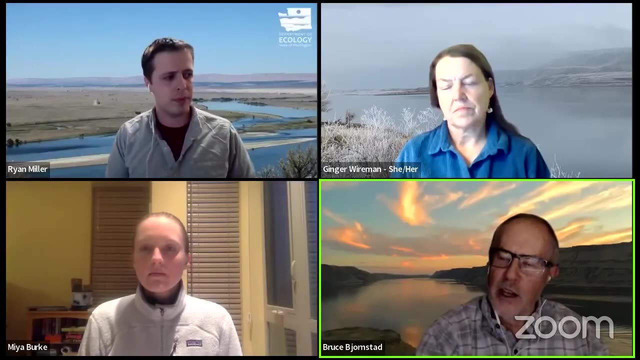 to grow and they're still growing today. So these ridges are going to keep growing, uh, getting probably bigger uh over time, and there there's uh very likely uh going to be ice age floods again in the future. I mean we. the history of flooding goes back two and a. 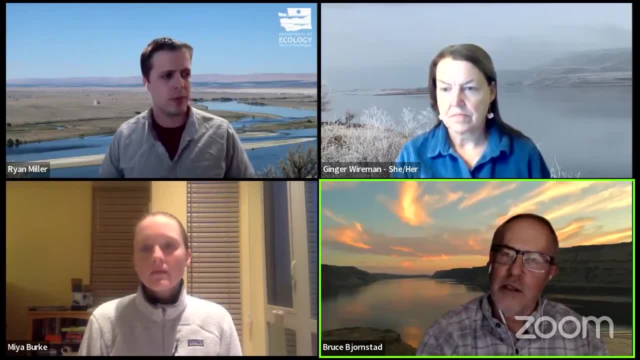 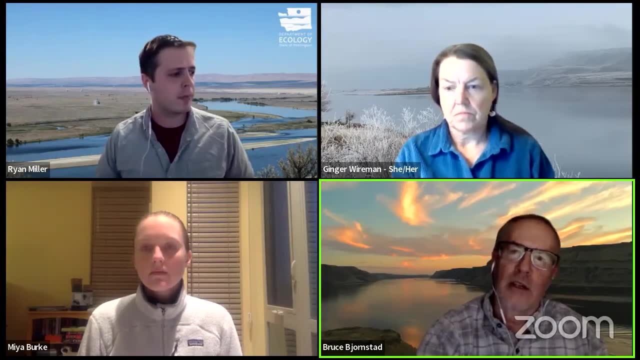 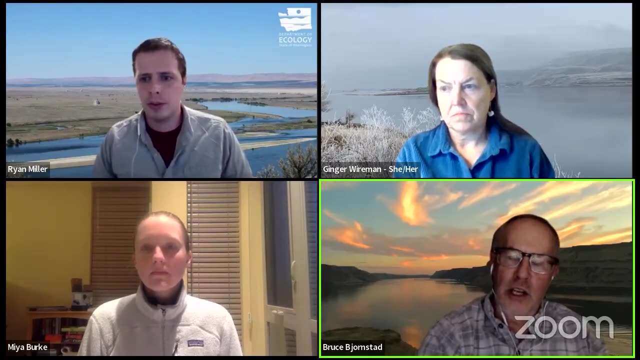 half million years And, uh, the last event was 15,000 years ago, so it's they'll be, unless we've permanently changed the climate. uh, due to global warming or whatever, uh, we should go back into another ice age because, um, they, they have been very cyclic and they've been occurring for for millions of years. So, it's likely that there could be other other ice ages in the future and more ice age floods, Because the the all the elements are still there for for flooding to reoccur, except for an ice dam which isn't there now but that could be in the future. So I'd say it could. you know there'll be. 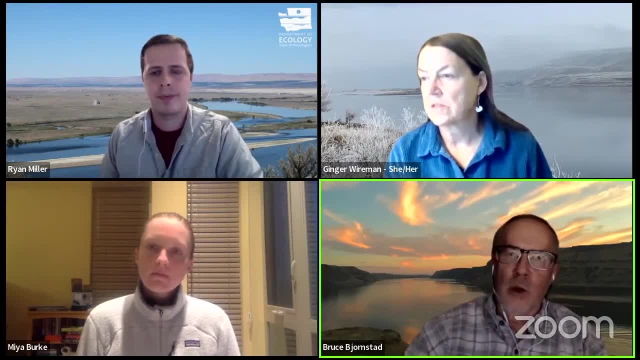 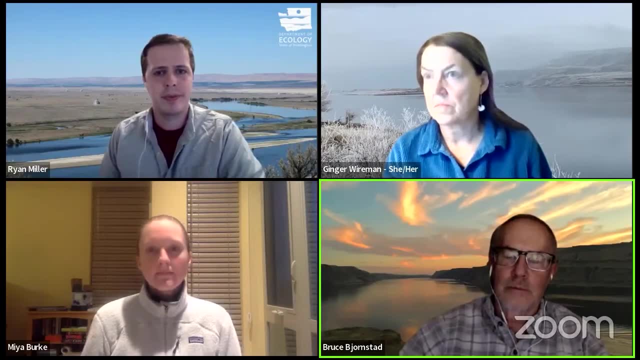 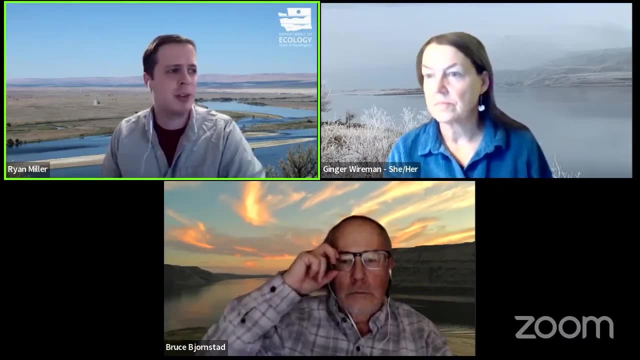 there'll be more changes maybe, uh, similar to what we've had in the past, and who knows what what other changes might occur? Wonderful, thank you, Bruce, and thank you Maya for your question. Um, we'll skip over to Facebook For a question here. this one was asked by Anthony early on in the presentation. Bruce, 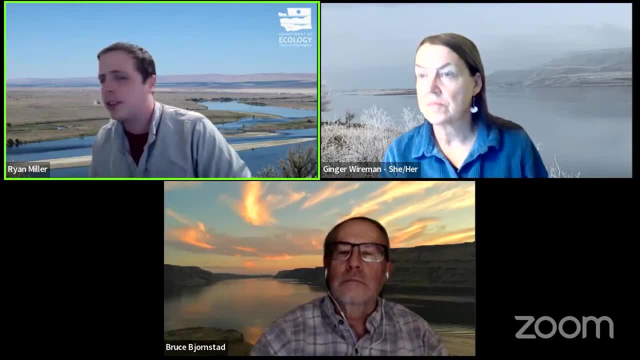 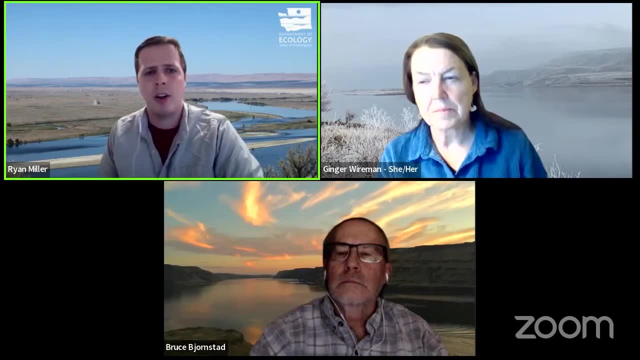 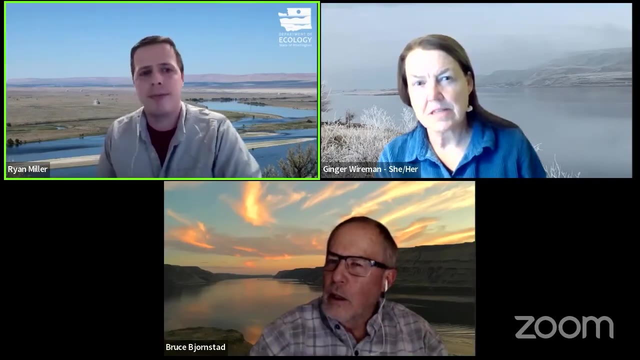 Uh, he asked: what size are these holes? and I think that was in reference to the slide that was covering the typical hydrogeologic cross section. on that slide, or the slide before at least What, what size are what the holes? Yeah, Does that mean the wells? Oh, the wells. 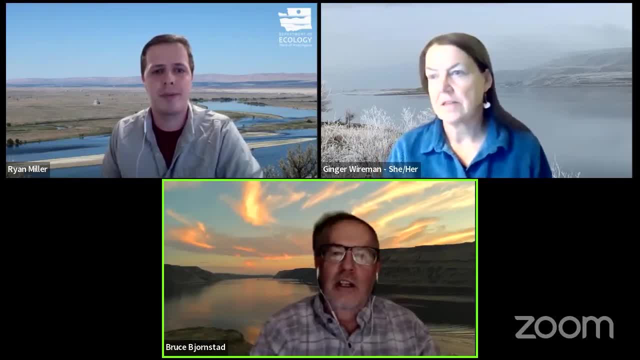 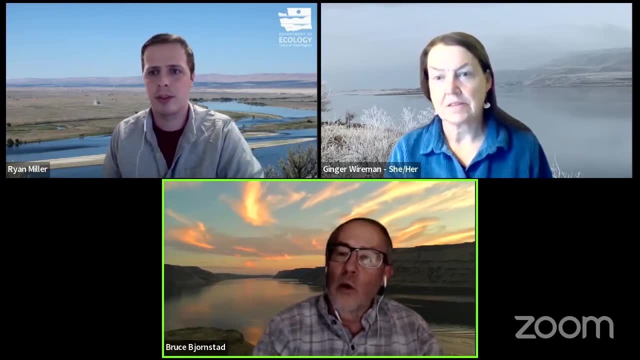 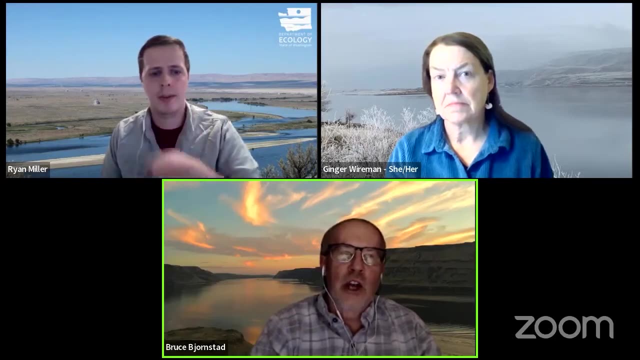 The drill holes? yeah, they're. uh, they vary in size, uh, from a few inches up to a foot, or even bigger in some cases. So, yeah, those they're there's. they're small boreholes, generally uh used for drilling. they're what. they're cheaper: the smaller they are, the cheaper. 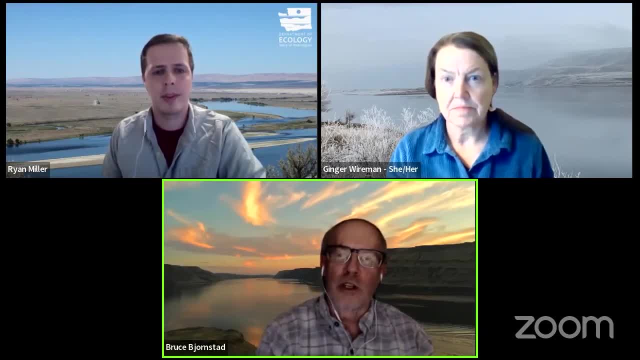 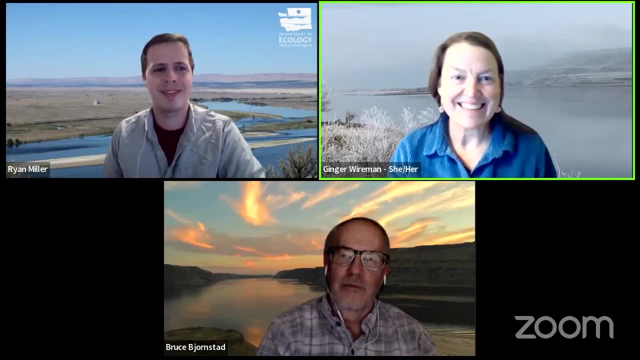 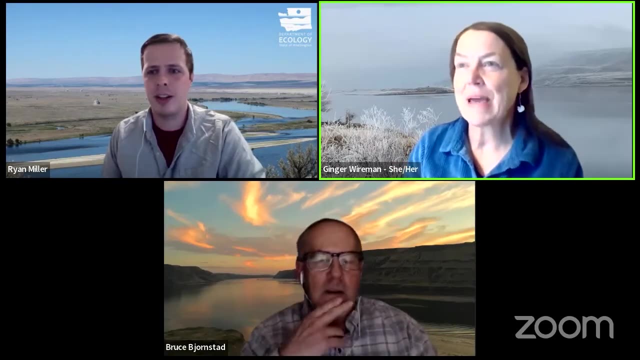 and the more you know, the more you can get, the more wells you can drill by using smaller holes. So they're pretty small. So, yep, Okay, we had a question in uh Zoom, from John Panasik. I hope I pronounced your name right. John, what originally caused the gorge to be where it is? Okay, well, the Columbia Gorge, uh is has probably been there for, uh, at least 20 million years. Um, and it it actually it was flowing through where you're aware it is today, when the Columbia River basalts were coming out 17, 7, 17 million years, as far, as far back as 17. million years ago Columbia Gorge was going. the basalts were going in and through the Columbia Gorge and getting out to the Pacific Ocean. they're actually lava flows, basalt lavas, out on the Pacific coast. Okay, Yeah, That came from eastern Washington or eastern Oregon, so, uh, it's been at least 17 million years. 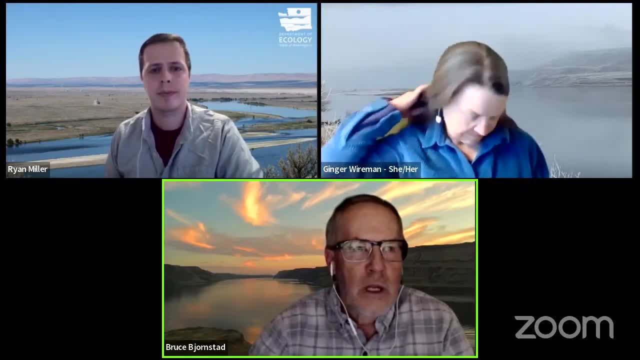 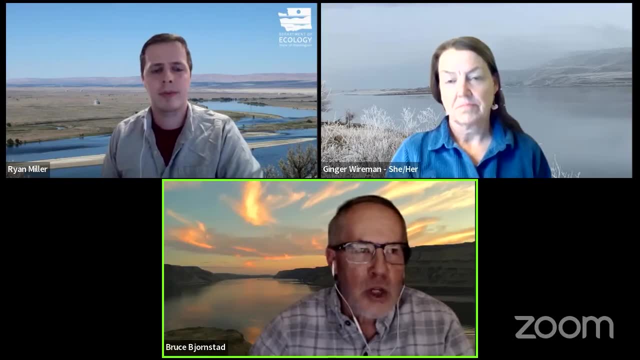 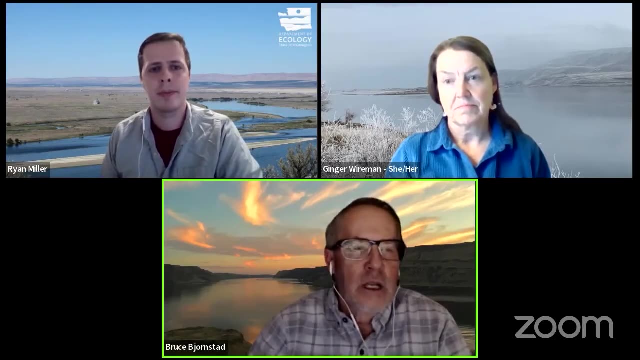 and uh once it started. you know, once the, the river got established, it would tend to just keep going in the same direction, even as the. as the Cascades were growing, the river was able to keep up with uh down, cutting uh through any of the uh Cascade volcanics that were accumulating in the gorge. Yeah, Yeah, Once it got established, we just beat through and cut through those and then, uh, keep going as it had been so, but it's been there for at least 20 million and maybe, uh, uh, maybe as as long as 40 million years. 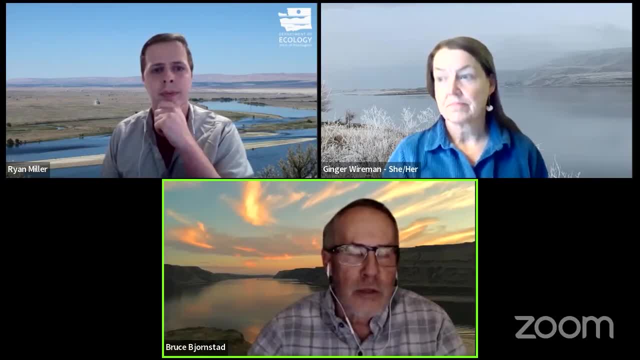 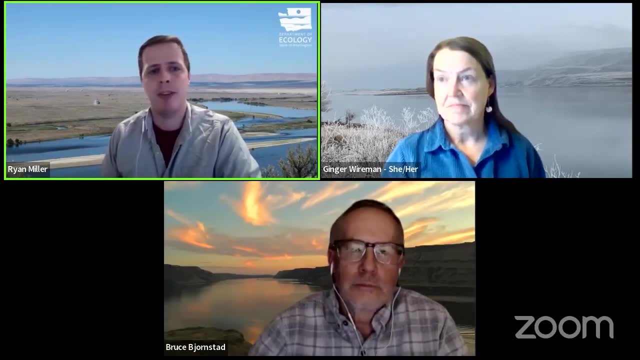 ago. we've had the Columbia River kind of going where it is today through the Columbia Gorge. Perfect thanks, Bruce. and I see we've got more questions on Zoom, in addition to Facebook, of course, and I'll just remind folks that if you guys do want to unmute and turn on your camera, 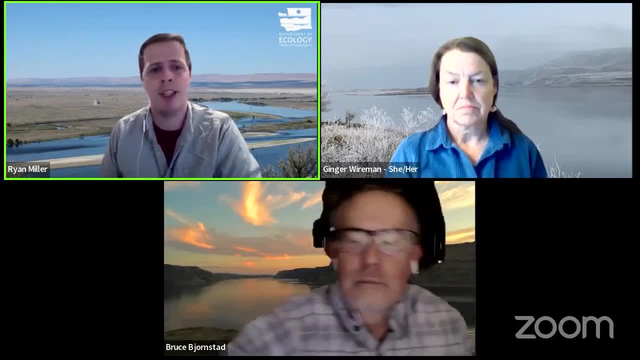 and ask Bruce your question. go ahead and make that note. Okay, I'm gonna ask a question on the chat, otherwise we'll just assume that you just want us to read the question and we'll go ahead and do that. um, but over on Facebook. bouncing back to Facebook, we 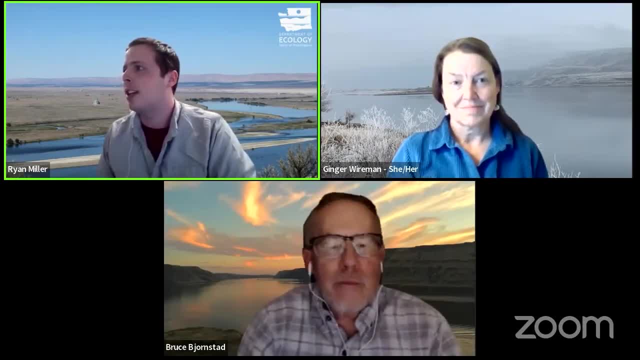 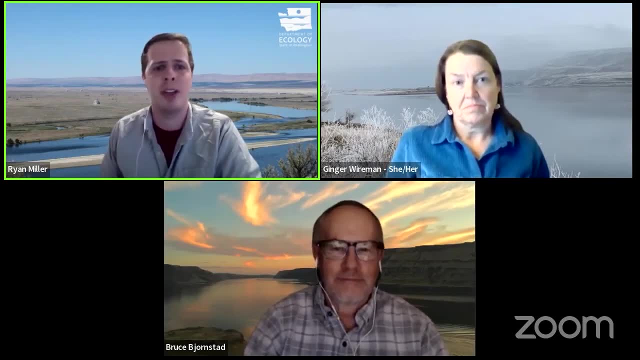 had Susan Leckband ask a question and she asked: are the decommissioned wells filled in so that they don't allow a pathway for contamination to seep into soil or groundwater? I'm not sure if that's a question to answer now, Bruce. 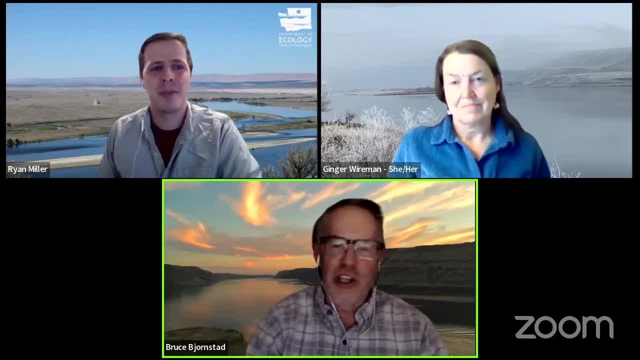 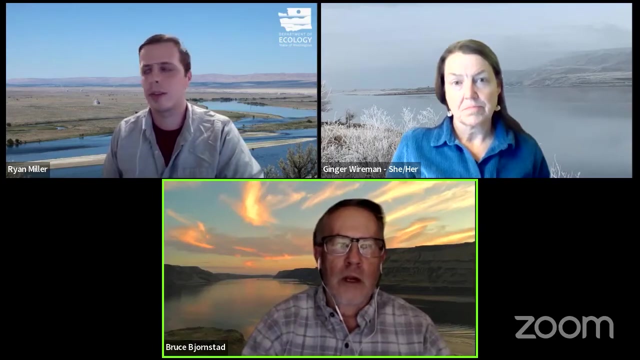 Oh yeah, and that's yeah and there's. the answer is yes. They're very, uh careful about well. they don't want to create any pathways for contaminants to move. so whenever they decommission a well, that's how it is backfilled. it's usually backfilled with clay, a very like a bentonite clay or cement, so that there's no. 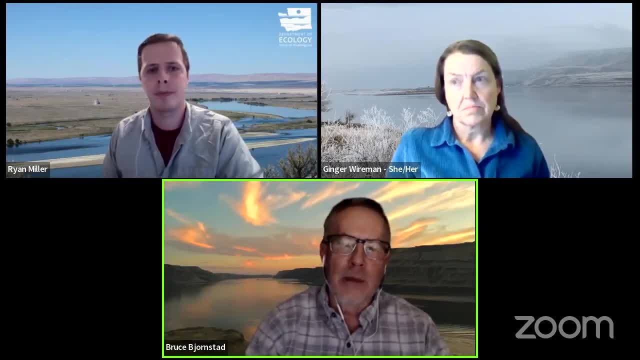 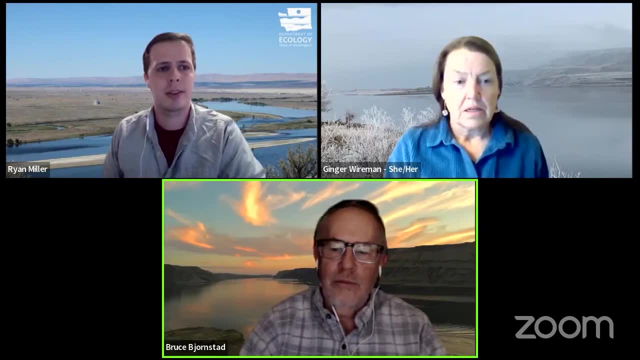 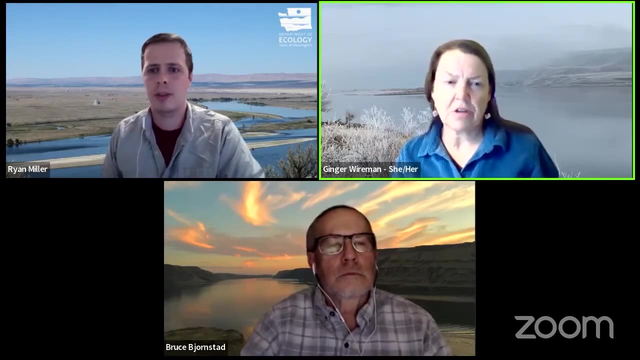 chance for it to transmit any contaminants that might be moving through the area. We had a question from Mark Hatchup wondering where are the decommissioned wells in the area? Where are the gravel deposits pictured? That is one problem with waiting till the end because we don't know what slide you. 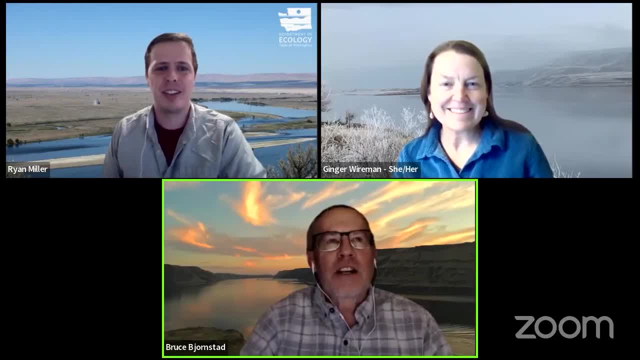 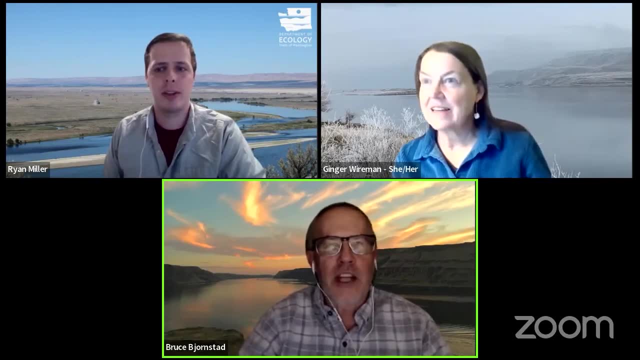 might have been referring to Gravel deposits for um, for the flood, the flood gravel. I wonder if that's if that's what he's asking. if it's the flood gravel, which is, yeah, that's, that's the most common gravel type deposit in in this area and in Hanford. 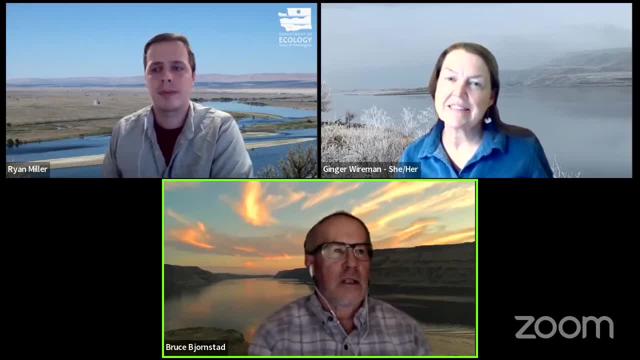 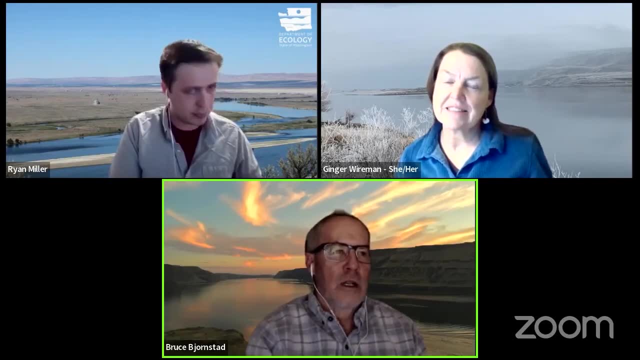 Those uh, that picture was taken uh with the flood gravels was taken just north or near Richland, but those flood gravels uh go all the way up the Columbia River to Sentinel Gap. they tend to disappear as you go south uh through across the Hanford site. 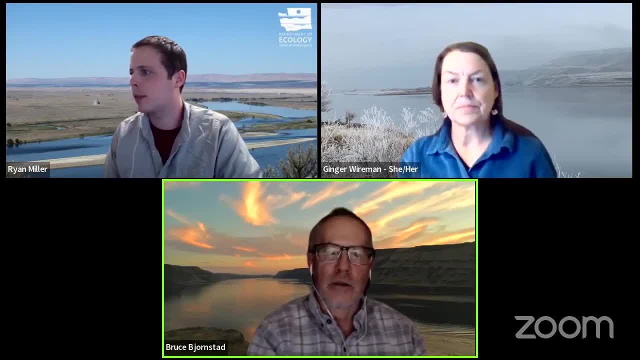 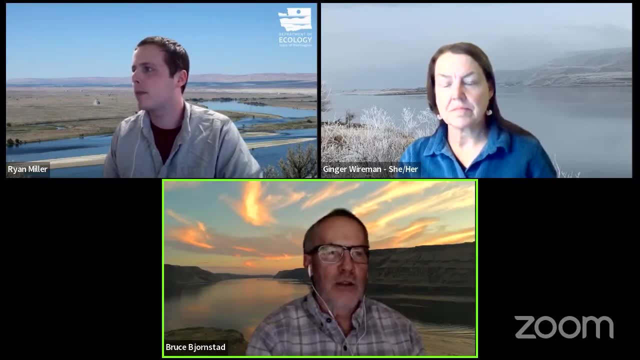 because that area was further from the high energy of the floods in those areas, uh to the south, or mostly sand and so so the gravel is kind of restricted. the flood gravels are kind of restricted to the northern and eastern part of the Hanford site. 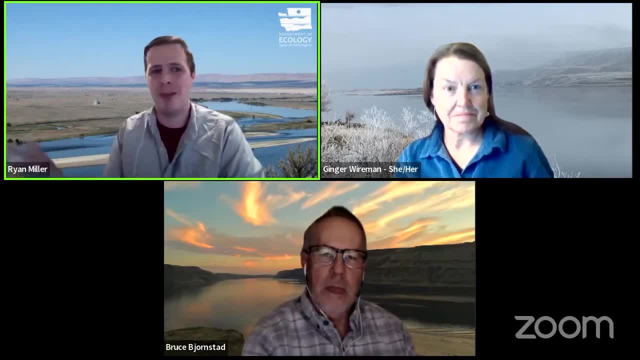 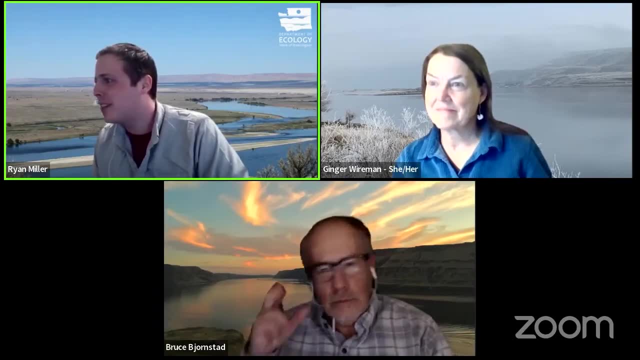 Awesome. thanks, Bruce, and sorry everybody, if you see me looking left and right. I've got a couple different screens up with uh questions. We've got another question on Facebook here for you. This one was asked by- let me scroll down here- um, by Ryan Bailey, and Ryan asks: is Badger Mountain? 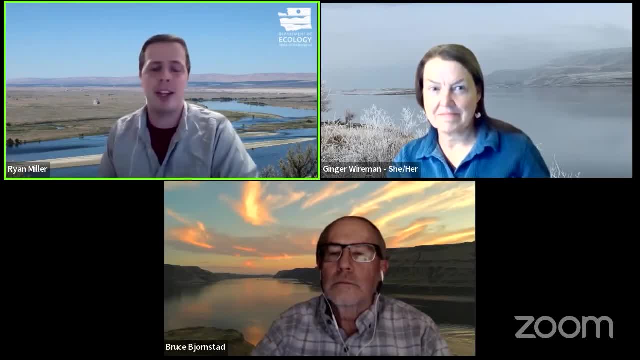 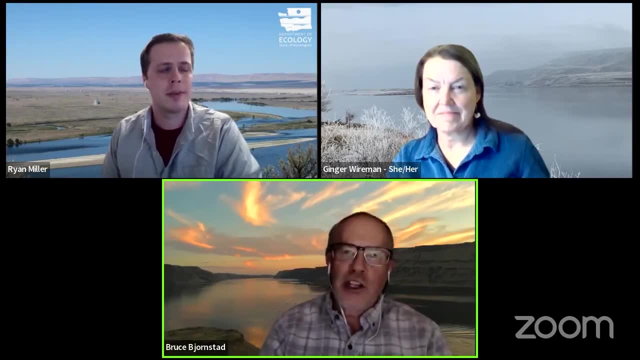 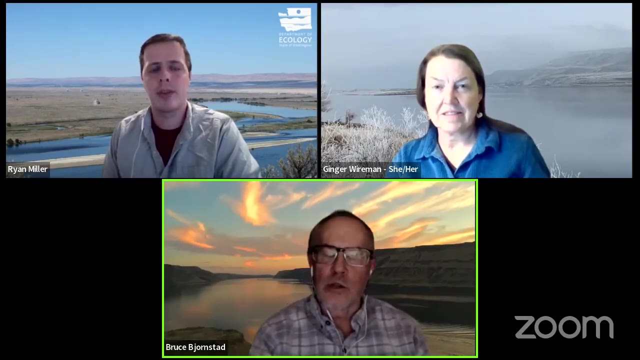 Candy Mountain, Red Mountain and Rattlesnake Mountain, all part of the rattlesnake fold. Um, that's all part of what we call the rattlesnake lineaments, or the Olympic Wallowa lineament trends along those, those hills, those structures. 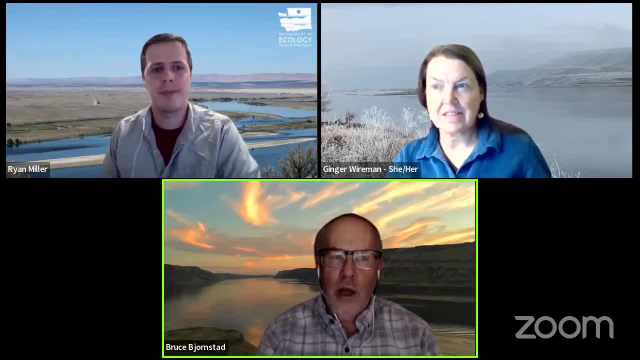 and the rattlesnake fault is. there is the right, there is a rattlesnake fault, but that's kind of. it's kind of uh, restricted to the rattlesnake mountain. The rattlesnake mountain fault is also part of the the raw and the the owl, so there it's one. 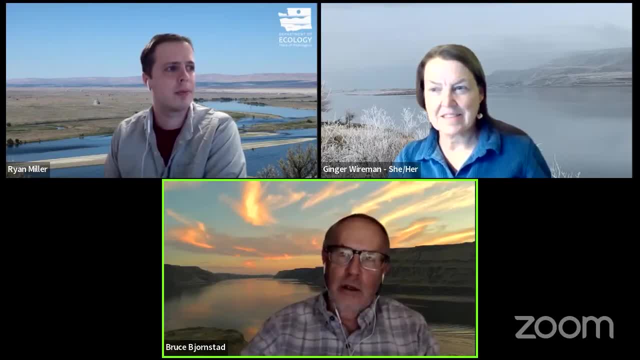 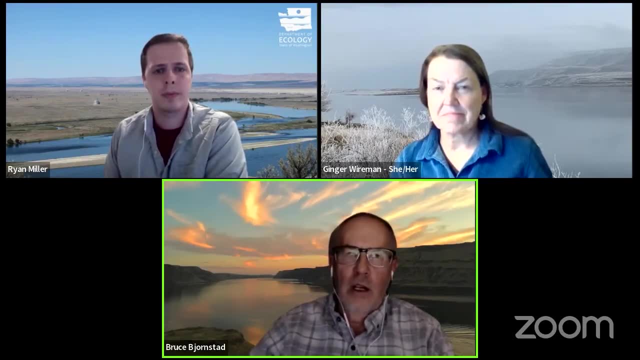 very long feature. the rattlesnake fault is just one part of it. but those ridges uh- Candy Mountain, Badger Mountain, Red Mountain- are all on that same alignment so they are connected and they are related to the same uh tectonic uh. 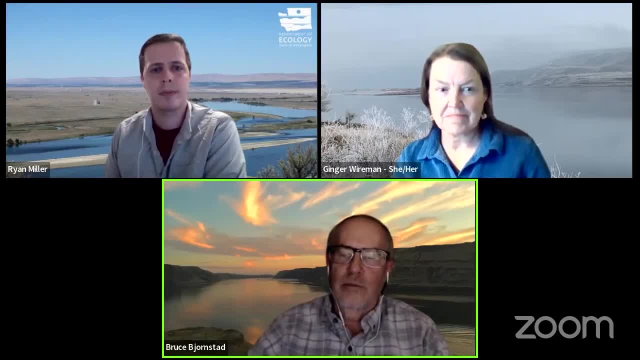 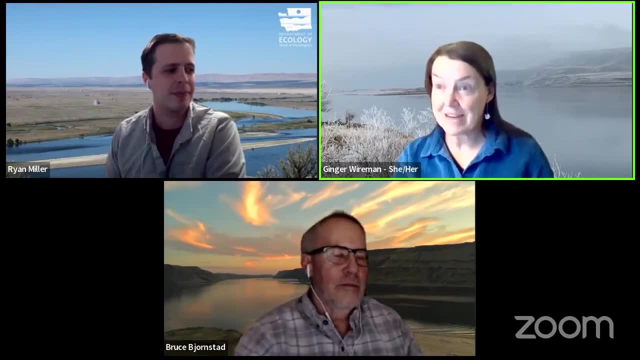 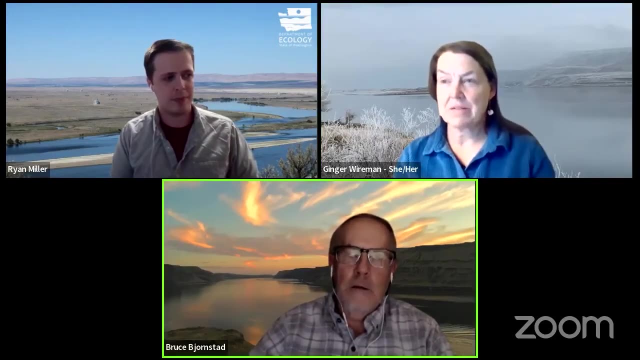 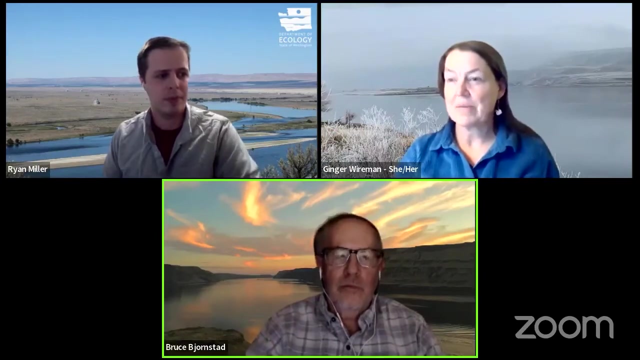 elements, Great um. so we we had a question from Chris um, asking about the formation of rattlesnake, which I think you've covered that a little bit, um, and I think we need to make sure that we're clarifying fault and fold. Fold is where they're and then the faults are the breaks in them. So, Mark Derrick, 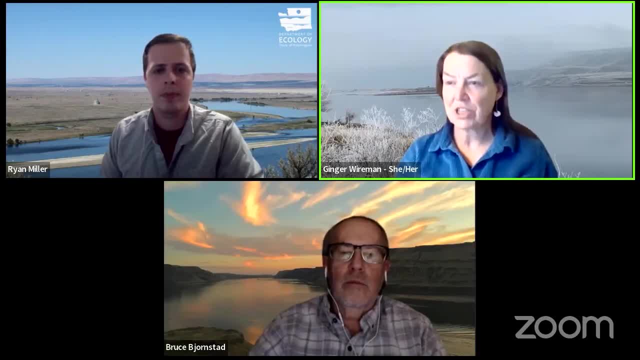 asked: how active are the faults and has that been a factor in the formation of rattlesnake Fault, and has there been any trenching work specifically along rattlesnake mountain, the rattlesnake mountain fault? that tells us just how large the earthquakes are. 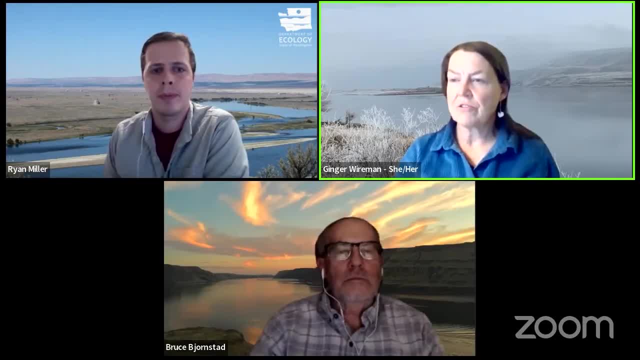 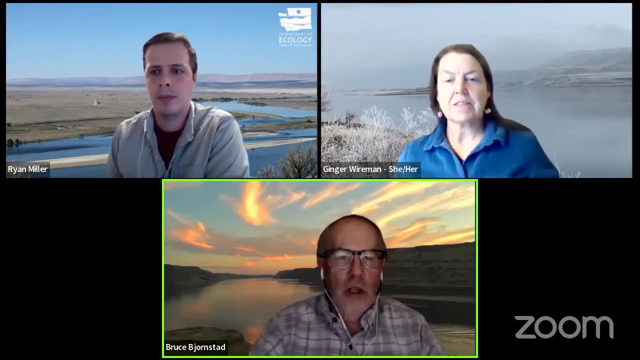 were could be and what the reoccurrence intervals might be. Michael West's from the Colorado School of Mines work suggests earthquakes in excess of 7.0.. Um, yeah, there has been trenching done along those faults. The trouble is they're really, they're- uh, they're low angle thrust faults, which is 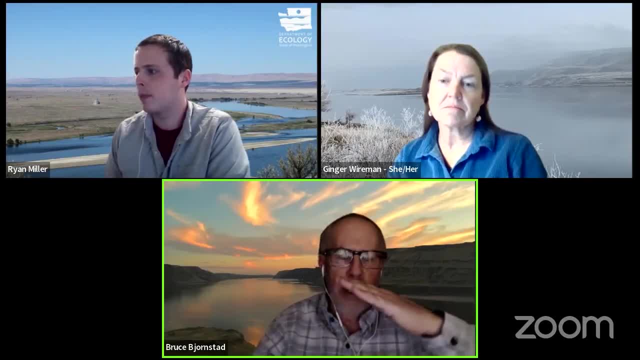 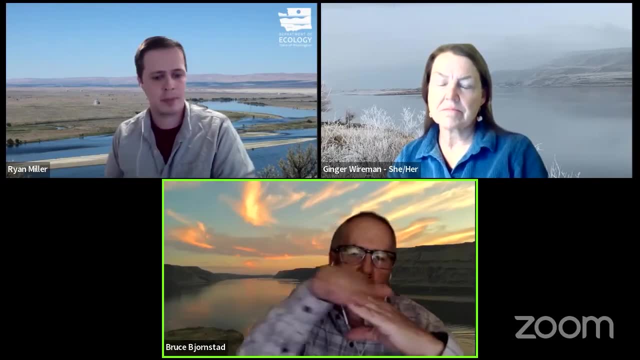 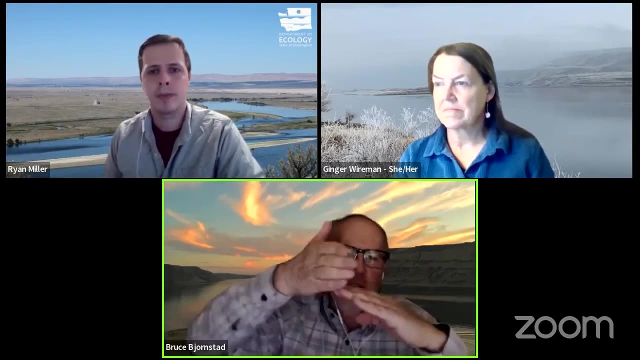 in other words, they're the faults, they're not like this, they're low angle and the uh, this part, the southern part of the fault, um is moving up and over um at fault. So if you, if you trench it's, it's hard to trench, going uh sideways into the, to the mountain when they trench. 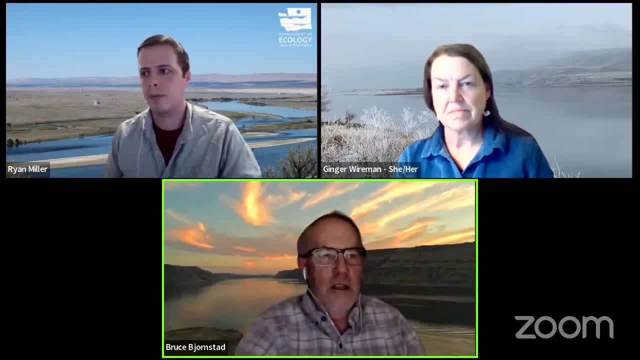 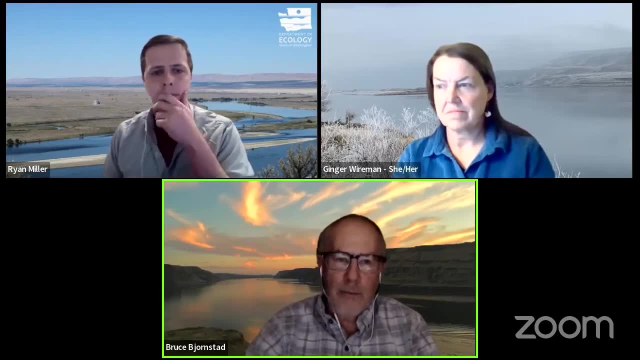 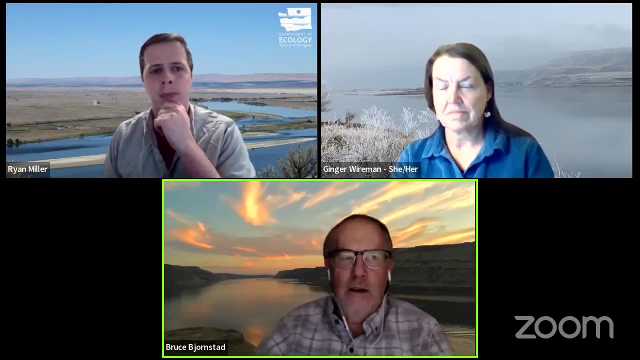 They usually go vertically like this. and so there there have been uh, studies done, trenching done. there's been trenching done, uh, and a little gap along some faulting there. Uh, the trouble with trenching on the Hanford site and on rattlesnake mountain is it's a tribal. 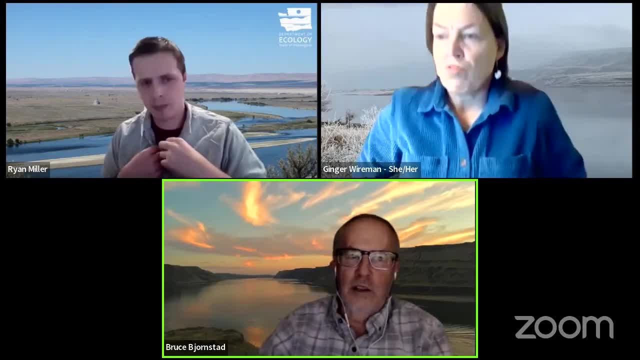 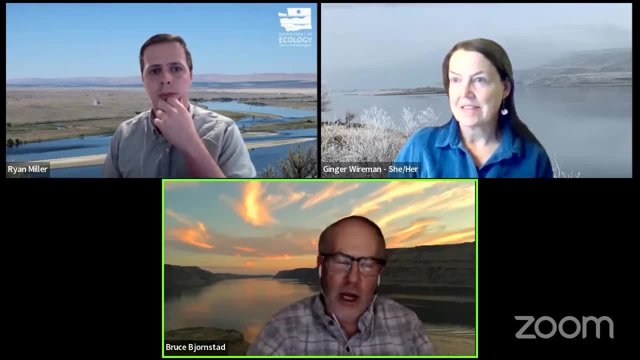 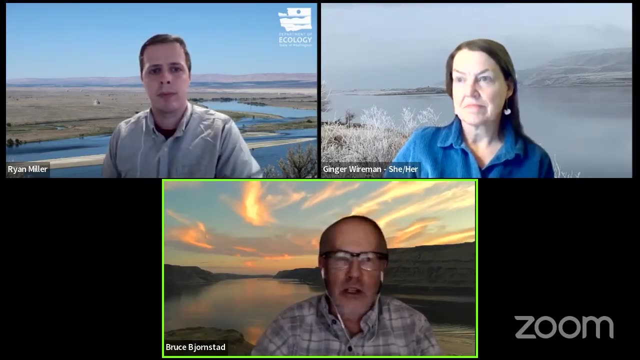 area and the the Native Americans are very sensitive about doing any uh disturbance in that area. So there hasn't been a lot of trenching directly on rattlesnake mountain. but there's been other studies done: AeroMag, uh gravity surveys, lots of other surveys. 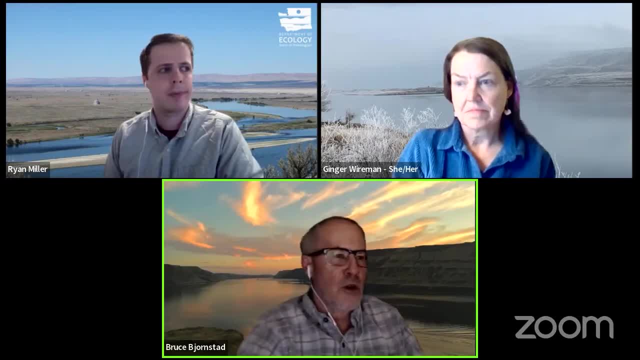 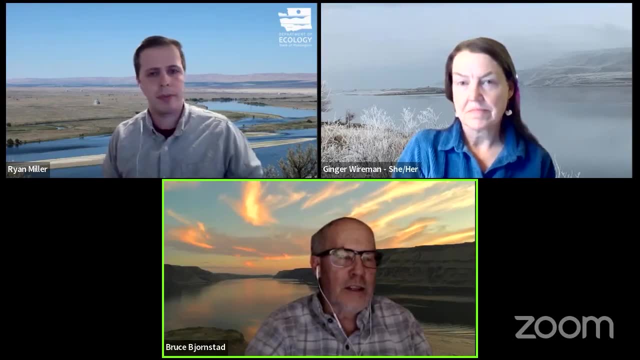 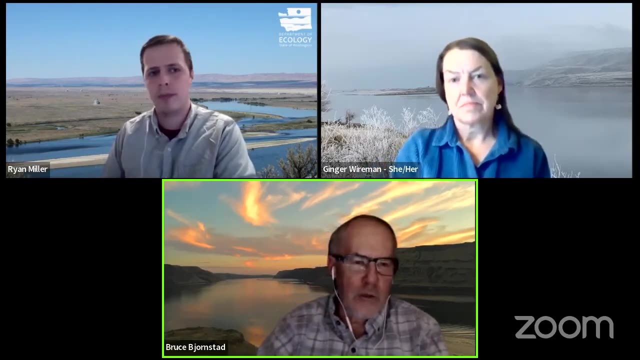 geophysical surveys that have been performed to try to remotely detect these faults And I think the historical earth biggest earthquakes in our area are somewhere around five or six magnitude. five or six. I don't think we've had any going up to seven. uh, because we're for 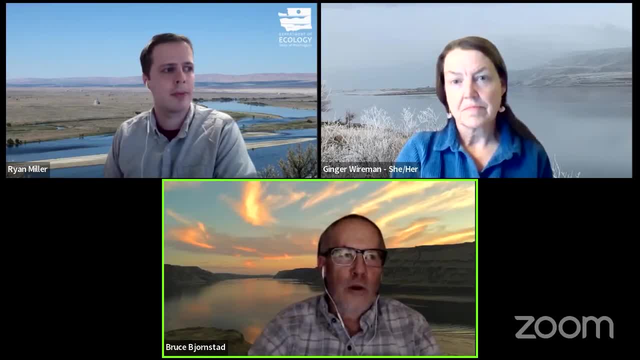 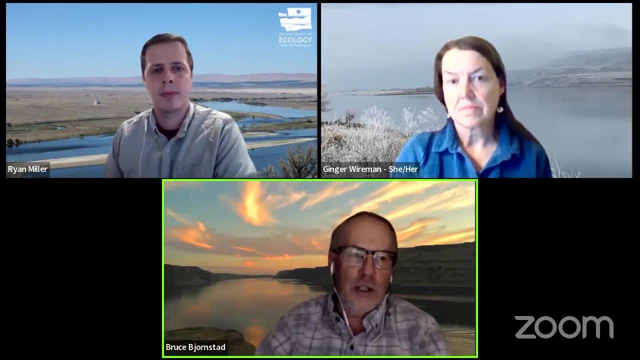 in our area. uh, we're further away from the major subduction going on on the west coast, over by Seattle, off the west coast of Oregon and in Washington, So we don't we're not likely to get as big of earthquakes here as we you'd see associated with these subduction zone earthquakes. 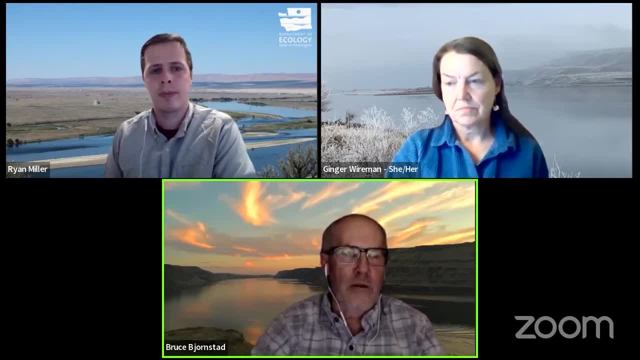 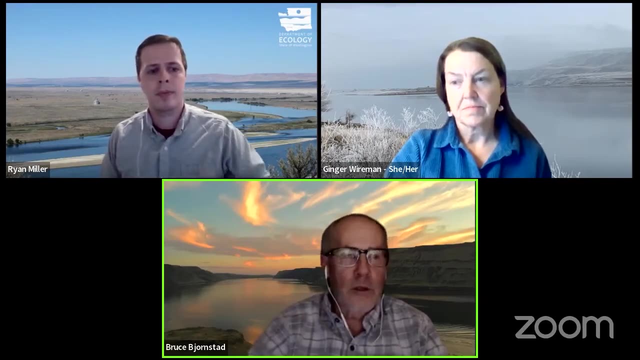 The further. we're quite a ways away from there and if we had any uh faulting uh associated with those, those faults, the subduction faults, they'd be uh, minimized uh this far away in eastern Washington. But we do have faults along these folds, these Yakima faults and uh and that could. 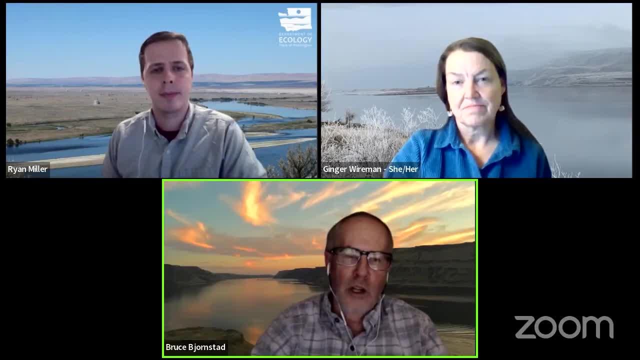 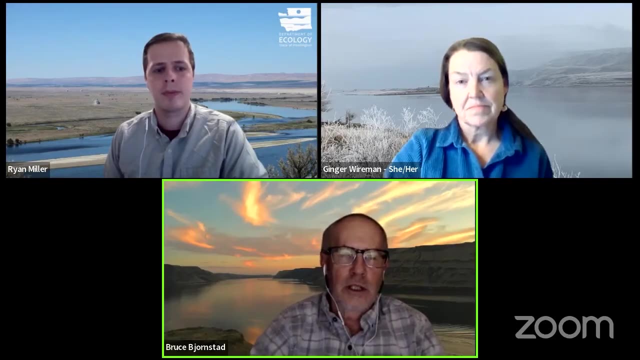 be like: um, those could be the faults that are generating these flies and sexes. There's still a lot of work to be done. it could be done on these, these Yakima folds, and there will be studies done in the future, I'm sure. But it's occurring slowly and it's 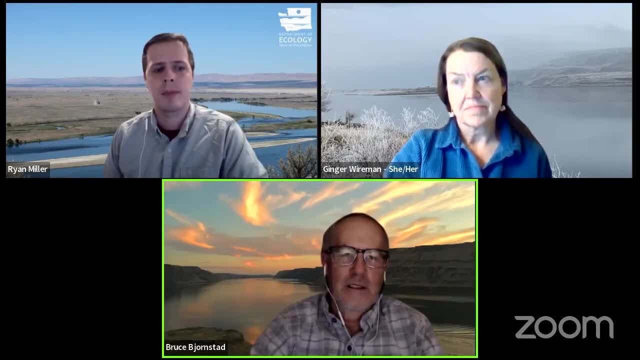 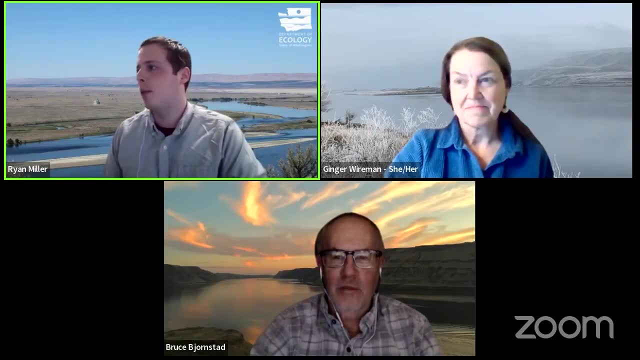 I'm sure it's not fast enough for a lot of people, But it costs money and it takes time, so Awesome. thank you, Bruce. Um, we had a question that I kind of answered in the chat on Facebook, but it'd be good to ask it over over Zoom. 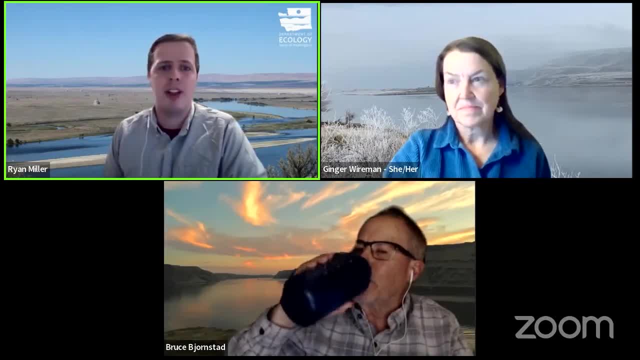 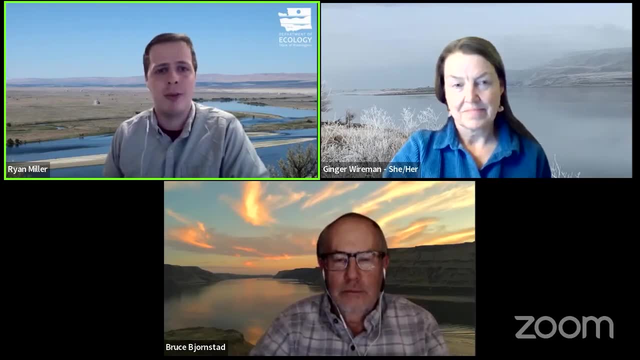 was another question by Susan asking if this presentation is going to be available on the college's website. answer is yes. after last event we put up a little section on the public education page on on our Hanford web pages that shares the presentations from these events. we're going to 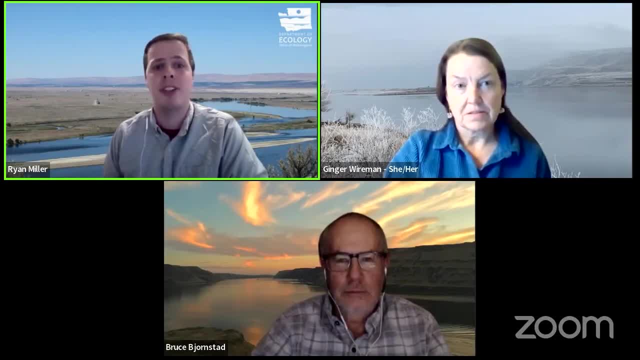 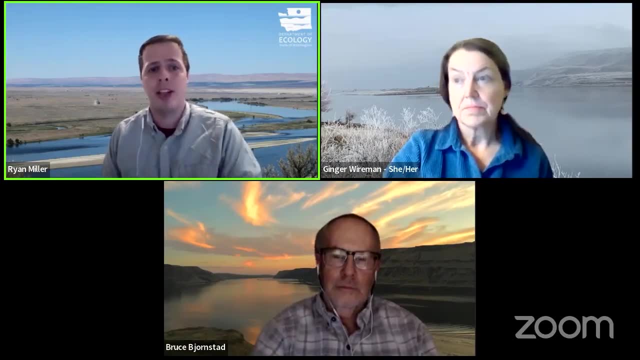 be sending out a social media post after this event, one that gets posted. so we will put the slides up there, probably in the next day or so, and we'll get that that put up and we'll share the link on social media and we'll probably send out an email list, like we did the last go around. 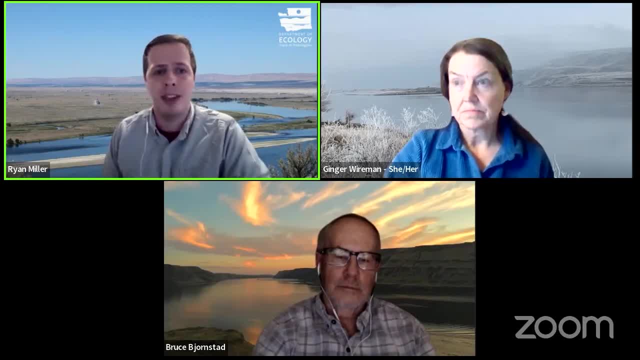 and and before we go into another live question, I thought we could skip over and start knocking out some of the pre-submitted questions too. so we had a couple questions asked from Philip over over email before this event started and, Bruce, I know you kind of covered this in your presentation. 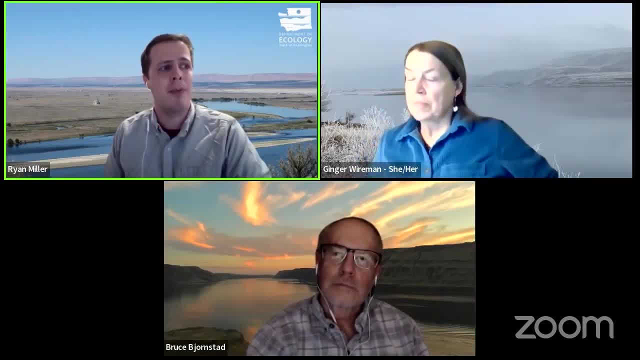 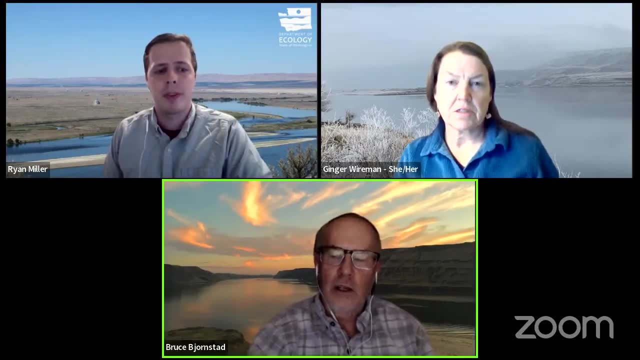 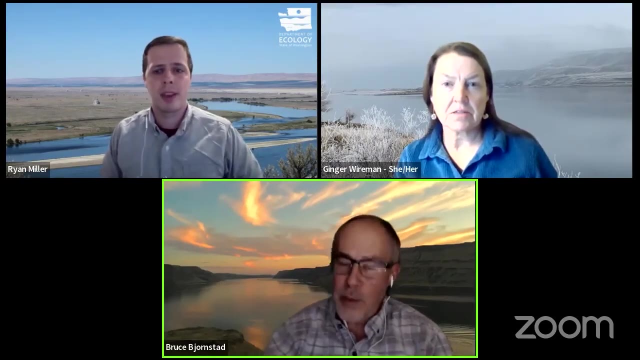 Philip asked: how was the sentinel gap formed? I'm I guess if you have any other thoughts to add to that from your presentation. do you have anything else you want to add on that topic? okay, that's, that's a good question. we have several gaps: the sentinel gap, the lilla gap, uh, Frenchman gap. these are all places where the Columbia river cuts. 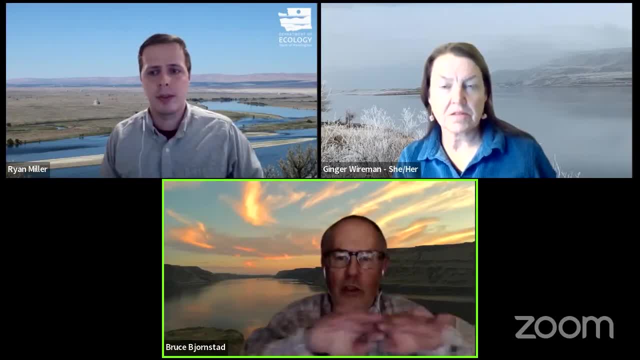 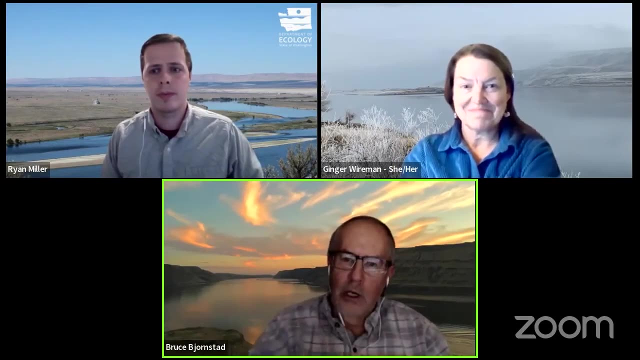 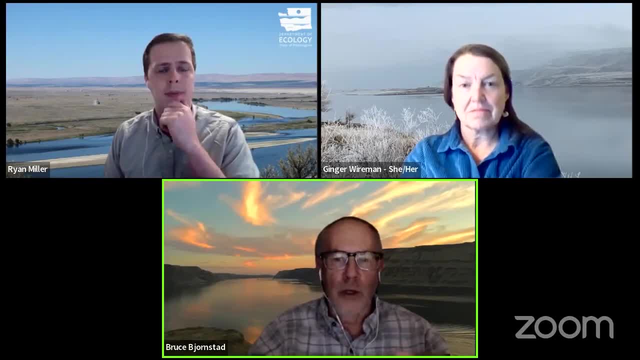 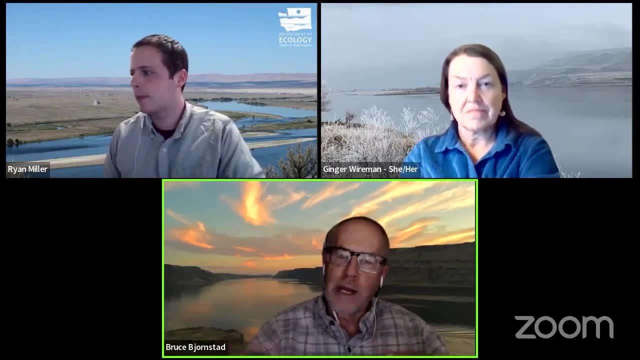 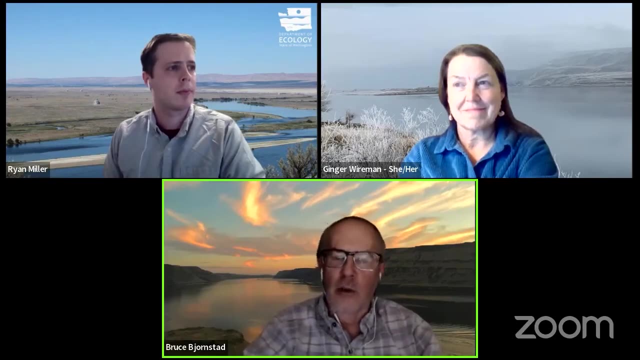 they were growing very slowly. over a long period of time, million, ten, you know, 10 or 12 million years these ridges have been. they've been growing, but the river has been able to keep up. as the as the ridges have slowly rise, the river's been able to maintain its channel through those, through those. 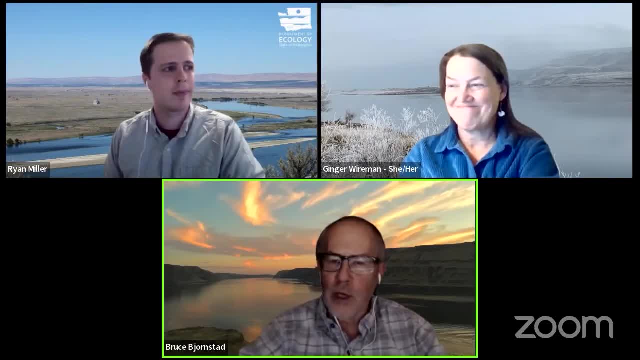 ridges. so the sentinel gap is just one. it's one of many water gaps where the Columbia river has been able to keep up with the tectonic uh up folding of these ridges. so that's one of the many water gaps where the Columbia river has been able to keep up with the tectonic. 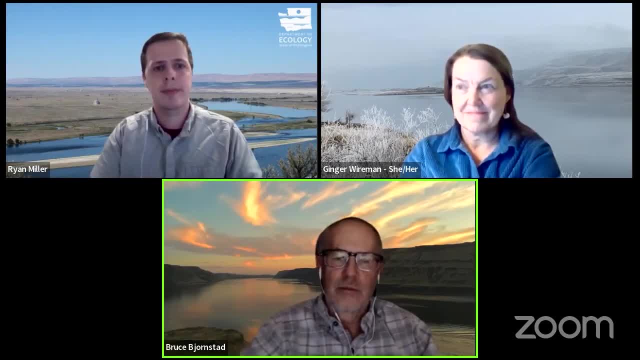 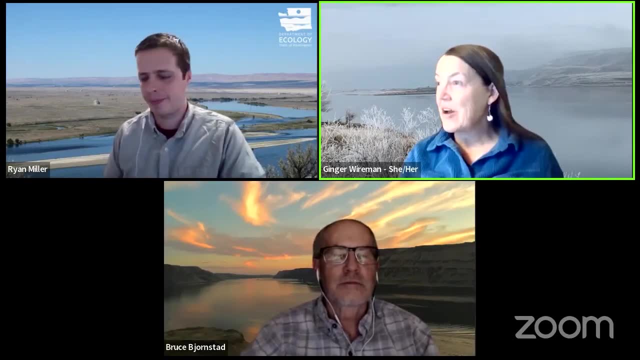 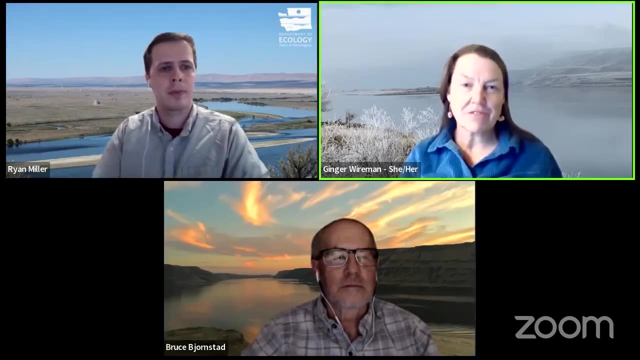 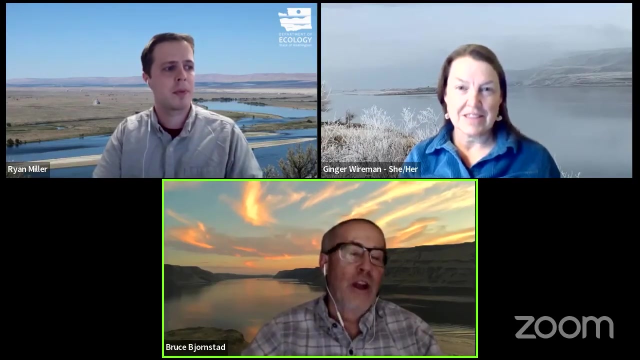 up folding of these ridges. let's see, did you? let's see? um, oh, how about how many? this is another one from phil. how many distinct Columbia river channels cross the Hanford reservation? well, there's, besides the one that where the river is now, there's been one other major uh channel where the Columbia river used. 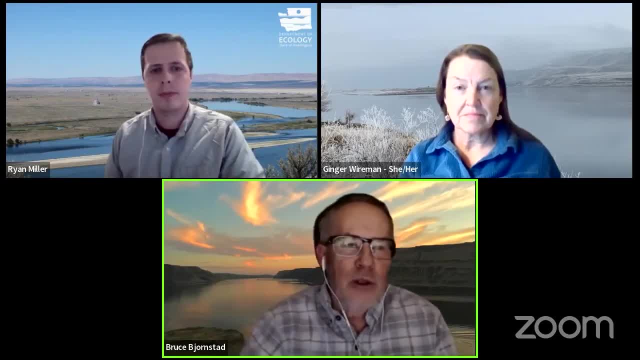 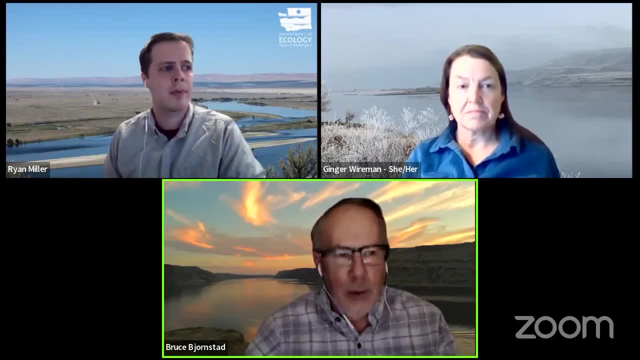 to go and that was through, uh, Gable Gantt and the Columbia river used to go through the Columbia river which is on the Hanford site. it's kind of in the middle of the Hanford site. we have Gable mountain and Gable butte and in between we have a channel. 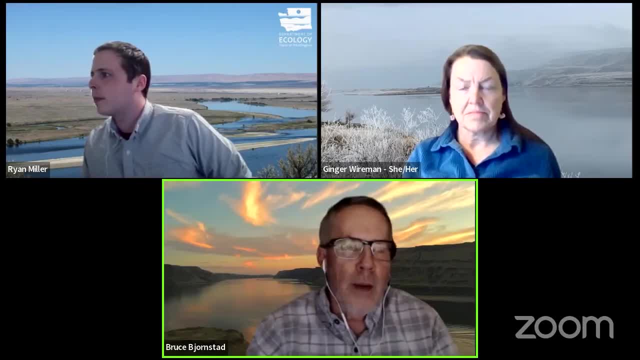 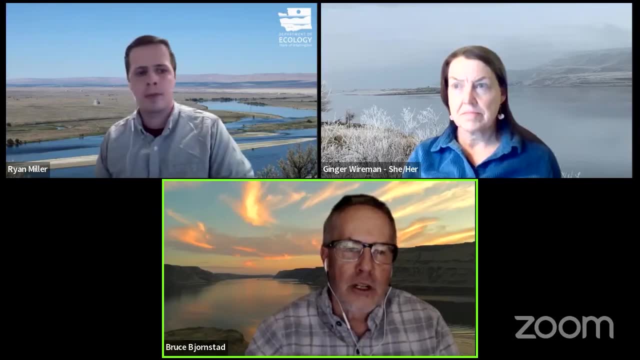 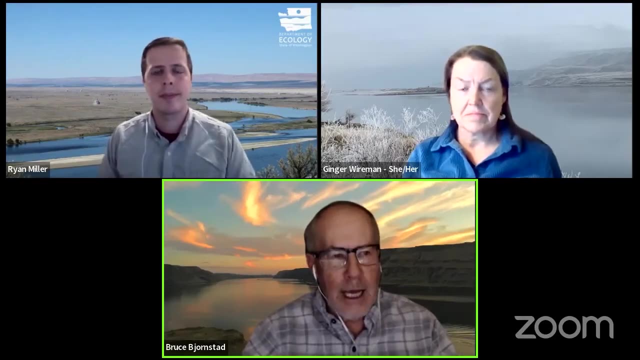 that was cut by the Columbia river and we know that by looking at the boreholes and sediments uh that are in the gap that are uh characteristic of the Columbia river. so that was from there and the river did cut through uh Gable gap and then it kind of hit its. 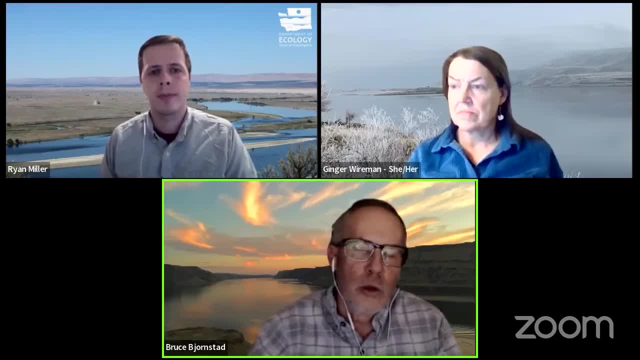 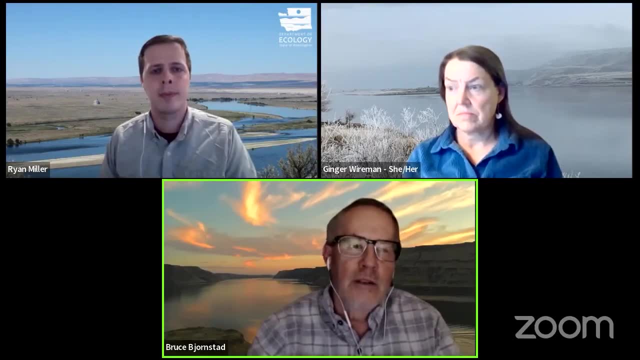 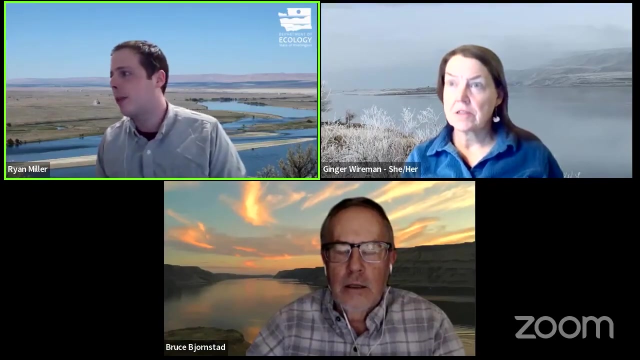 and west, kind of parallel, so to where it runs today, but it was probably a few miles west of where it is today and it's it's buried now. it's buried under, you know, these all these younger sediments that came in later. awesome thanks, bruce. uh, next question comes from facebook, and this one is from: 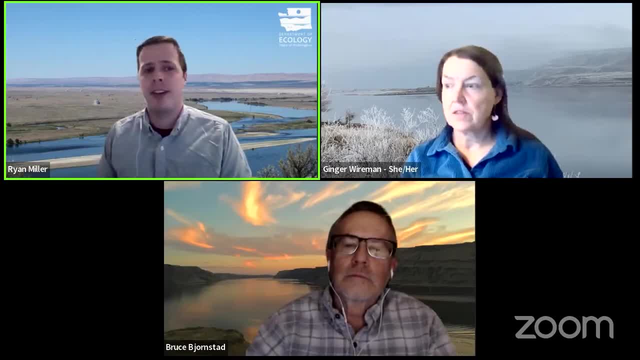 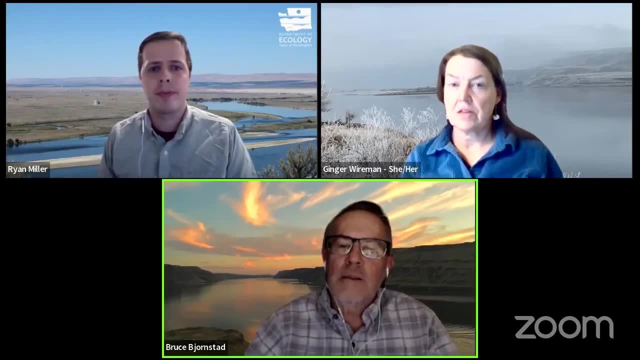 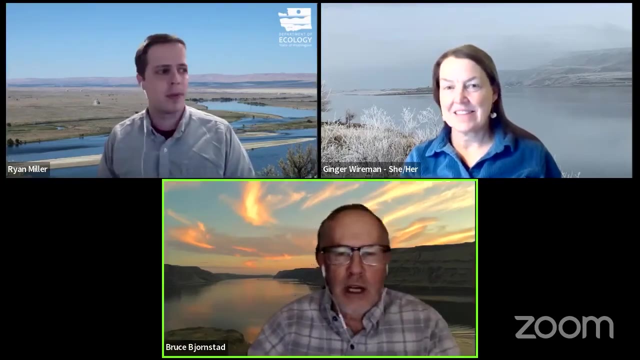 uh, leela leila, apologize if i mess up your name. this question was so: will the yakima folds continue to fold further? will the yakima folds continue to fold further? yes, definitely. uh, it's. they've been going on. this has been going on for um at least 12 million, 17 million years. 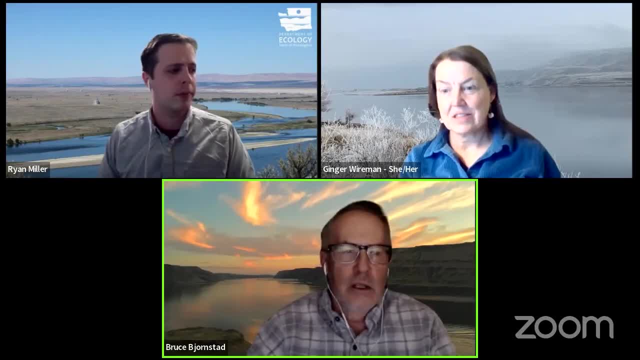 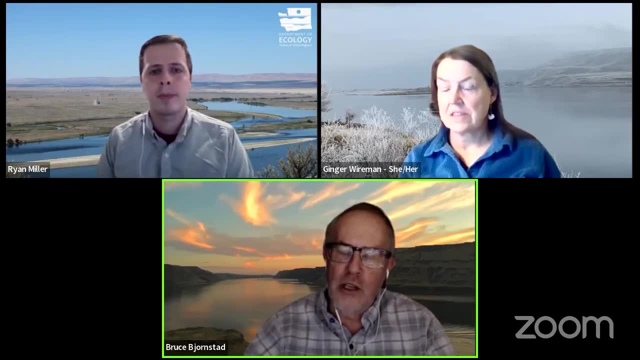 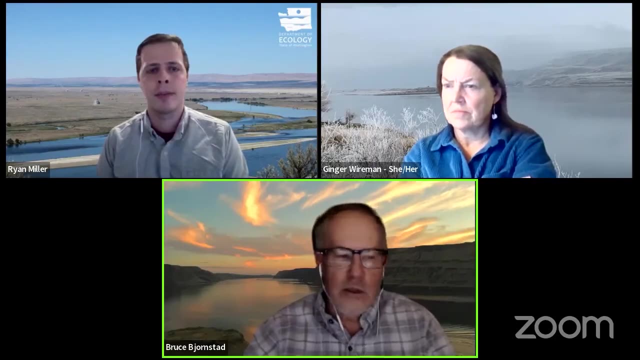 and the chances are of it continuing, uh, or high, especially continuing, or high, especially continuing, or high especially continuing, considering we, we're, we're continuing to have this tectonic rotation of of eastern washington and as long as that keeps rotating, uh, there's, there's gonna the 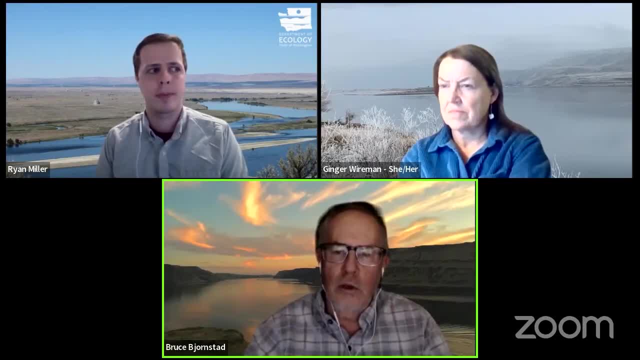 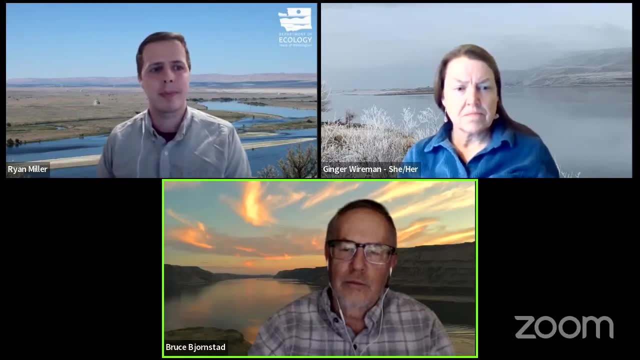 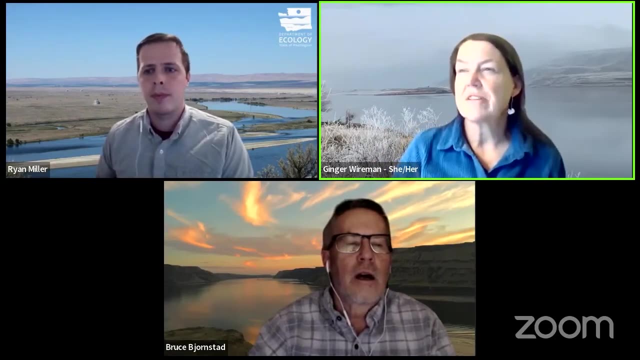 stress is still there to create and to continue, force these folds to continue to keep growing. um, gerald, you're. yoka asked how far back can we trace the, the continental hotspot that moved east to its current location, and was it close to Hanford? Well the Yellowstone hotspot is actually. it's migrated from where it is now. It used to be down in Southern Oregon, Northern California. That's where it was about, I think around 30 or 40 million years ago. The Yellowstone hotspot was under that area. 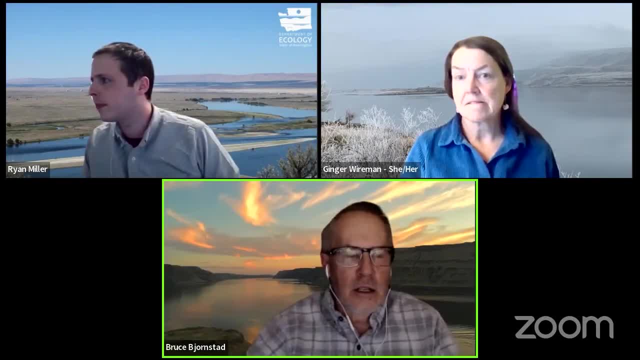 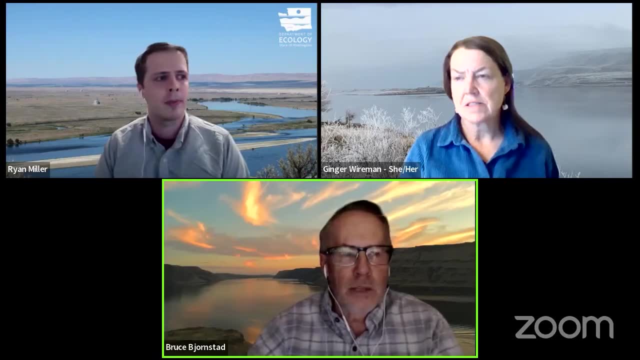 but because of tectonic rotation, the Earth's crust, the North American plate, is rotated and the hotspot has moved. As the North American plate moved, it migrated from Southern Oregon to Wyoming, Eastern Idaho and Wyoming where it is today. 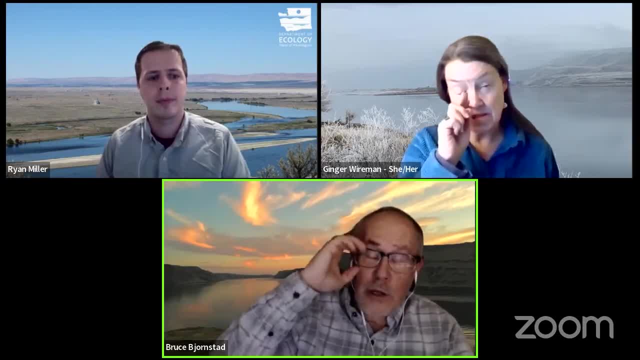 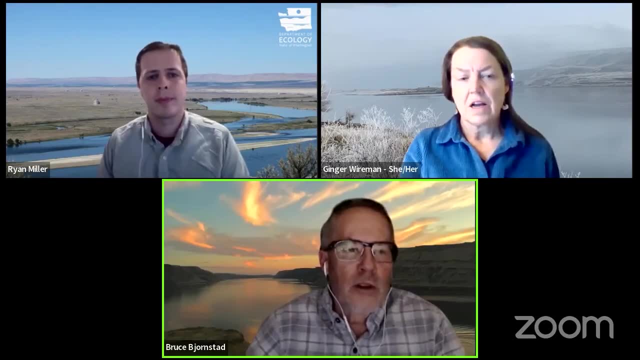 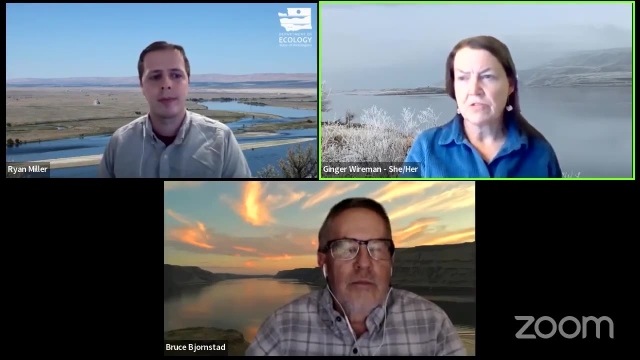 So, yes, But it was never. the Yellowstone hotspot was never directly in Hanford or Washington, but it was much further south than Washington. I'm going to jump in and do a follow-up, because we were talking about this rotation. Jeanette, do we feel the clockwise rotational movements? 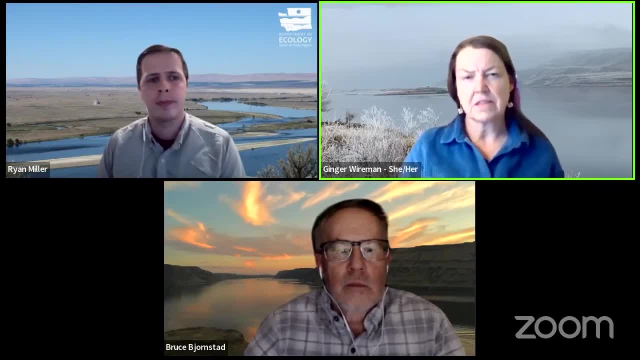 that are measured via GPS, Like. is that something? is that picked up, I guess, by like size, By seismic machines, or how do you know? No, not really. How do you know what's happening? There's no seismic, it's not tied to the seismicity. 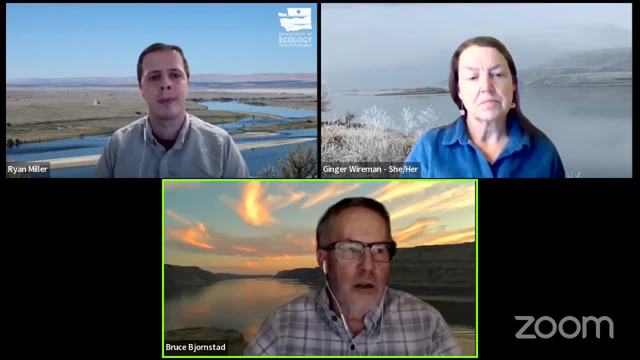 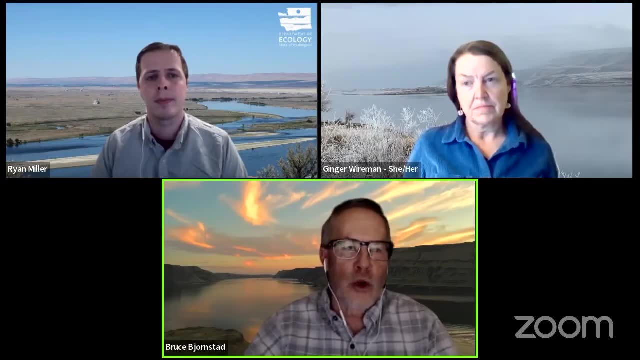 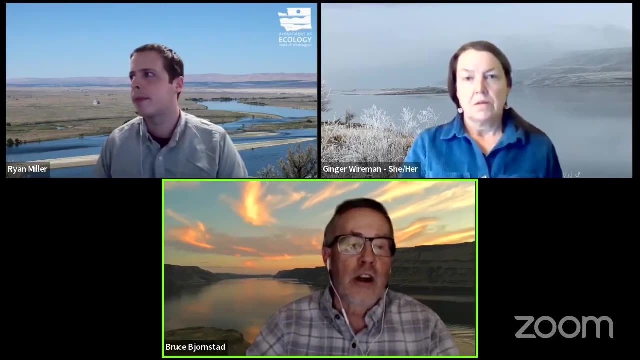 These GPS units when they they've got hundreds of these spread out across the Pacific Northwest And what they do is they're recording their location And their location is migrating, is changing over time. So in one year, because they're highly precise. 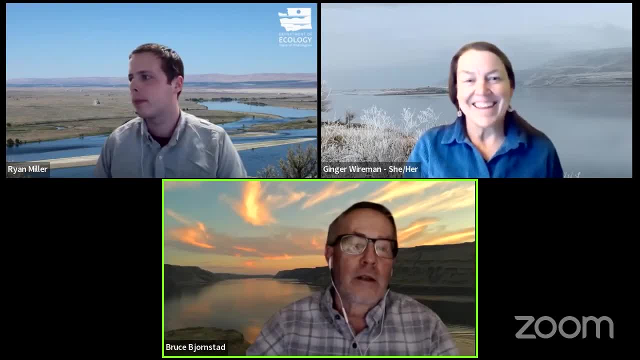 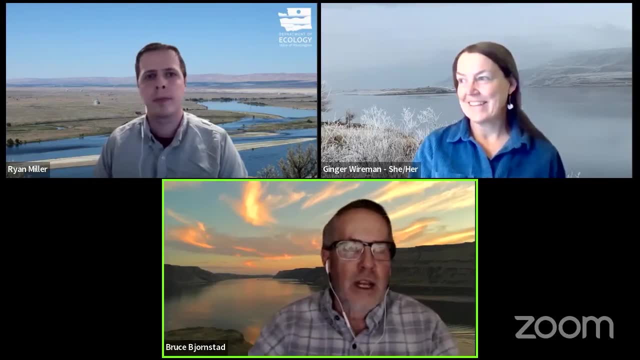 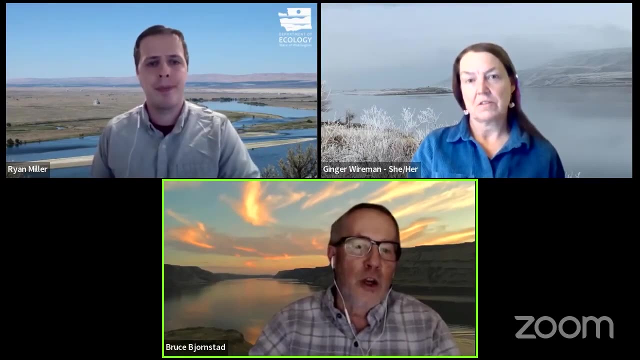 they can measure 20 millimeters of movement in one year over time. And then each one of these, and they're in that most, the most amount of movement is going on in Western Oregon and Washington And under Pendleton we have. 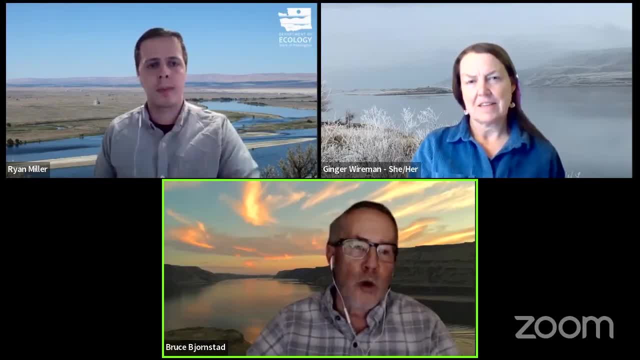 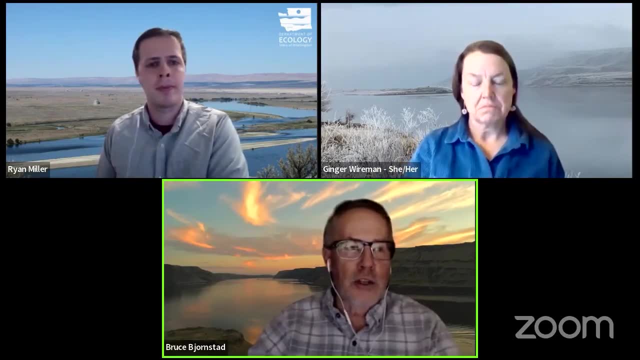 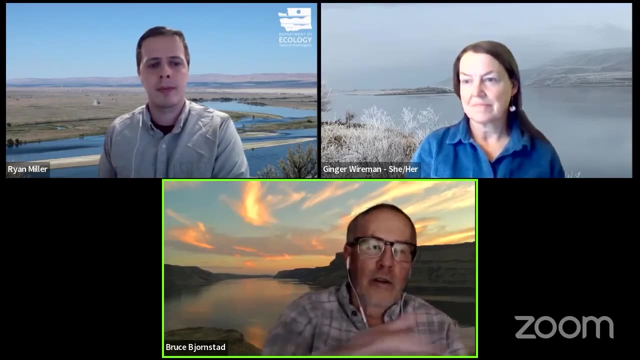 they have the same GPS units and there's no movement because it's at the focal point for the rotation And in Eastern Washington, Eastern Washington, there's not as much motion either, because it's closer to that pivot point, The further, further away from the pivot point you get. 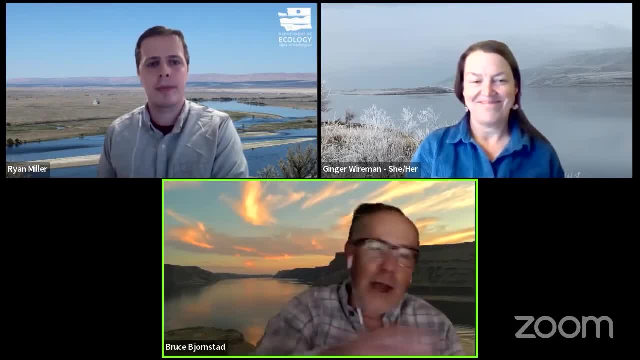 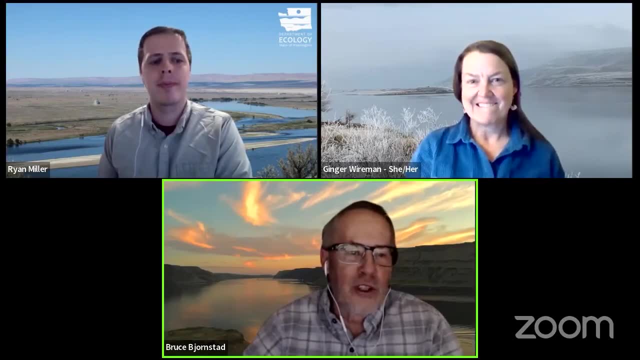 the more rotation you're going to see because of angular momentum and all that stuff. So and so, yeah, we don't feel, we will never feel or detect any motion in our. you know, humans are not able to detect that small amount. 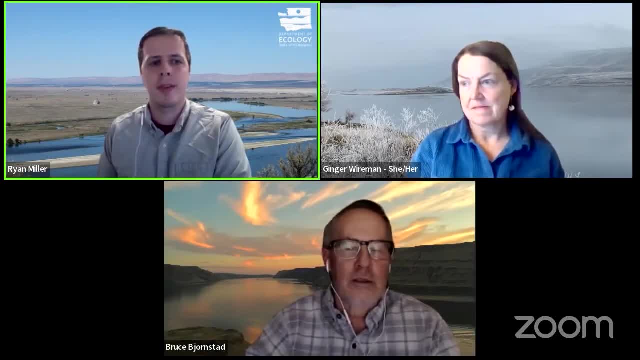 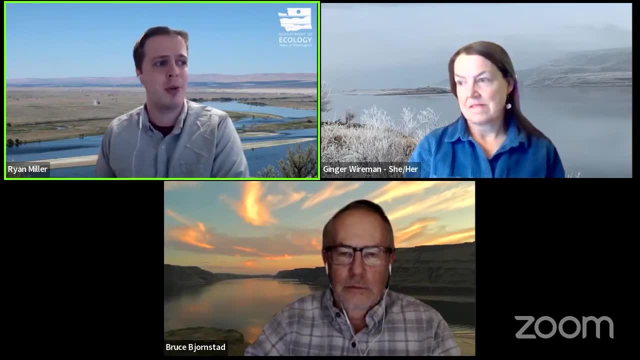 They're not able to detect that small amount of motion, but these GPS sensors can and they do. Perfect Thanks, Bruce. I have a couple of questions on Facebook. This first one comes from Teresa and Teresa asked: is Idaho affected by the rotation? 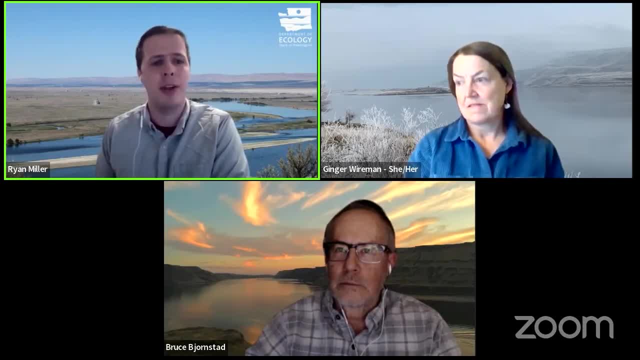 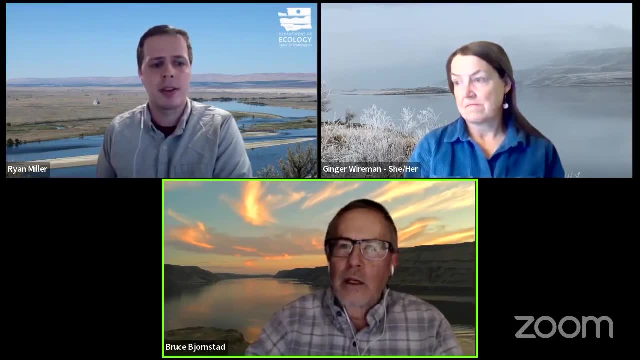 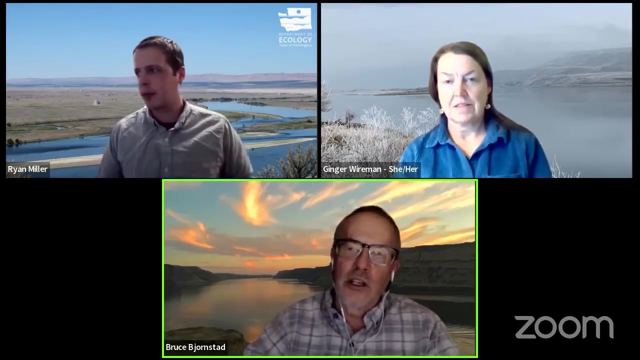 And this was asked back around the slides involving Ringold- And it might've been the slide right before the Ringold formation slide- Is Idaho affected by the rotation? It is by the fact that the Yellowstone hotspot is migrated underneath Idaho and then to Wyoming. 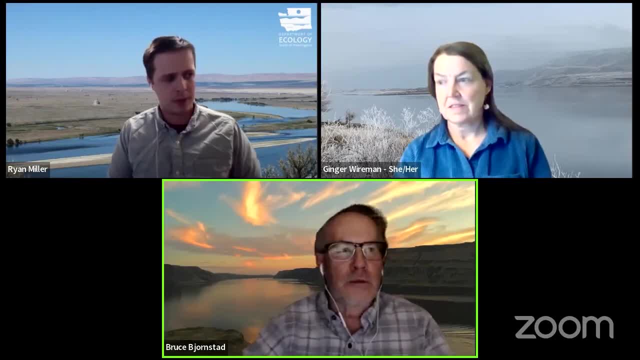 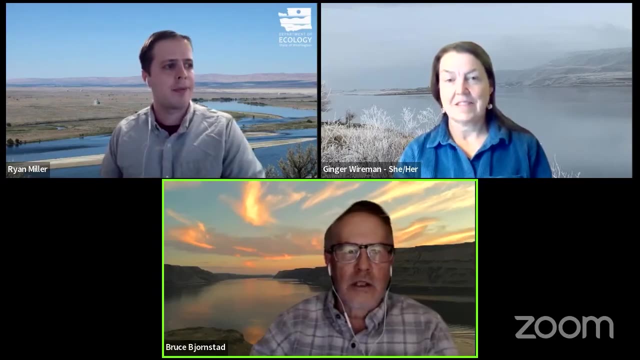 where it is today. So it has been involved, but it's mainly Southern Idaho. I think Northern Idaho may be more fixed in its position and maybe not moving as much, but Southern Idaho is definitely is part of the story of rotation. Awesome Thanks, Bruce. 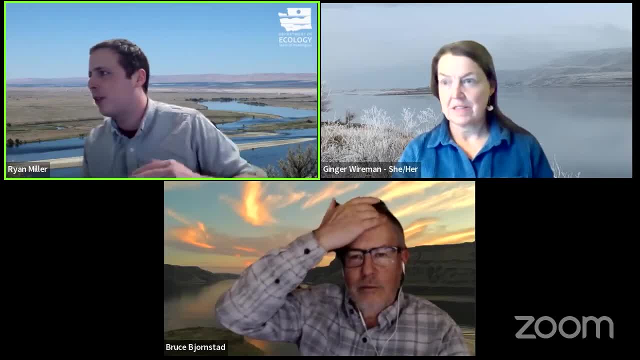 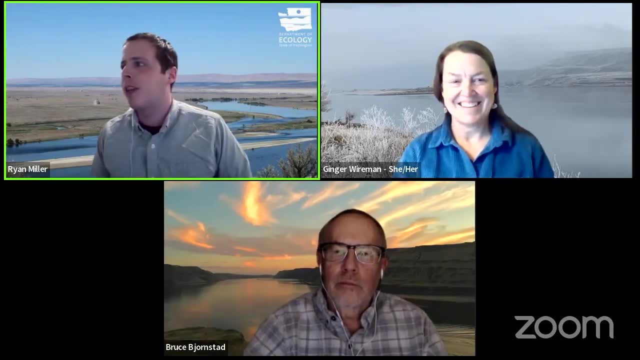 We've got. I'm just going back up to the next question. Make sure we're going a little in order here. This one comes from Susan Lechband again, And Susan asked: have any precious metals ever been discovered at Hanford? 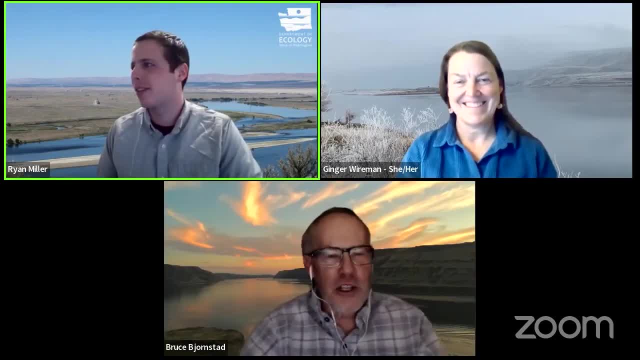 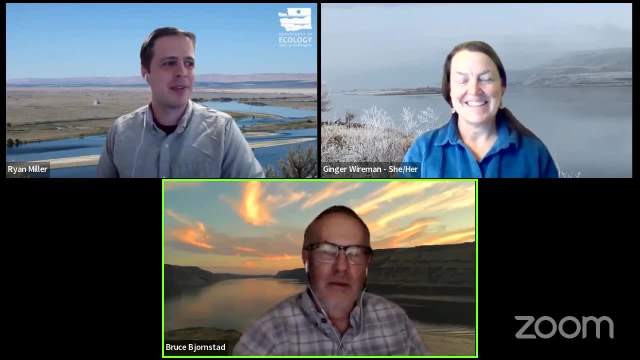 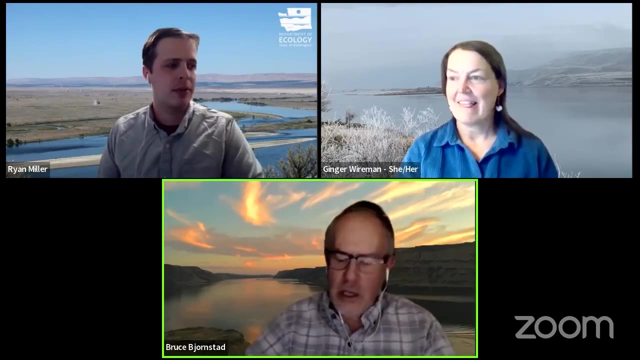 Not yet. There's a lot of metal associated with contents of the tanks, The you know the underground storage tanks at Hanford. I know they're. I think them were in a liquid form. but as far as the you know the Ringold formation. 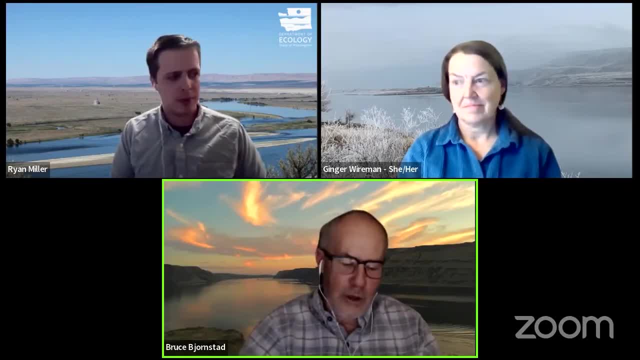 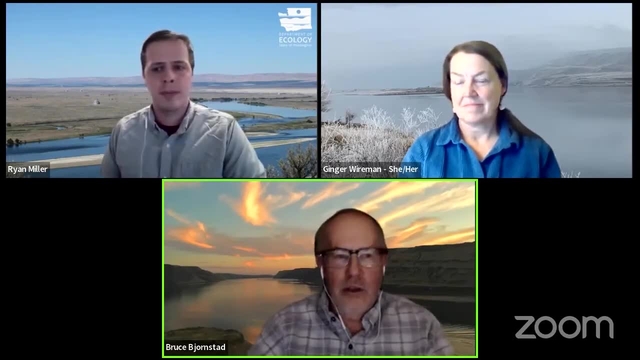 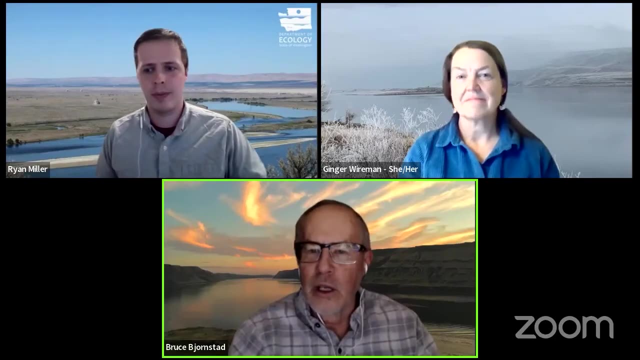 that the salt Ringold Hanford? they're not. they're very rare, They're very. they have trace metals, trace amounts of metals associated with the sediments that are in them, but they'll never be of economic value because they're not concentrated enough. 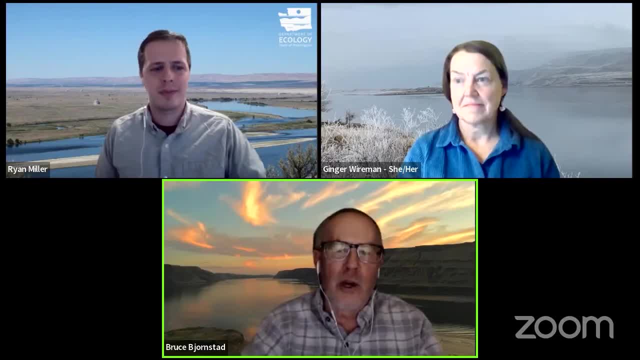 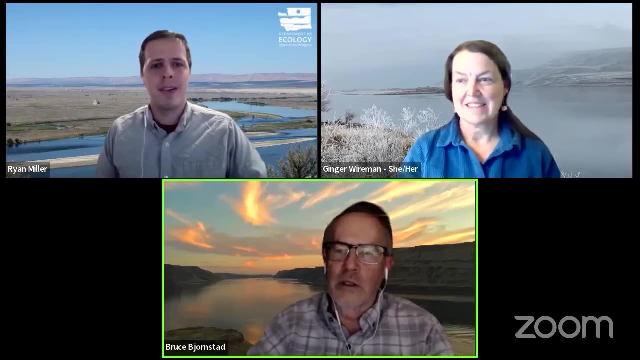 They're very. Bruce D Potter Various my new quantity quantities and precious metals that are within those deposits. so and the salt is is very, is really not Bruce D Potter A very. it's not economically valuable. Bruce D Potter As a as a resource. 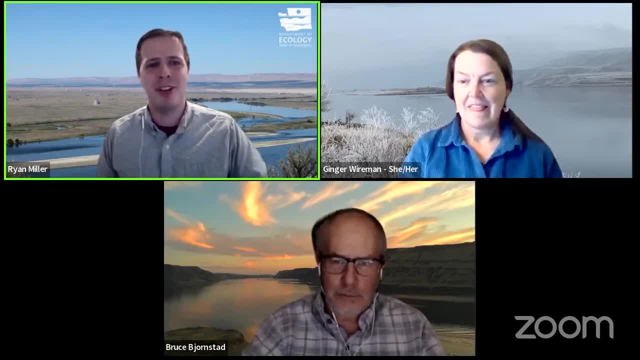 Bruce D Potter. Thanks, Bruce, and I don't know. I want to consider this: natural metals and apparently back. you know, decades ago somebody robbed the white bluffs bank and made off somewhere between hampered and and when actually, and then they're shot before they were covered the treasure. so there might be some treasure buried. 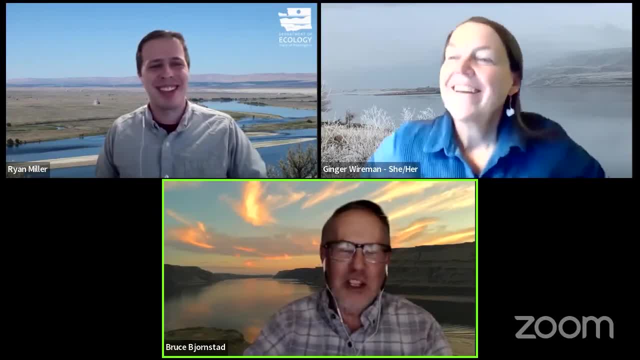 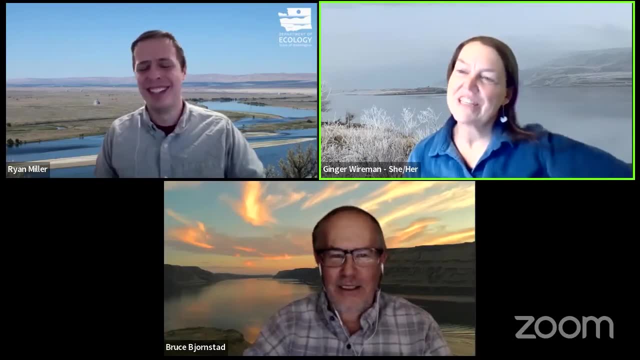 Bruce D Potter. Okay well, Bruce D Potter. yeah, that may still be out there. hi, Bruce D Potter, Good luck. good luck finding it, Amy Dalsimer. All right, well, we have a question that came from mark Derek. 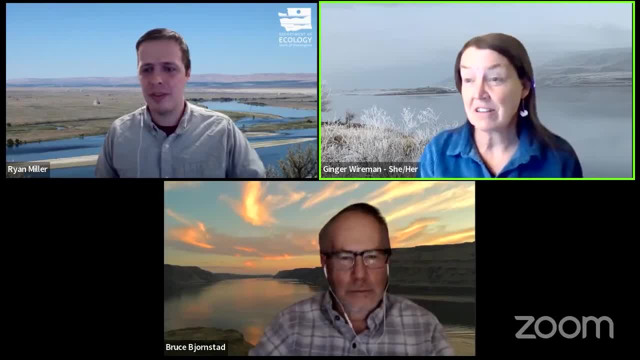 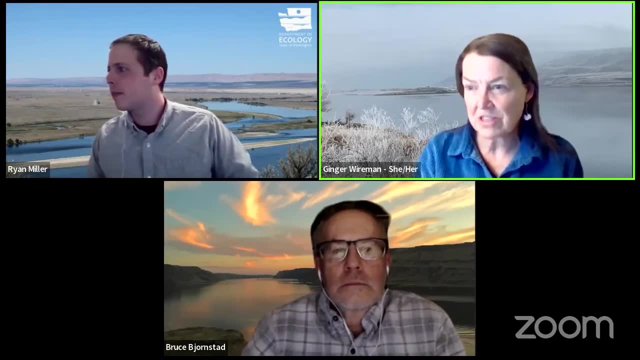 Amy Dalsimer, There are, on zoom, many neo tectonics. geologists would argue that the faults along rattlesnake- and i'm tan of bridge are truly very dangerous. why have there not been more studies? or why have studies? 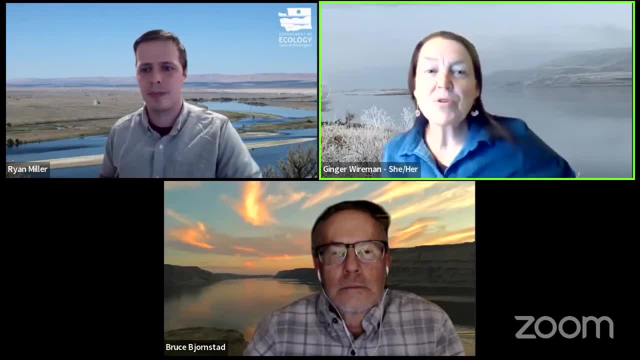 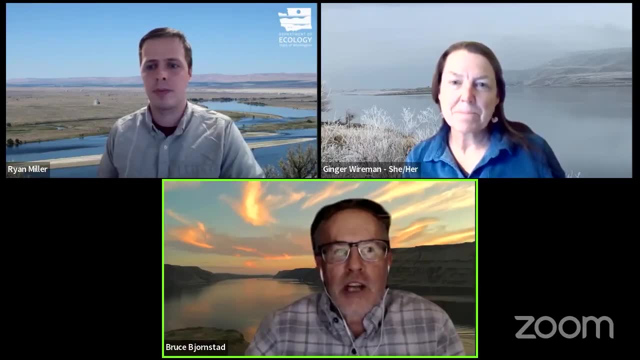 Amy Dalsimer- i'm sorry who I? have the studies not been studied more seriously? there we go thoroughly. maybe Bruce D Potter? Well, we have. we have a record seismicity going back 100 years- Bruce D Potter or so- and 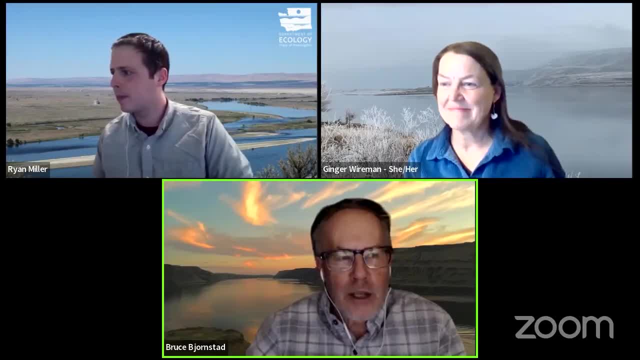 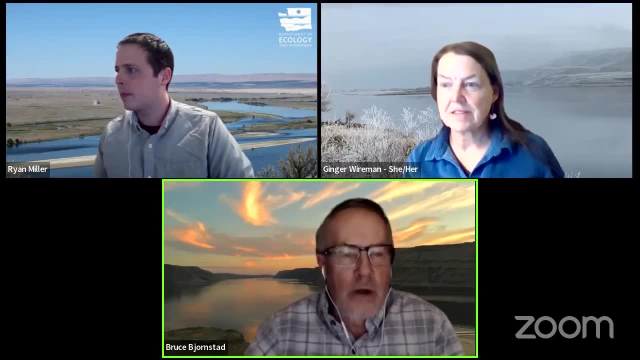 Bruce D Potter. There there have been no bigger quacks on at hanford. there was one down in Bruce D Potter, The Milton, your Milton free water Bruce D Potter East of here. there was one over in the cascades. 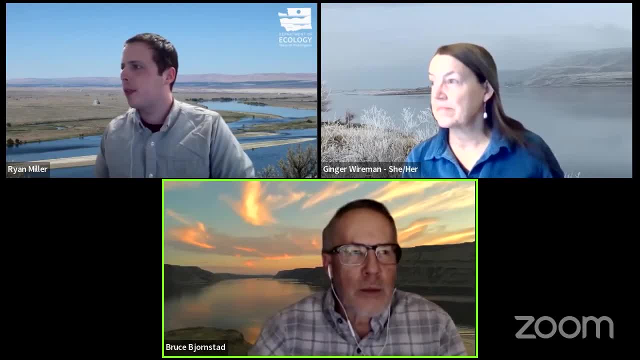 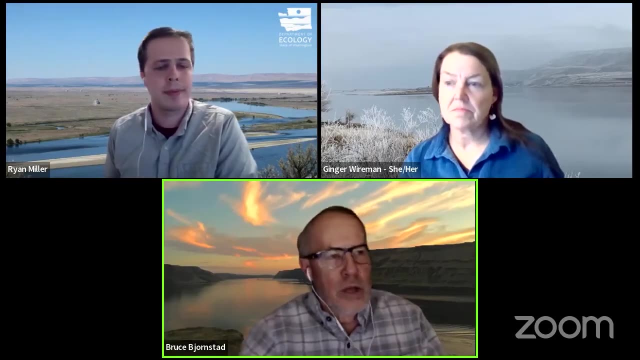 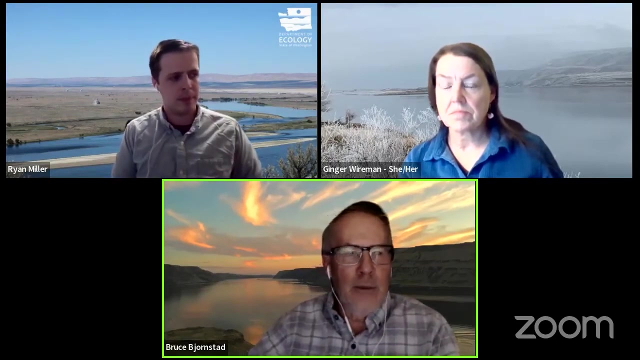 Bruce D Potter Near when atchi that I think maybe went up to like maybe six or seven Bruce D Potter But Bruce D Potter Locally Bruce D Potter, there's Bruce D Potter And they've looked at records but people have made over the years- people living here hundred years ago you know reported may have reported some shaking going on and they've been able to estimate how, how big those earthquakes were by. 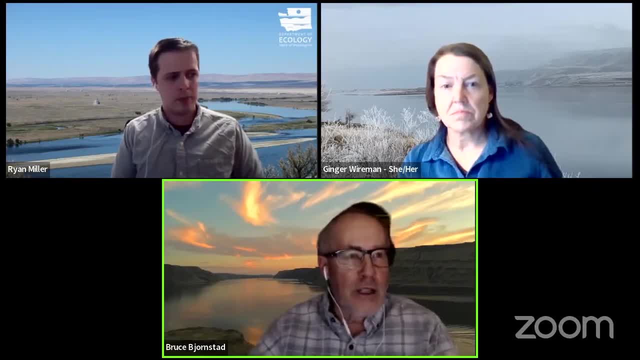 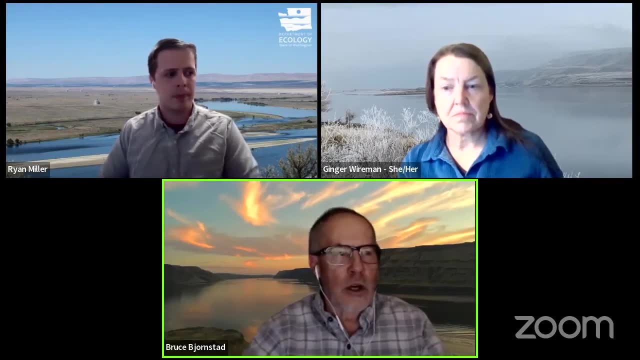 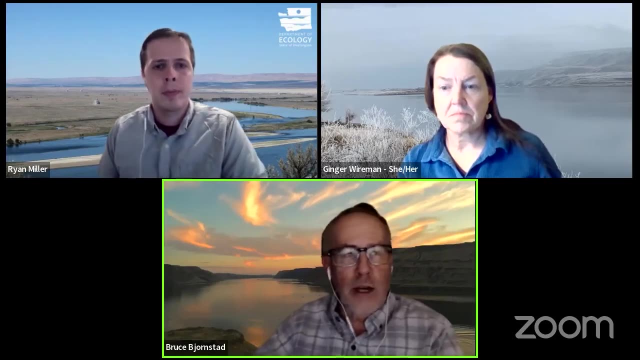 Bruce D Potter By the, by the number of people that reported it and where they were. they were located, Bruce D Potter, And there have been no major earthquakes. Bruce D Potter To would cause serious damage yet, but then it doesn't mean there won't be any in the future. but based on the last hundred years record, there's been no majors, no major earthquakes. 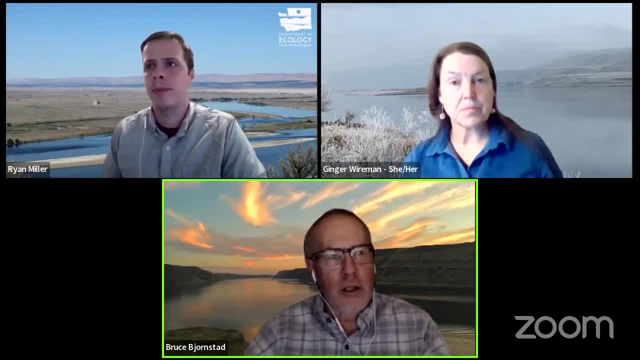 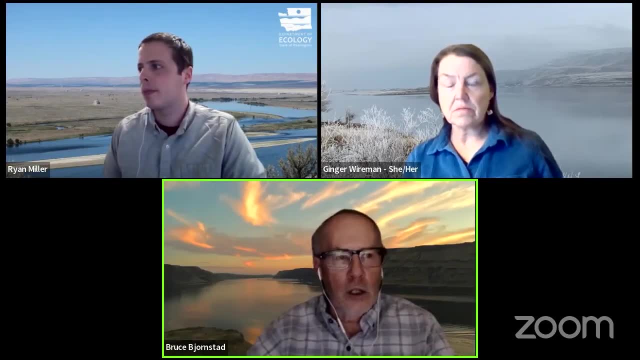 Bruce D Potter In this area, and the further away you are from the earthquake, the less damaging it is. so, and there have been no major earthquakes recorded in close by to the to the head for tonight yet. but it doesn't mean it won't happen. 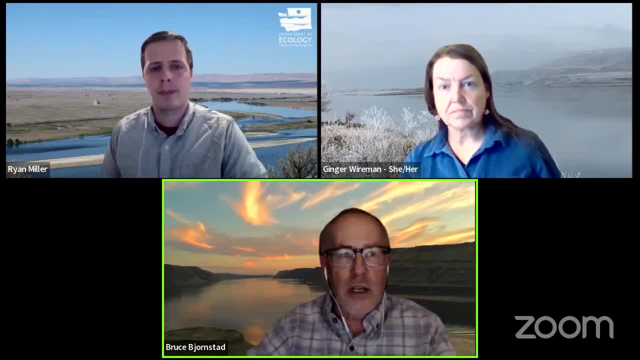 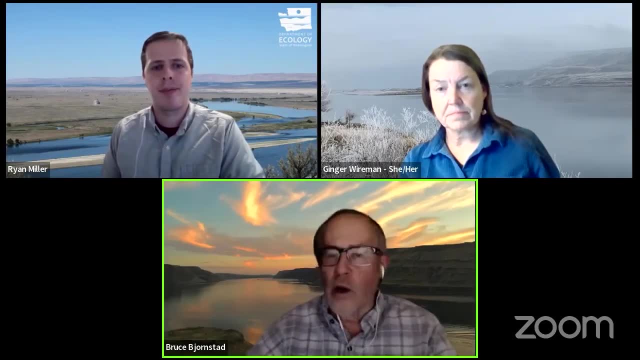 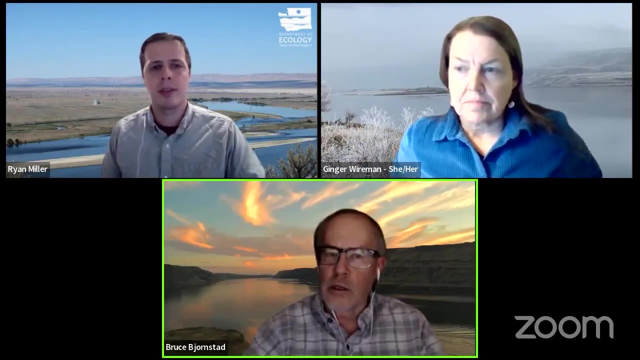 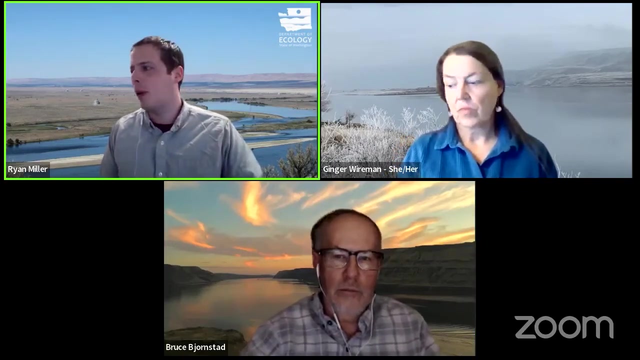 Bruce D Potter In the future. Bruce D Potter And seismologists are studying these structures that are generating earthquakes and so far I have not heard about any alarm being alarm or imminent huge earthquakes occurring in our immediate area. Bruce D Potter- awesome, Thank you, Bruce. one quick question that I can jump in before we do. another geology question was this: 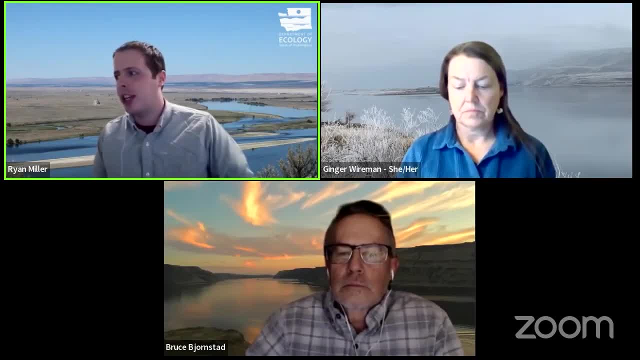 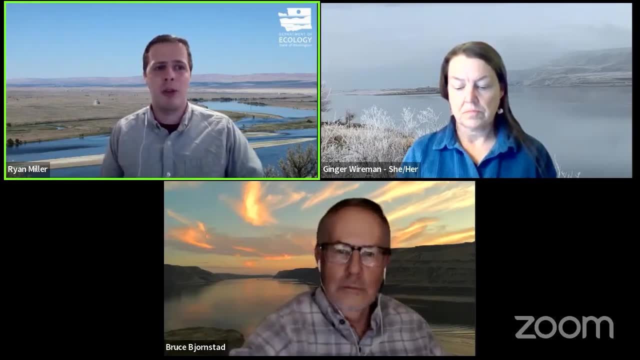 Bruce D Potter comes from. Bruce D Potter. Inga Bruce D Potter On Facebook Bruce D Potter And asked any chance this presentation will be recorded for rewatch? yes, the immediately after the event Bruce D Potter. This recording will buffer a little bit on Facebook and then you can watch the recording on Facebook and that'll be both on our 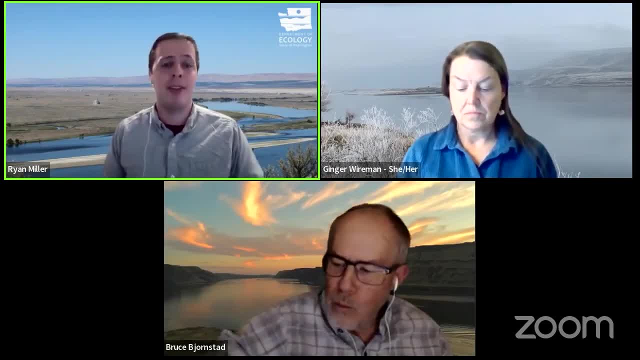 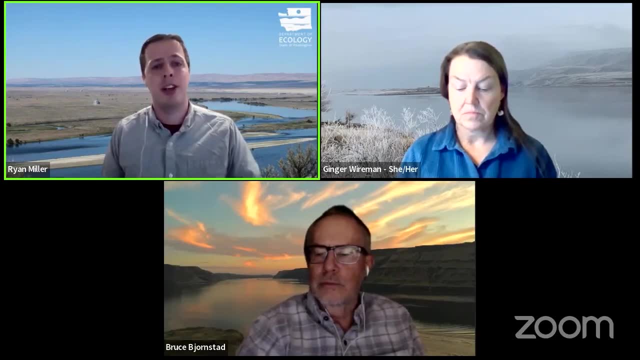 Bruce D Potter, Washington department of ecology handbook Facebook page and also be on the event page for this, for the for tonight's event and also tomorrow. i'm going to go and upload this to the ecology YouTube channel so you can watch it on the ecology YouTube as well. 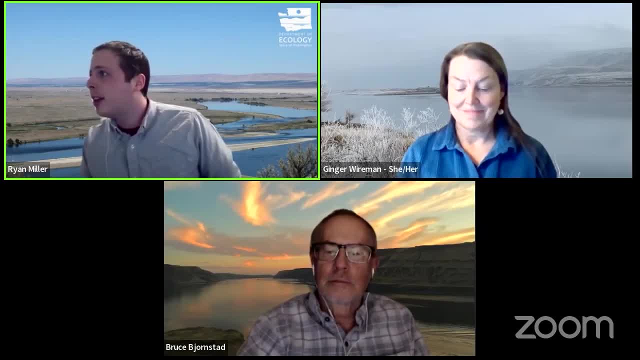 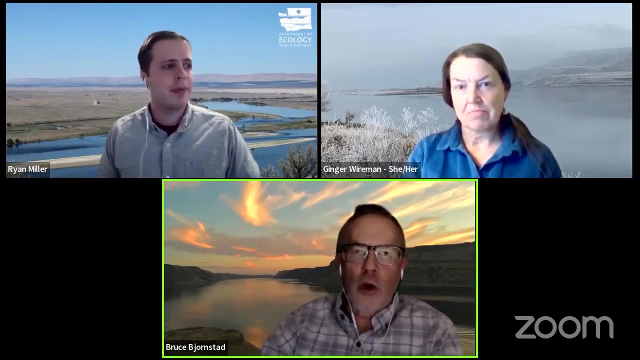 Bruce D Potter And Bruce. we have a question from Bruce D Potter A wind Campbell on Facebook and wind asks: are the sand dunes accessible to the public or are they only on the hampered site itself? Bruce D Potter, um well, the sand dunes I showed in the video, those are. 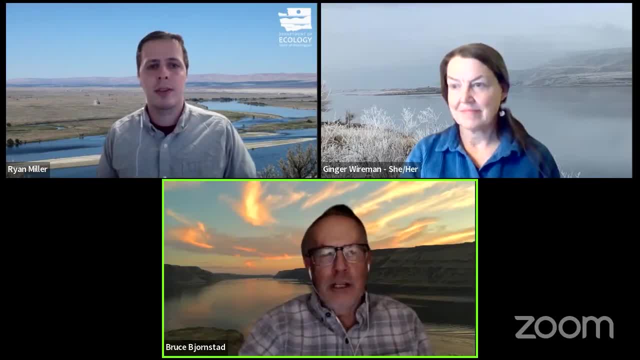 Bruce D Potter, Those are actually. well, some of them are on hand for site, some of them are fishing wildlife land which is generally inaccessible to the public. Bruce D Potter, You can actually, if you have them, but if you have a motorboat you can. you could go up the Columbia river and actually access those sand dunes. 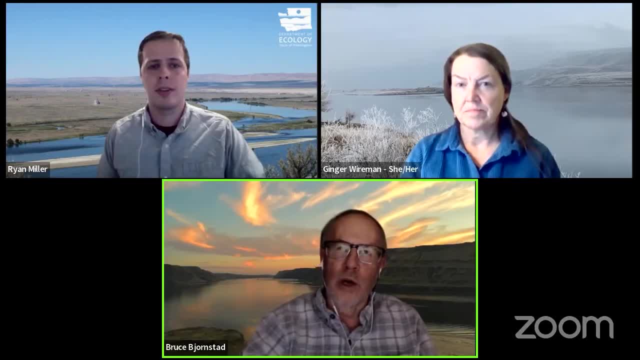 Bruce D Potter, That are in the national US fish and wildlife land but the best place to see sand dunes and public land is up near the white blouse very landing, which is up north along the Columbia river and you can drive there some fish and wildlife land publicly. 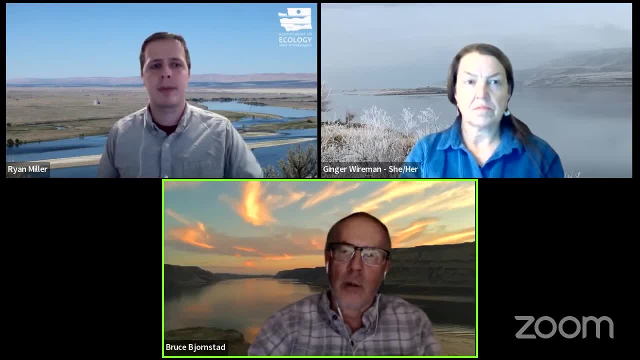 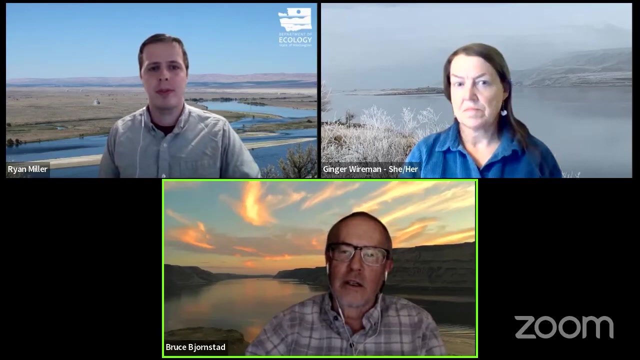 Bruce D Potter, You can actually hike to some beautiful sand dunes that are up high along the river and I showed them those those big, long sand dunes over in my video- Bruce D Potter, Along the river. you would those are. those are open to the public and I highly recommend going out there. I I love going up there and just hiking. you can hike for miles up there and hardly see anybody and have the place to yourself. so if you want to see sand dunes, i'd i'd recommend going up to 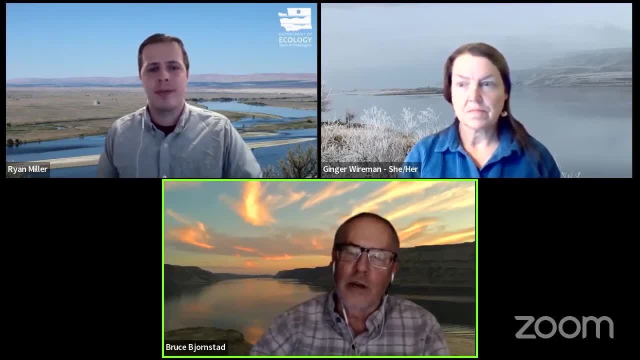 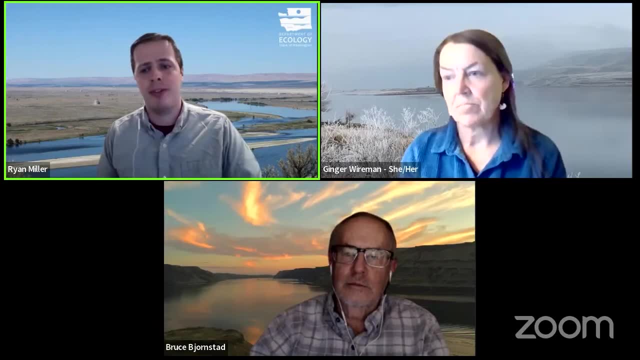 Bruce D Potter By the white blouse, very landing, and taking the trail that leaves from there. Chris Winslow, awesome Thank you for your question. also say ginger shared a link in the chat that that shares the white blouse- very landing. i'll go ahead and put that link into the Facebook chat and go and ask your question. 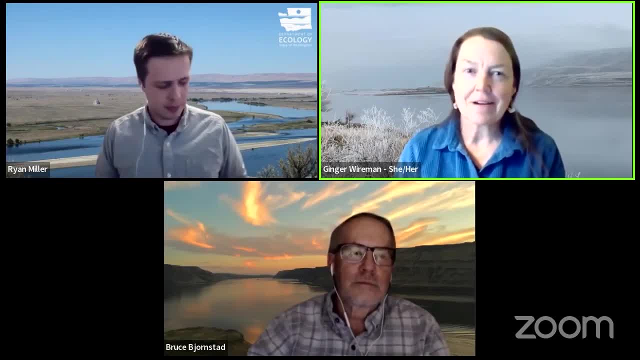 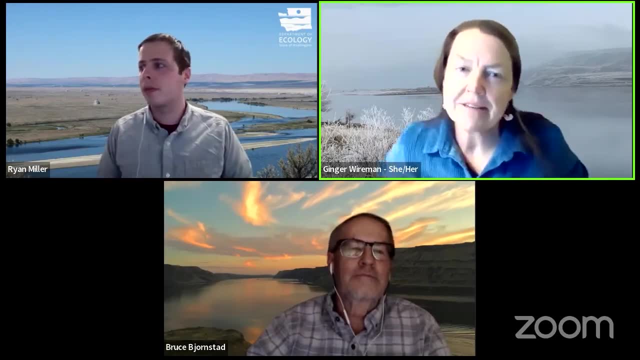 Ginger Kowalczak. And just a warning. I went out there a couple of weeks ago and if you try to go right now, it is extremely muddy at the top and the mud is, Ginger Kowalczak, You say clay and it's.